may connect and network with each other. This can be done by using the chemical engineering life. You 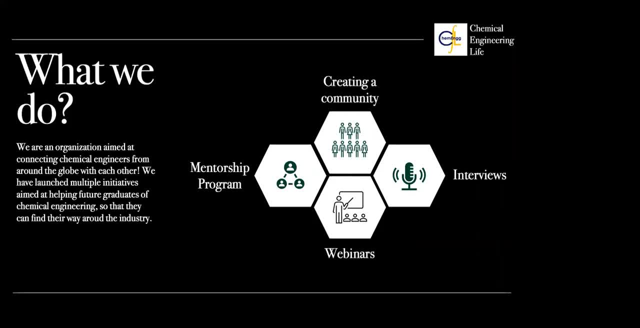 can become a part of the community by becoming a free member on our website. We also share interviews of chemical engineers from around the globe, where they dive into and tell us what they do and how they do it. This acts as inspiration for the readers and shows how many different fields within the field of chemical engineering exist. We also run a mentorship program. This is a biannual program where we connect young professionals to more and more experienced engineers from around the globe. Like we are doing today, we host webinars. Our webinars are done on different topics. These are done by people who have a lot of experience within the topic that they showcase to us in our webinars. All the people who host the webinars are the one who, let's say, they know what they're talking about. It's no joke. 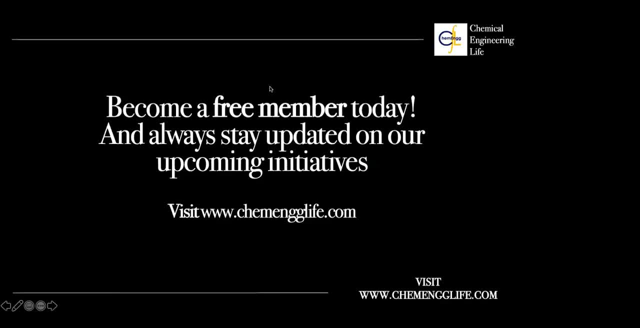 Make sure to become a member on our website. To become a member it is completely free. 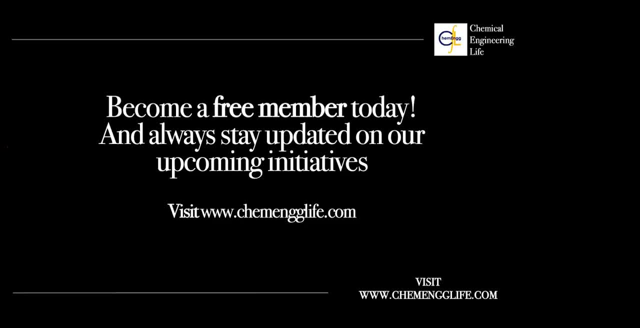 Honestly, why not do it? By becoming a member, you get a head start invitations to all our different initiatives. So you don't miss out on anything, whether that is our webinars, the mentorship program, the interviews, everything. That is it for what we do at chemical engineering life. 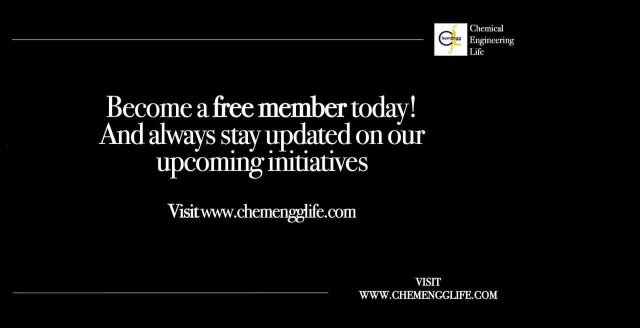 Now we will move on to the next slide. Thank you for watching. The link is in the description. If you want to check out our next slide, please do so, click the link. If you have any suggestions related to engineering, please contact us via the chat box at GMS. . And if you don't want to miss the next slide, the link is in the description. Or contact us via the chat box on the screen. We will send you an email once. You can check at that link and we will be able to get to the next slide. I will pass on the mic to Hamza and Kaz Fula because I'm sure you are all very eager to learn 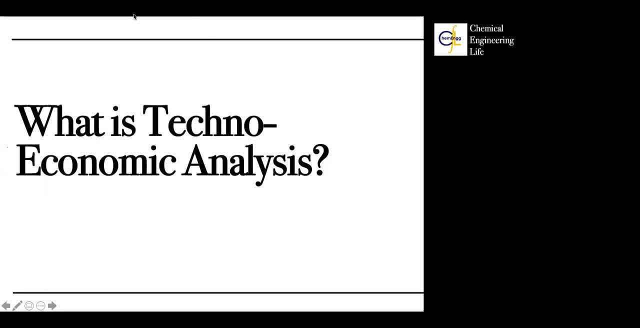 about the economic technical analysis. So let's do it. Welcome, Hamza. The mic's all yours. 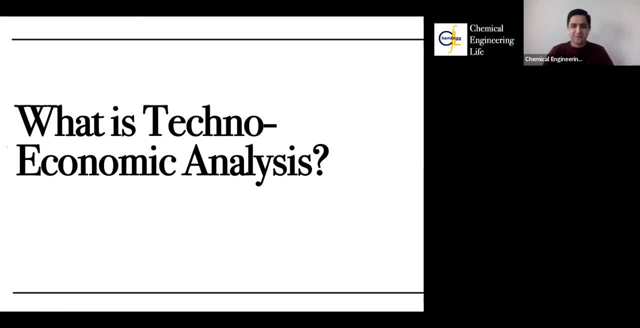 Great. Thank you so very much, Emma. Thank you for the great introduction. And hello. Good morning. Good evening, everyone. Thank you for joining us today for the webinar and for willing to listen to me speak about technical economic analysis. So to begin with, let's talk about what exactly 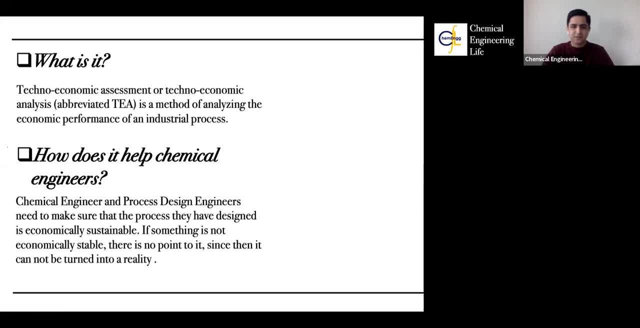 is technical economic analysis. And technical economic analysis is defined as a method of analyzing about the economic performance of an industrial process, basically just asking yourself the process that you are designing as a chemical engineer, will it or will it not make any money? And that is much more important than many people perceive it to be because in reality, every process or every project that you work in as a chemical engineer or any engineer, 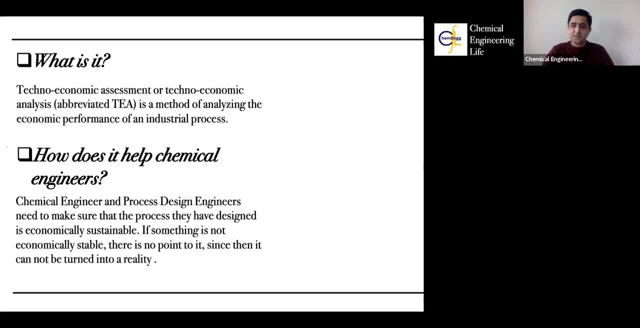 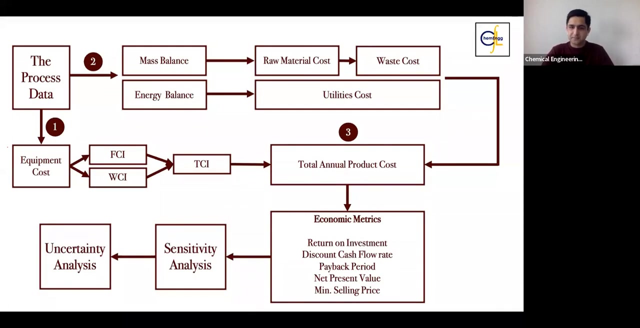 at the end of the day, it all comes down to dollars and pennies. If the process that you have designed, if it is not making or generating any profit, then that project will never be implemented or actually go into production. Therefore, when you are designing a process, you need to be able to keep in mind that the process that you are designing always is profitable, is capable of making money, and the money that you will generate from your production can be used to further expand or to sustain your own expenses within the production. And that is something that we'll do today. The general process of doing techno-economic analysis is that you start off your process data. The very first step is that you, for all the design that you have created, that you have designed, that you have made, you need to find the equipment cost. The equipment cost is something we call the total install cost. That means that you need to find the equipment cost, the equipment cost is something that you, for example, when you have a heat exchanger, it costs a certain amount. Then you also need to find, then you also need to calculate how much will it cost when it is installed in your production site. And that is what we call the total install cost. You do that for all of your equipment. You find the sum of all of them. Using your equipment cost, we can then go in and find 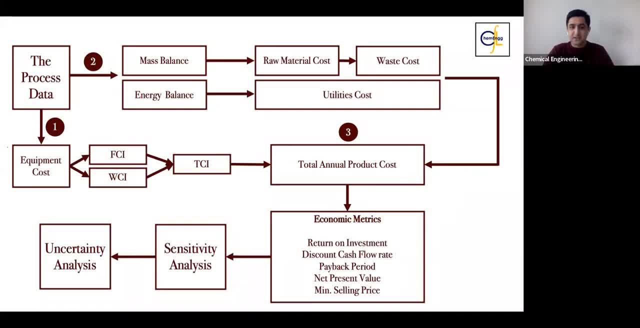 our capital investment. The capital investment is the money that you need in hand to basically build your plant, or the money that you need to build your plant. And that is the total investment that you need to raise to start your business. By doing so, then the second step then is that you need to perform your mass balance, the energy balance. Through the mass balance, we then find our raw material requirements, product production, the waste production. And then, of course, you need to buy your raw materials, you need to sell your products, and you need to pay for your waste that is being produced. Using the energy balance, we can then calculate our utilities cost. And the utilities, they include everything from, you know, the energy cost, the source of the waste that is being produced. So, we can calculate the cost of the waste from steam, cooling water, electricity, refrigerant, and anything else that you might need for running of your plant. And once you have done that, and you have your capital investment, and you have your day-to-day operation cost, we can then go ahead and calculate something we call a total annual product cost, or also referred to as PPC. This is the amount of money, the minimum amount of money that you need to run your plant. And that is the amount of money that you need to run your plant. And that is the amount of money that you need to run your plant. And that is the amount of 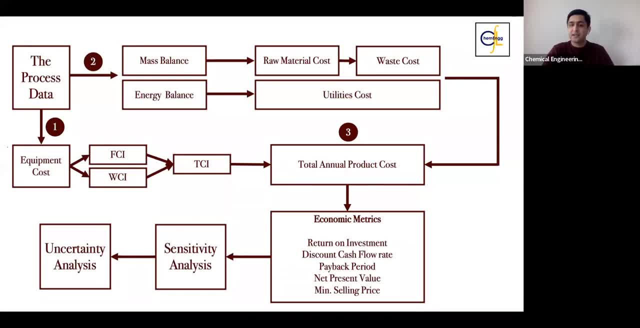 annually. So that means that if we calculate that you need $10 million per year, that means that you need to have $10 million in hand by profits or by investment or by any other means to make sure that your plant keeps running. Once we have this value, then keep on using all the other variables, we can then move on and calculate our economic metrics. There are multiple metrics that we can use to calculate the profitability of a plant. But for the purpose of this seminar, we're actually going to focus on return on investment, payback period, net present value, and the minimum selling price. And we'll dig a little deeper into what exactly they are and what they mean. Once you have the metrics in place, and this part is very important because everything that you do up until this point, it all is very theoretical. We are not actually building a plant. 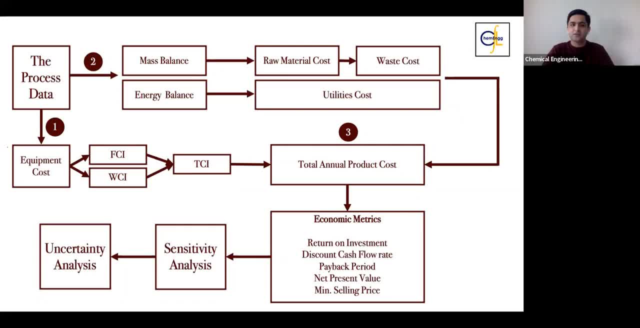 You're not going to be calling actual suppliers and asking them the cost or the realistic cost of each and every equipment. 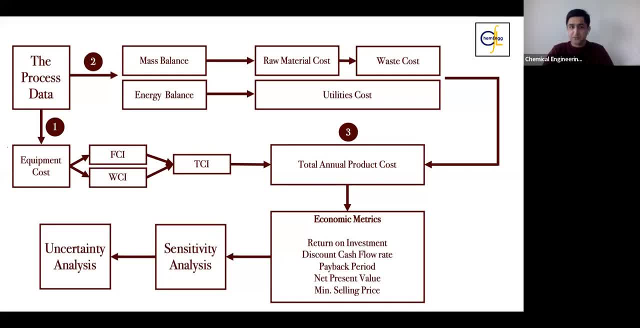 But all of this is done through literature study. So when you are doing mass balances or energy balances, the price of your raw materials, your products, the cost of how much electricity costs, these all will have to be taken from literature. And therefore, it is very important for you to understand that all the calculations that you do, you need to be able to verify and validate those numbers. One way of doing that is, of course, 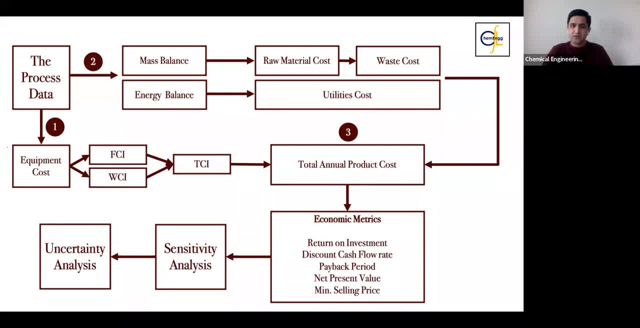 you can do sensitivity analysis. Now, the sensitivity analysis does not really cover the validation or the verification part, but it covers the uncertainty that you might have in any of these numbers. One example is, for example, if I was looking at a raw material cost, let's say I'm buying methanol. If you were to take the price of today, but the price of methanol is dependent on the market, so it can either go up or it can either go down. Tomorrow, it can increase by 10%. It can increase by 10%. It can increase by 10%. It can also decrease by 20%. It can also decrease by almost 50%. That is something that is entirely dependent on the market. These sort of deviations, that is something we cover through sensitivity 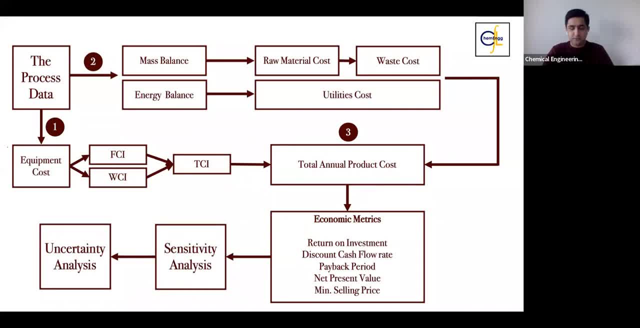 analysis. And again, this is something that we will dig deeper into this webinar today. And finally, you can also do uncertainty analysis. We have decided not to cover the uncertainty analysis in this webinar, but the uncertainty analysis covers how certain or uncertain your values that you have used are using different products. So, for example, if you have a product 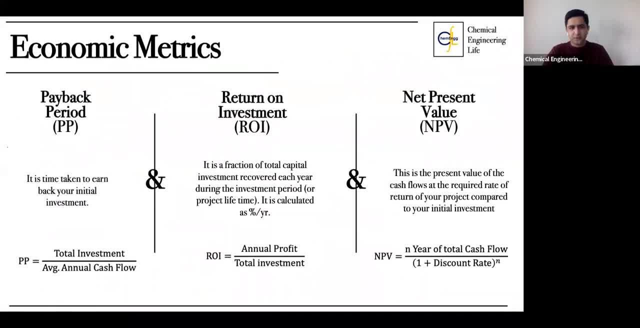 So, coming up to the economic metrics, and it is very important that we understand what these metrics actually mean and what it is that they are covering. So, firstly, the metric that we have decided to look at is the payback period. So, when you get an investment for your project or for your production, the payback period tells you how long will it take for you, to fully cover those expenses let's say you're buying a shop and you go to the bank and the bank gives you a hundred dollars and you need the payback period tells us how much time will it take for us to pay back that loan 100 to the bank and that is calculated as so you have your total investment divided by your average annual cash flow so how much money you make in a year for your investment divided by your annual cash flow per annum and that's where you end up getting the years how long will it take for you to give back the money the shorter it is the better 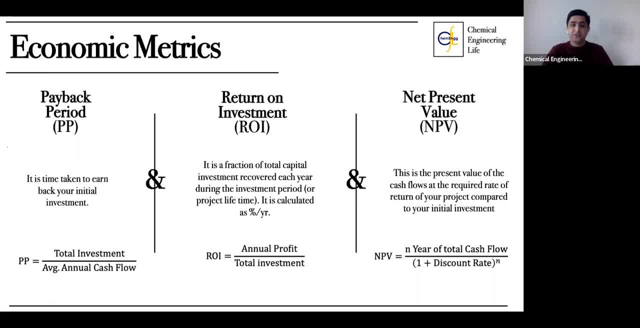 the longer it is the worse it is because if it takes you 20 years to pay back your capital investment that means that you're not making that much money to cover up your expenses and then for your investment and your investor might ask you that if they're going to see all the money in 20 years years, then they are better off investing in someone that will be able to pay them back in one year. 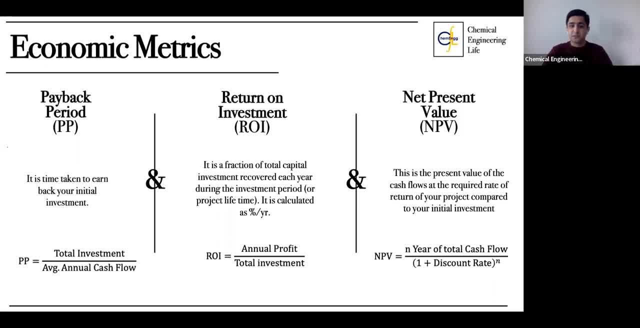 The second metric that we decided to look at is the return on investment. 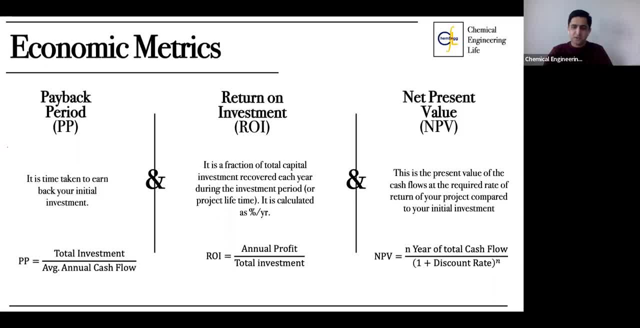 And it tells you it is a fraction of total capital investment covered each year during the investment period or the total project time. 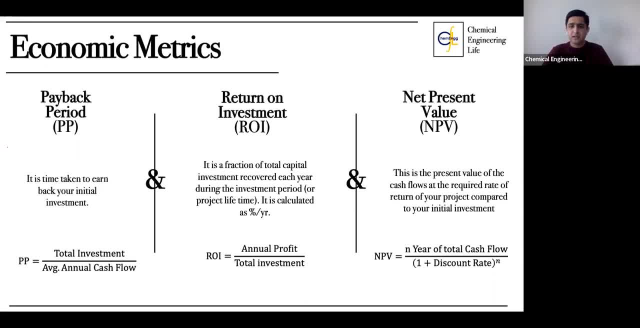 So let's say we have a production for 20 years and you need to be able to understand or you need to be able to tell you an investor about how much money did you actually end up making with respect to your investment. 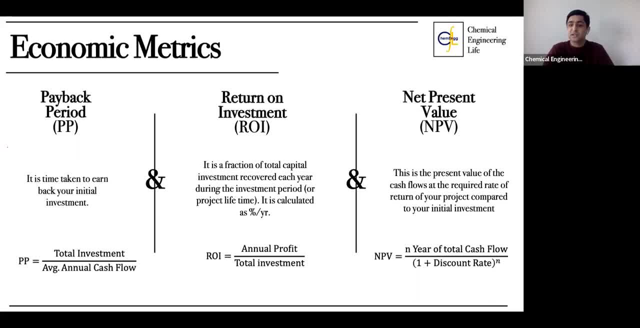 And of course, it should always be more than one, like more than 100%. So you have your way we calculated is your it is your annual profit divided by total investment. And this part is very important. 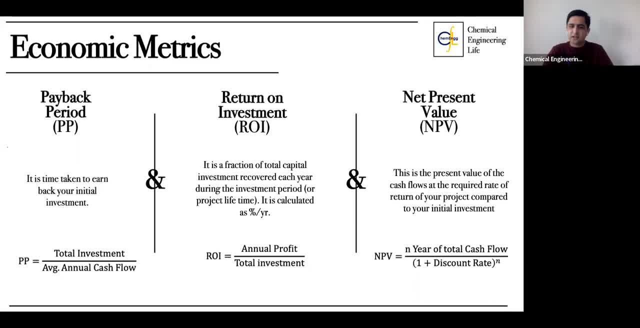 As you can see, it is your profit that you need to calculate and not your annual cash flow. 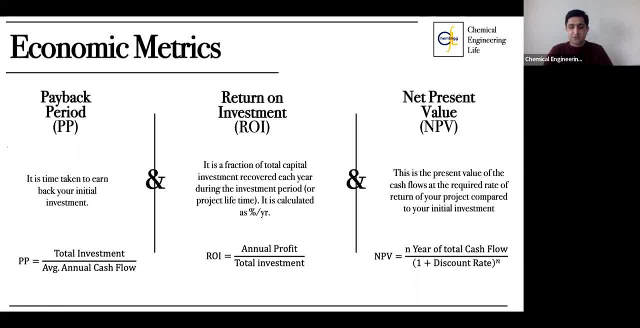 So let's say I'm selling something for, let's say I have a shop and I'm selling something and my annual income is $100, right? But that $100 is not my profit. I need to pay taxes. I need to pay salaries. I need to pay my expenses. And let's say my profit comes down to $20, right? 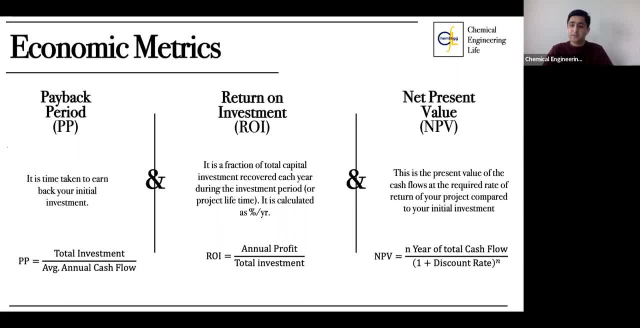 That $20 and divided by your total investment. And let's say the. 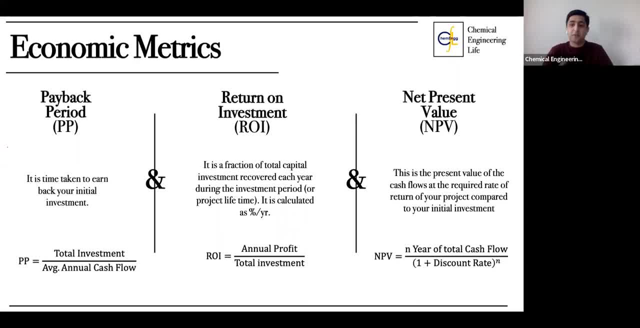 Person gave invested $10 in my shop, but my profit is $20, but that will be 20 over 10. That means that my profit is still my ROI is still 100 double what my investment was. 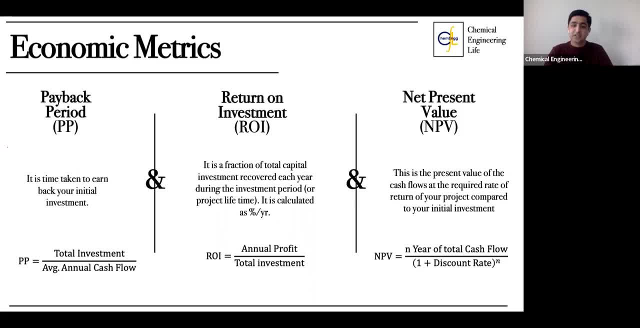 And this is very important because many people, they end up using the actual cash flow. It's not, it is your annual profit that you're going to be using. 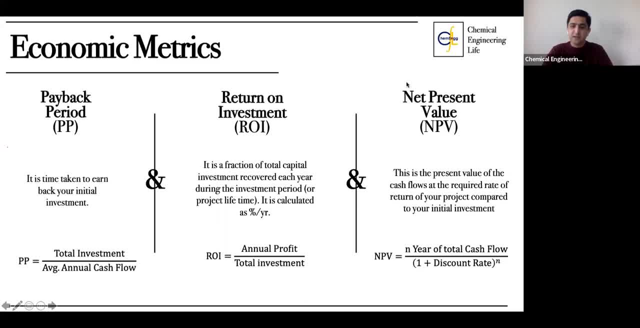 Finally, the behalf is the net present value, the net present value, it relates how much money, uh, how much money you're in your investment will be worth in coming years. Let's say you have 20 years. It calculates how long it calculates the time value of your, of your investment and the time value in order to understand is that, um, you all have to understand that with time, the value of money changes, the money that you have today is going to be worth a lot more than the money that you're going to have. In a year from today. 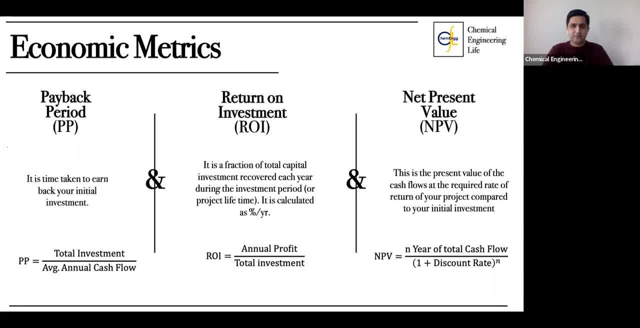 And the reason is that today you can buy, let's say you have $10 today. You can buy more stuff with it because it has more buying power, but in one year time, due to inflation, due to some other variables, do the market fluctuations, if you're going to have $10 in one year time, that's not a good net. That's not going to be as powerful as a $10 you had today. So with time, you actually end up losing value unless, unless you invested your money in a bank or. Or you, and you took interest on it, or you made a business with the money that you had today. 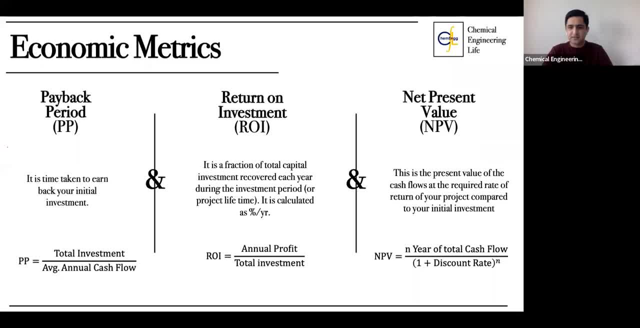 And the NPV, the net present value is something that calculates how worth your money will be in the coming years. 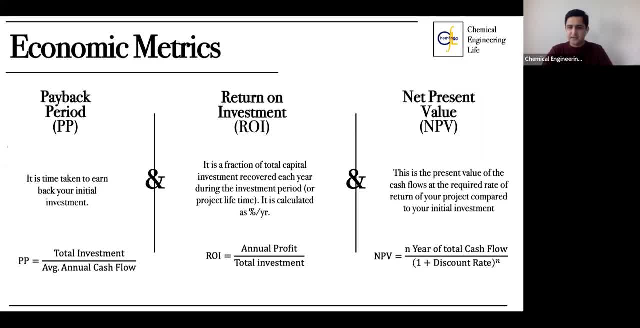 And the way we calculate it is you, it is the, uh, the end, it is the number of years for the end year of total cashflow, but you sum up all the money that you have earned so far, you divide it by one, by something we call it net present. 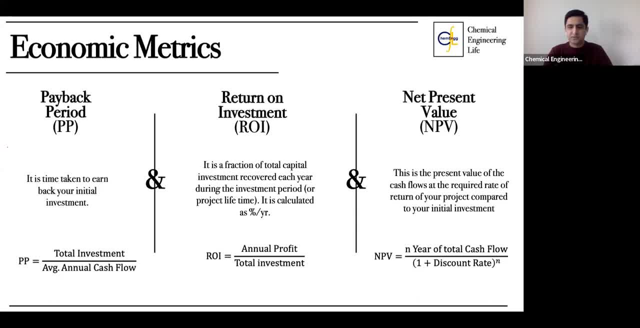 So the net present value is the worth factor, and it is calculated as one plus discount rate to the power of n, where n is again, the number of years, the discount rate is, is the rate that is given to 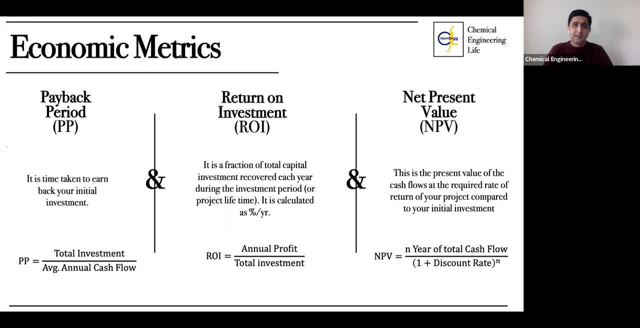 you, depending on how risky your investment is. Now you must be like the, the less risk there is, the lower the value will be, the more the risk there is, the higher the value will be now for the purpose of this webinar, as I'll tell you later on, we, we have decided to use. 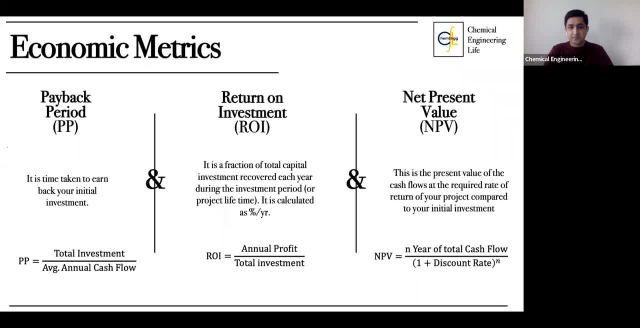 The discount rate. Uh, and now you're going to be wondering that what makes something less risky and more risky in a chemical process environment. 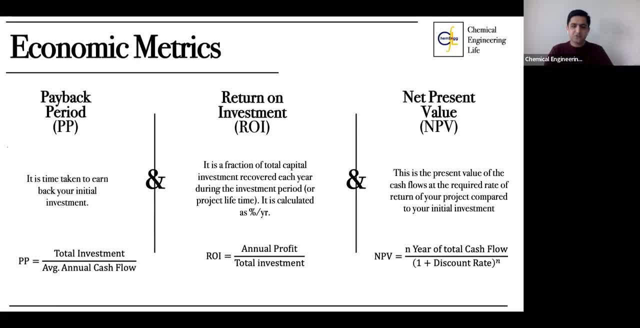 And, uh, the easiest way to do it is that if something is developed, if something has a very good market, if something has, if it is something that has been done before you, it's going to be very low risk for the bank, for your investment. 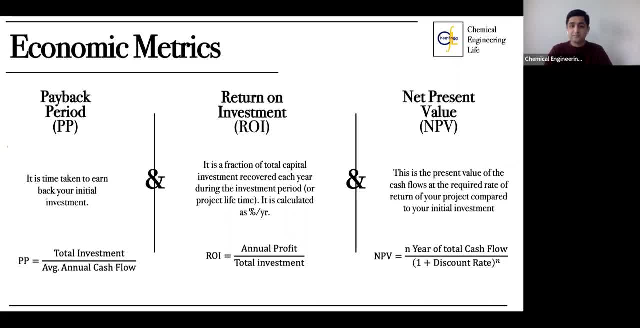 So let's say if you want to go and build a plant to produce methanol, that's very low risk investment. Why? Because it has a created zero market. 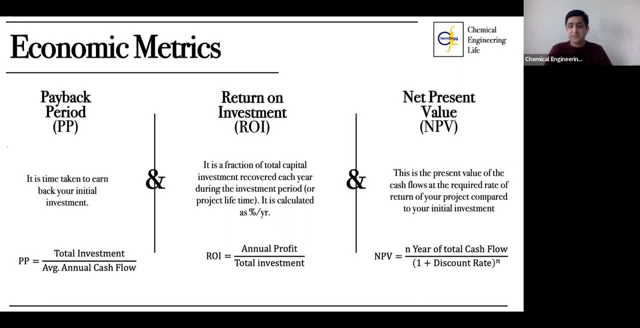 It has a great deal of, uh, for example, many other companies have done it before you, and they all have been quite successful at it. 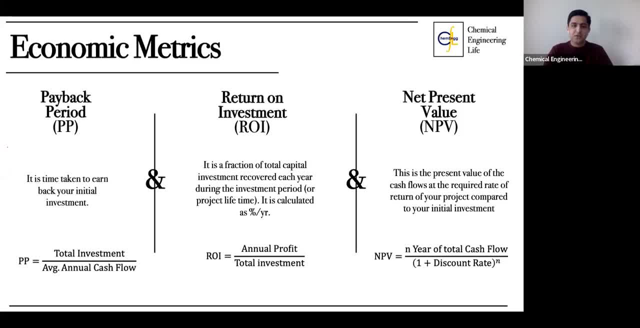 So the investor are going to be able to do it, but let's say you go in and you tell someone that you want to produce a biodiesel, for example, now the biodiesel does not enjoy that huge of a market as methanol though, biodiesel is not something that is readily available. There are not a lot of companies out there that are working with it. 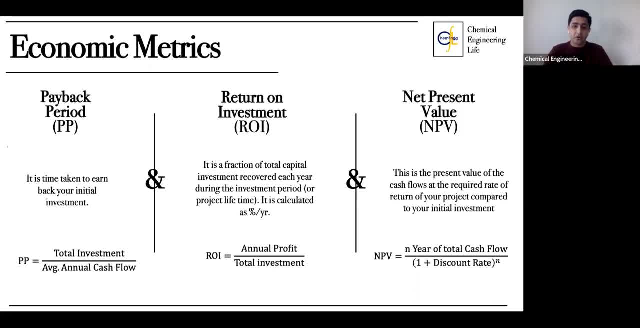 So now the discount rate would actually be slightly higher. Uh, and like I said, for, since we're going to be looking at biodiesel production for this webinar, I have selected the value of 11%. And these values, you pick them from literature. 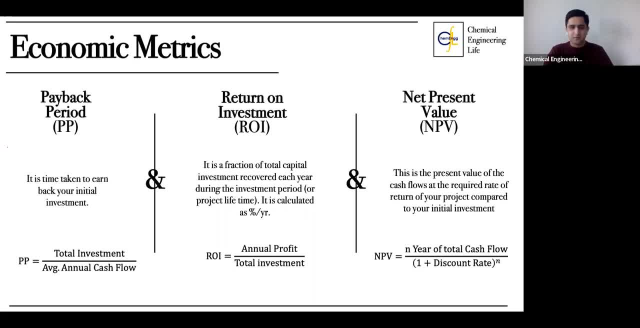 There are different factors that you can use to calculate. Uh, there are different, um, like for example, if you were to look at different intervals, the lower the risk it is, you can, it takes a value between zero and one to five. 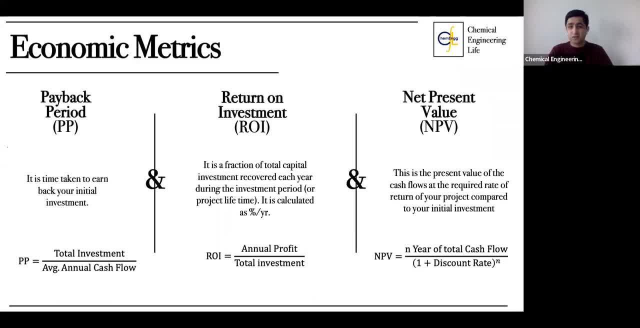 If it is medium risk, you can take a value between six to 12, if it is very high risk and it can go up to 15%. 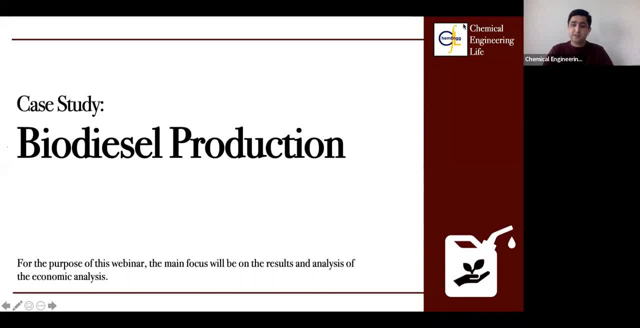 Then that, that would be the brief that, that was the all for a brief introduction about technical economic analysis. Now we'll dig deeper into the applying technical economic analysis to a case study. 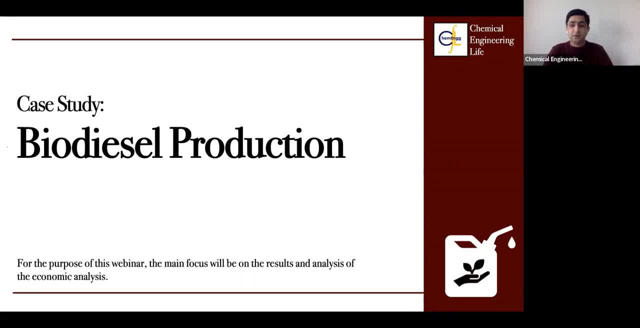 And now for the purpose of this webinar, I have decided to work on a biodiesel production and, um, the data or the methodology that is being presented here is slightly inspired from the, my own research paper title and integrated biorefineries, uh, that, that, that has been shared with all of you before the webinar. 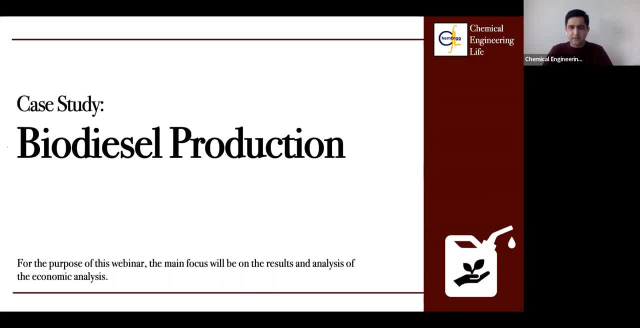 I hope you all had a chance to look through it, but if not, we're going to go through key values, um, in the webinar as well. 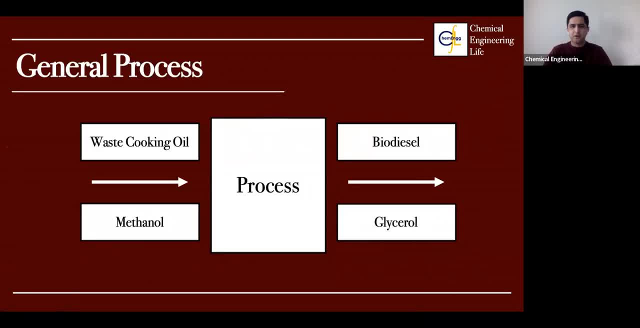 So the general process for the boundaries of production is that you're going to be using waste cooking oil and methanol. Uh, we use that in a, in a catalyst process, and then we create biodiesel and glycerol. Now, uh, we do, we are using waste cooking. Oil and the methanol and the waste cooking oil is actually a waste product. So already there, uh, the, the, the idea behind using the waste cooking oil is that it is cheap. It's easy to find. It's cheap. It's, it's a waste stream. 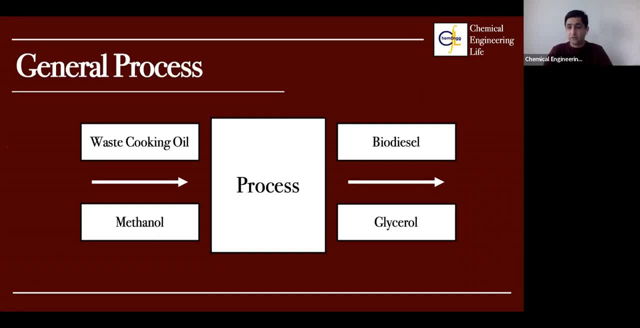 It's not a valuable product, so it can be acquired at a very low price. Methanol, unless one of the products that is the requirement of the process, and then we produce biodiesel and glycerol. 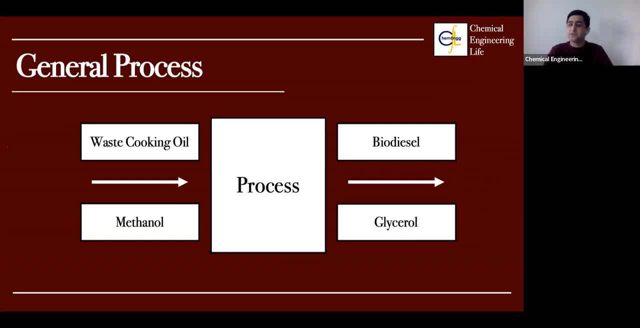 And now the, the purpose of, of biodiesel production, of course, is that we are moving. 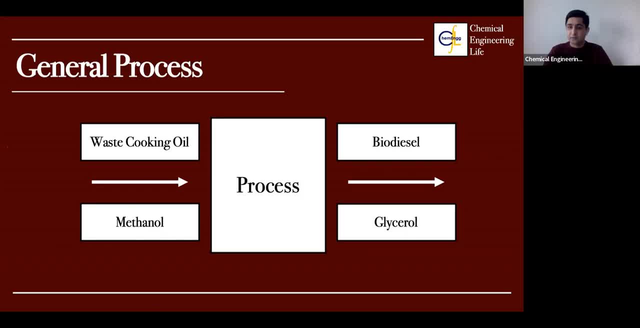 We are moving towards, uh, we are facing many climate challenges around us, and instead of using petroleum fuel, biodiesel can act as a very good alternative to petroleum fuel. So in that way, you can see that, uh, the process that you're using for the production of biodiesel is, can be in, in high demand. 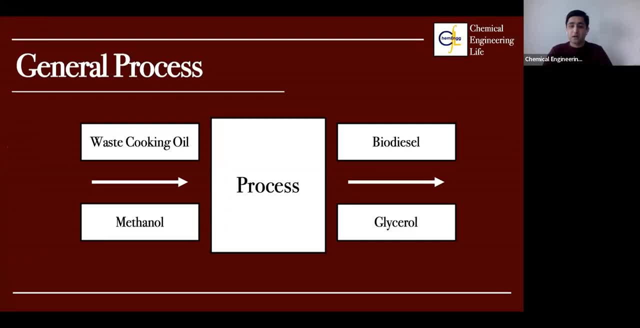 It can, it is very useful. It is a major requirement for our, uh, global, for fighting up the challenges of climate change, and therefore. 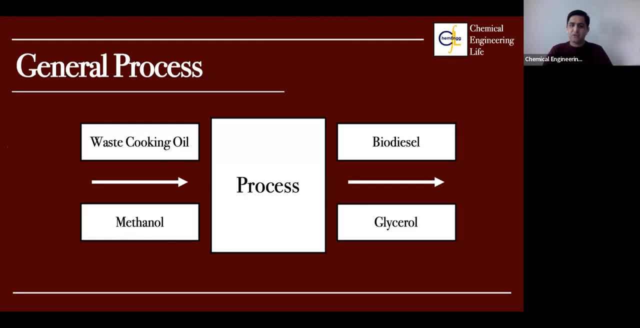 It can be argued that it is not a very high risk investment, but it is at a somewhat medium level investment, because even though it does not have a strong market right now, but as you're moving, but as we're going into the future, it might create a bigger market. 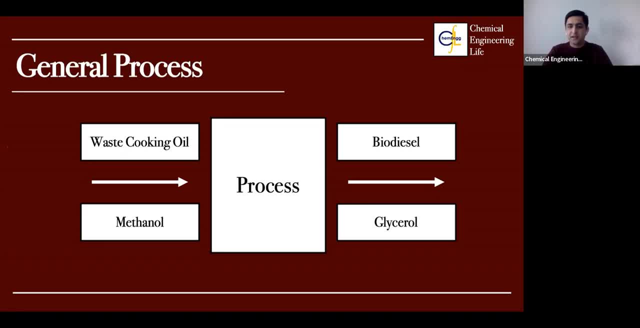 So therefore it, therefore we have, like I said earlier, that we have used the discount rate of 11%. 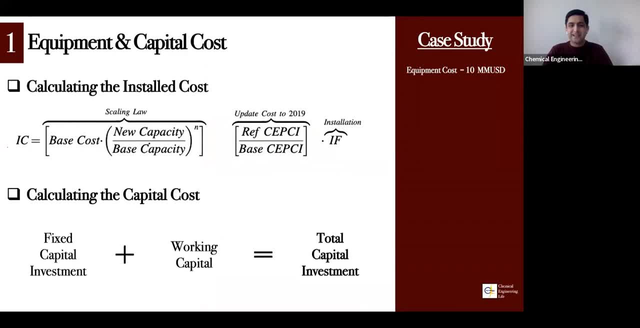 So the very first thing that we need to look at that is the equipment and the capital cost. The equipment cost can be calculated using the formula, uh, that is shown on the slide. Uh, now there's one thing I don't want you all to confuse that these are two different terms. So when you say equipment cost, that is the cost of your equipment, but then we have something called installed cost, and that is the cost of your equipment that is installed into your facility. So let's say I want to buy a flash tank and a flash tank. Cost, let's say $20. That is the equipment cost. What we want to calculate is the total installed cost, and that means that we need to calculate the cost when that flash tank is also installed within our facility. 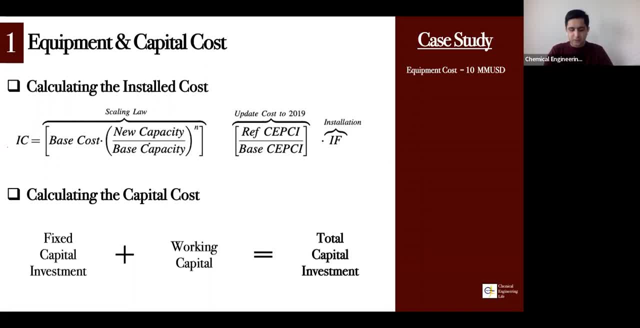 So the first thing that you need that you need to do is that you have your requirements. So you, um, design your equipment, you calculate the capacity, uh, the capacity capacity is not the correct word, but it's. 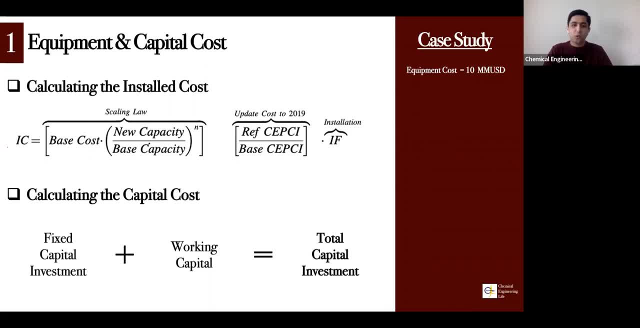 Usually the, uh, the variable that you're going to use, for example, when you're working with a flash tank, you use your cubic cubic, uh, metrics with the volume when you're using the heat exchanger, you use area, uh, so therefore for, uh, flash tank, it would be your volumetric capacity. 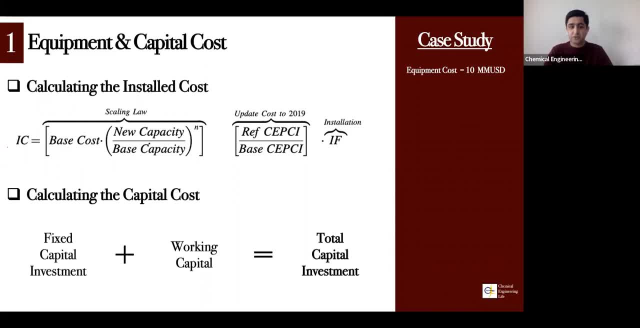 Then what you deal with, you go in and you, you scout, you scouts to literature. And you find the cost of, uh, for a given you, you find the cost for a given capacity within a book or within a literature study. 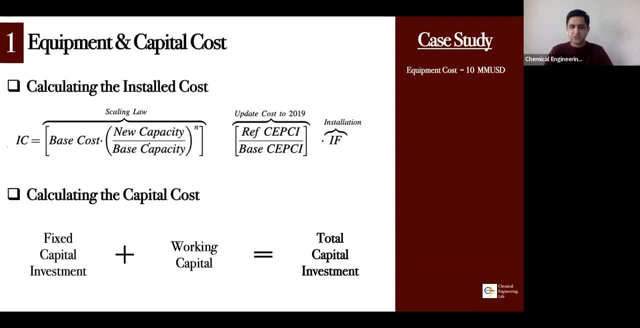 So that means that you go to, you find a paper and many of the times it's good to you always use validated papers, uh, papers that have been written by maybe the government or different universities. And so, and let's say you find from a paper that, uh, 10 cubic meters capacity of a flash tank costs $5. 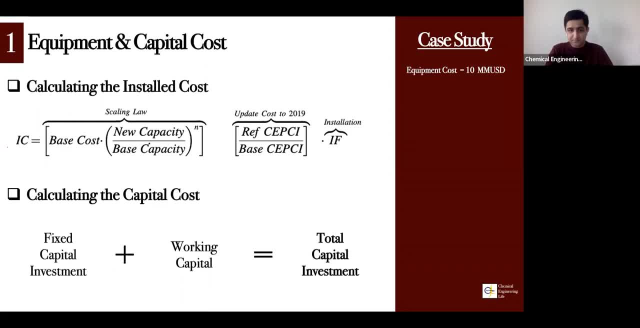 Then that's an example, then you put that into that formula and the end value that is, uh, that is the, uh, that is also the scaling factor and that it can post that is to be found from literature as well. 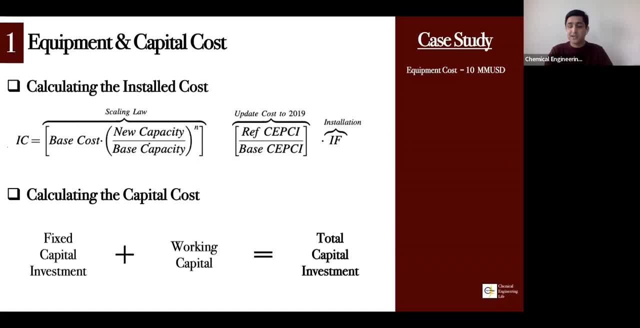 It is different for each equipment. So you can't just use, uh, the same value for all of them, but it's different from flash tank to distillation columns, to, uh, heat exchangers and so on by using that first equation, and you are, what you're doing is that you are finding the cost. 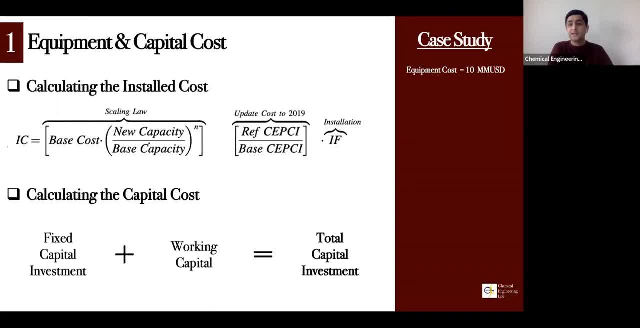 Uh, Uh, Uh, Uh, Uh, Uh, Uh, From the base cost to the capacity that you need for your equipment, and that is something we call the scaling law. 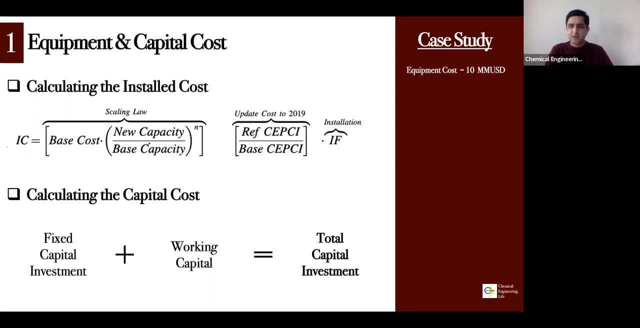 Uh, once you have that price, so that means that for your 50 cubic meter flash tank, it's going to cost you, let's say, this amount of money, then that is not necessarily for the year that you're working in right now. So let's say we are doing an analysis in 2022, and the price that you found was from. 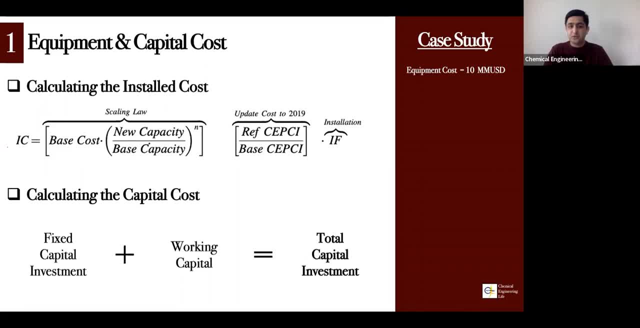 2005 Let's say, uh, 12. 2005 It is always best to find the prices within the last 10 years because then there are the newest prices. 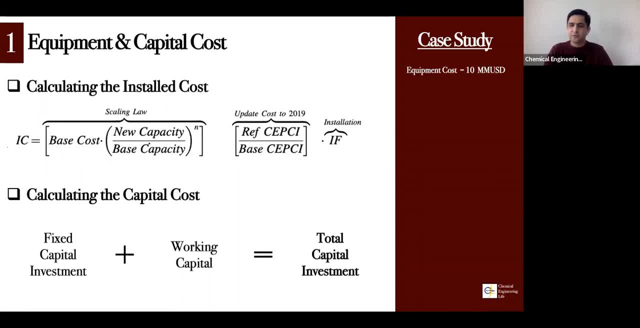 It's not a good idea to go back and find a price from 1940 and then convert that to now because that's a great deal of error and uncertainty. So it's always a good idea to use the prices within the last 10 years. 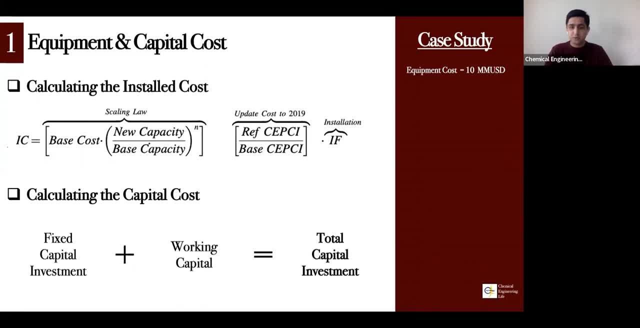 And the way you then, of course, you need to convert it to your present year. The way you do it is that we use this, uh, No. 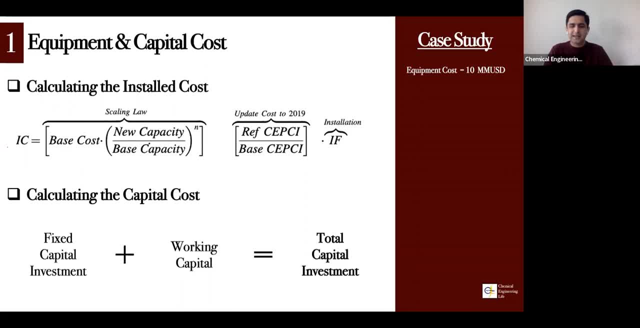 number called CEPCI, which stands for Chemical Engineering Plant Cost Index. Every year has a special value. So you find the value. So let's say we found the price from 2005, and you take the value from 2005, and you find the value for the year that you were doing the analysis for, and then you convert that year's price to your current year. So now what we have done so far is that we found the price for our capacity, then we converted that price to your current year, and then finally, like I said in the very beginning, you need to find the cost once the equipment has been installed. Then we multiply that gold price with our installation factor. 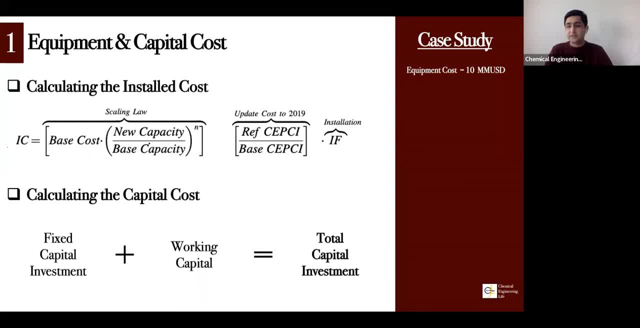 The installation factor itself is very different for each equipment, and that can also depend from literature. For the purpose of this presentation, I'm going to show you how to find the cost of the equipment. So let's 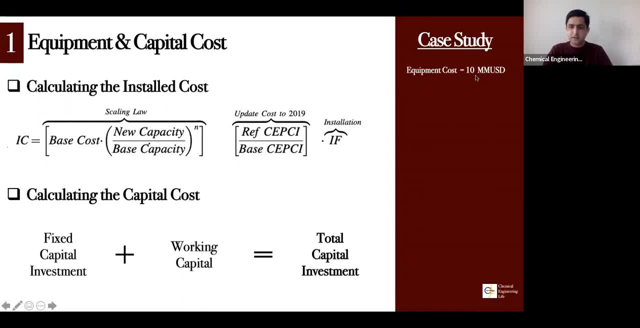 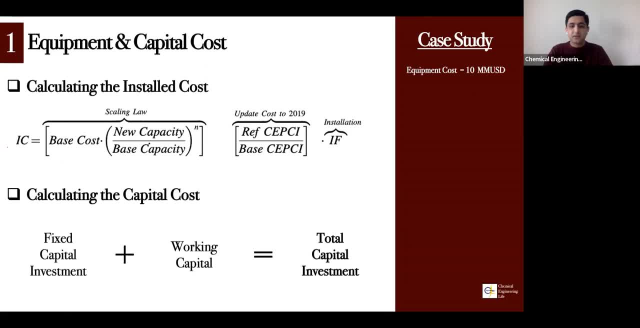 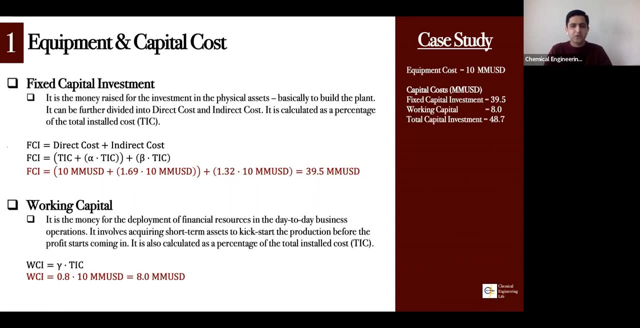 and you have your total install cost, you can then go on and calculate your total capital investment. The total capital investment is the sum of your fixed capital investment, FCI, and your working capital. And the fixed capital investment is the investment that you need to basically build your 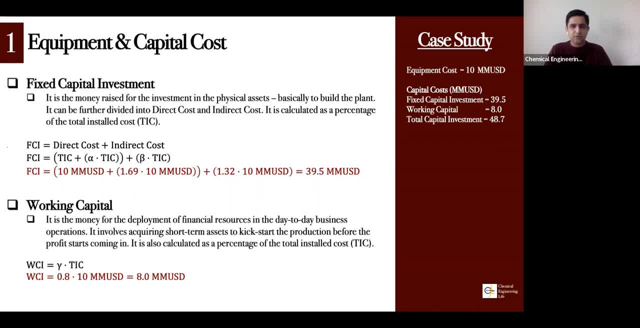 plant. That is all the money that you need to build your plant. So let's start with the cost of the equipment. So let's start with the cost of the equipment. So let's start with the cost of the equipment. So that is the cost of the equipment. So let's start with the cost of the equipment. So let's start with the cost of the equipment. So that is all the money that you need to something that you need to build a proper functioning facility. 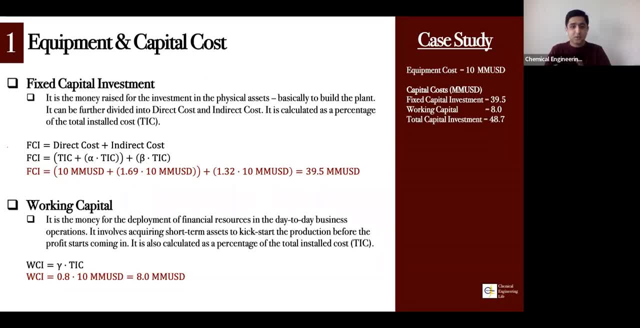 All that, that you need to prepare, to create a physical asset or to create a physical building, that comes under fixed capital investments. And its based on the intention that the insurance generator provides you with everything. In fact, it's based entirely marry things that are 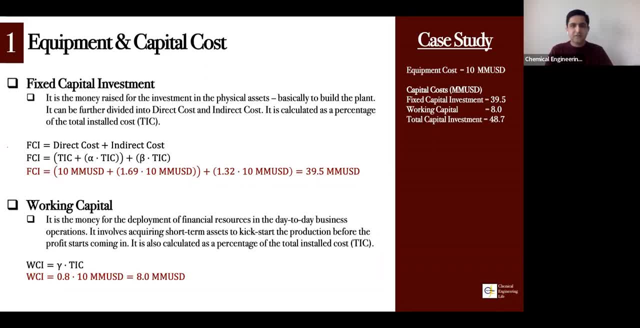 decompressed as a matter of fact. For the reasons that I mentioned at the beginning, everything from cars to archives to the fuel lines, it shows that you have to produce these electrical components in a way that are at youršmixable-üzikpad at the right time to 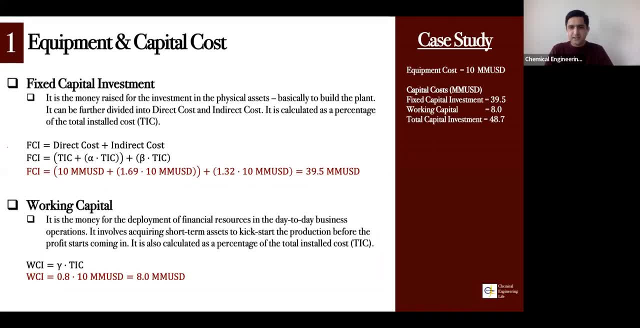 comes under fixed capital investment. To make things slightly easier, the fixed capital investment has been divided into, it's further divided into subcategories 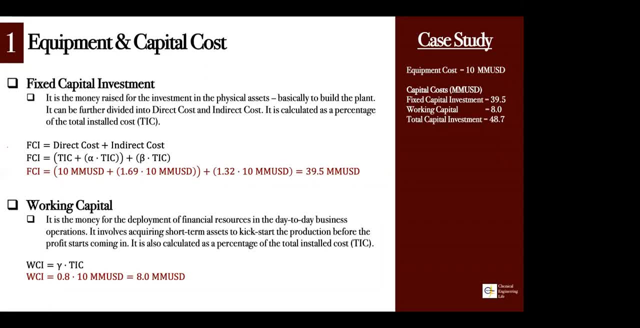 for your direct cost and indirect cost. 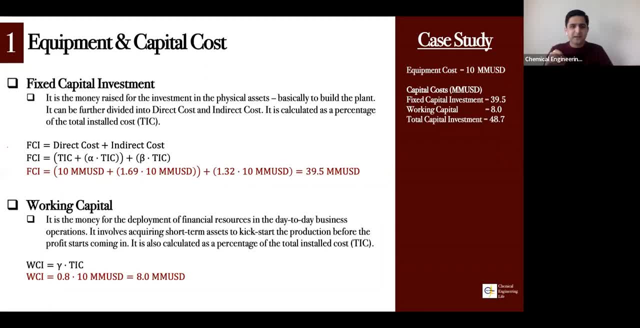 The direct cost is something that you need that is the money that goes directly in your production facility. 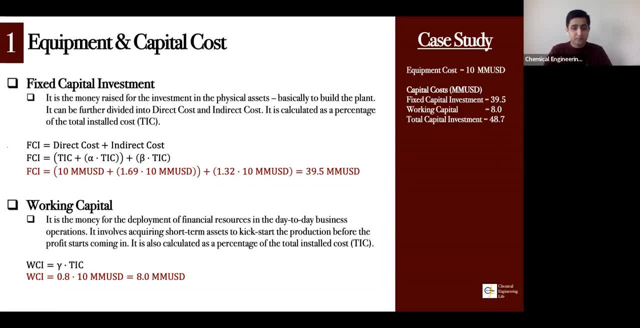 Direct cost, that means it includes everything from equipment, transportation of equipment, installation of equipment, piping, instrumentation, maintenance, paint, everything that you are doing within your production facility, that money needs to be taken from your direct cost. 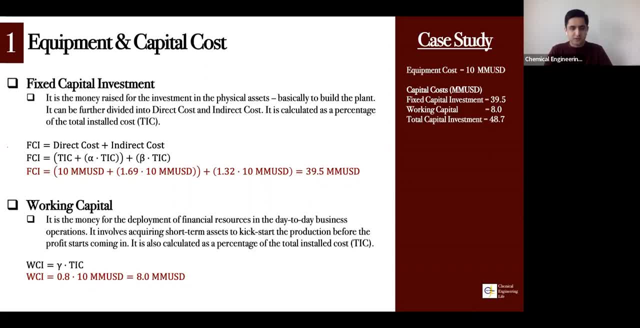 Then we have something called an indirect cost. The indirect cost is all the money that is required for the production, but it's not actually being used within the physical assets. For example, it could be anything in legal fees. It could be your contractor fees. It could be you need security. All the administration duties or administration costs of making sure that your plants get built, that needs to be covered by your indirect cost. 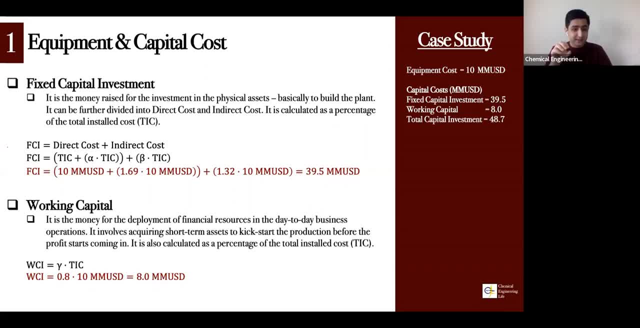 And your direct cost is something that covers the literal building of your facility. 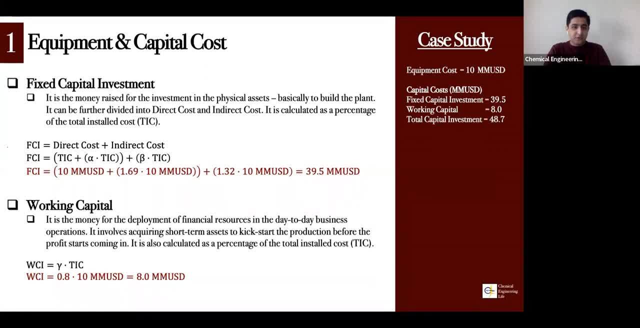 Now, your direct cost should, of course, always be higher than your indirect cost. 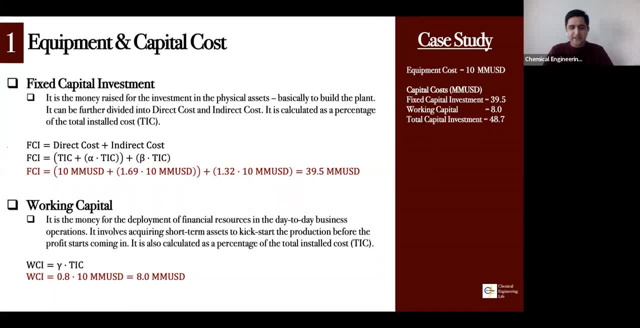 And I'll get into it in a minute on why it is. The way we calculate the direct cost and indirect cost is that we use our total installed cost of our equipment as a base value. And you multiply a factor with that equipment cost. 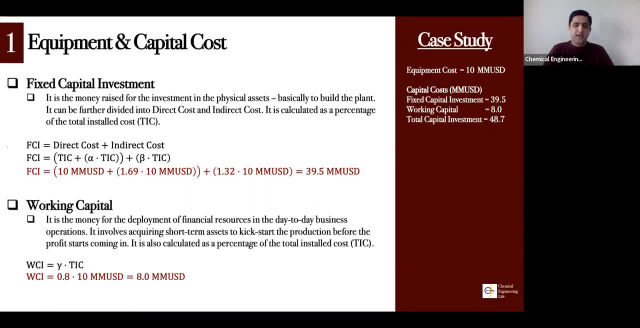 That should give you your direct cost and that should give you your indirect cost. 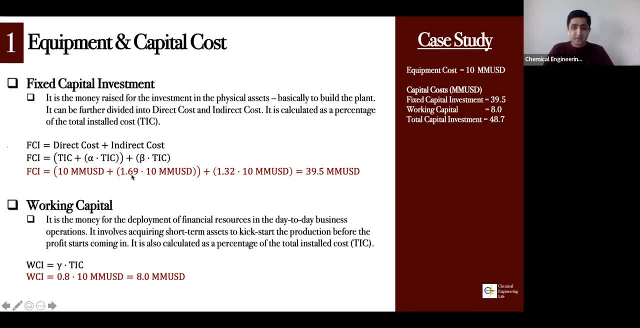 For the purpose of this webinar, I selected 1.69 as a factor for my direct cost and 1.32 for my indirect cost. And I'll get into it in a minute on why it is. 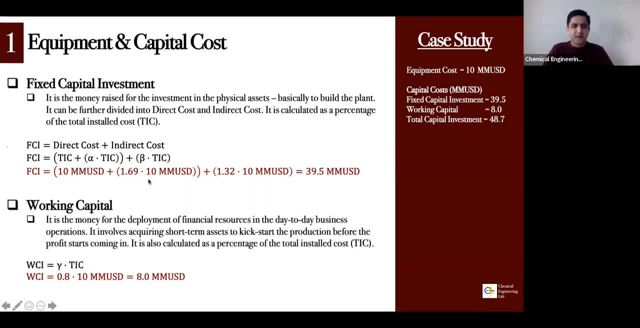 What it means is that that means that my direct cost is 1.69 of 10 million. And my indirect cost is 1.32 times by 10 million. 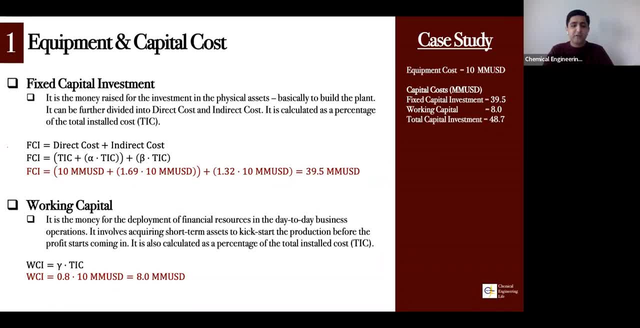 And that then gives me my cost. But you have to be very careful here because, like I said, for the direct cost covers all the assets. So you need to add your equipment cost, which is my 10 million, plus the factor times by 10 million. So that means that my direct cost is not just 1.69. It's actually 1.69 times by 10 plus 10 million. So you have your equipment cost. You calculate the direct cost. You multiply the factor. 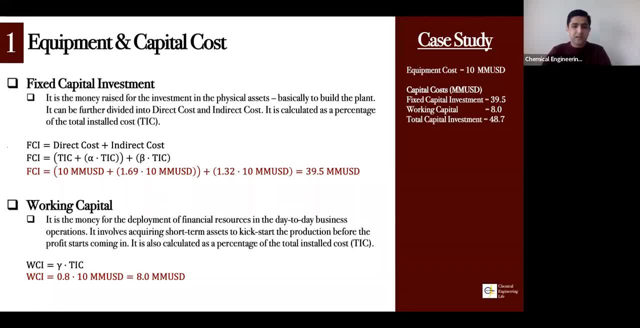 So your direct cost is the sum of those two values. 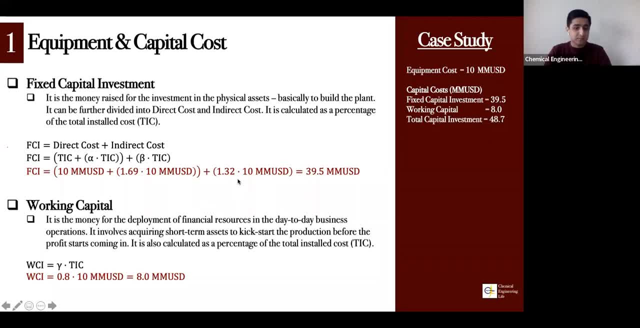 Your indirect cost, the indirect cost does not cover equipment. So there you don't have to add your equipment cost into the factor. 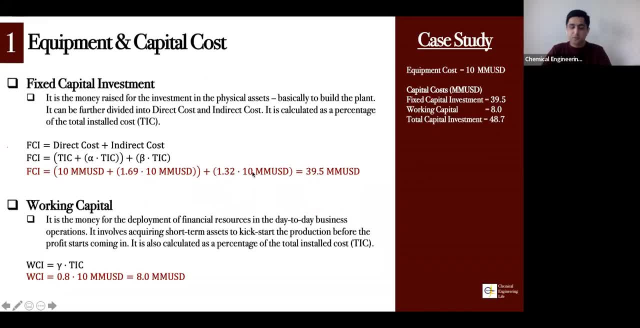 But you only have to multiply the factor with the equipment cost. 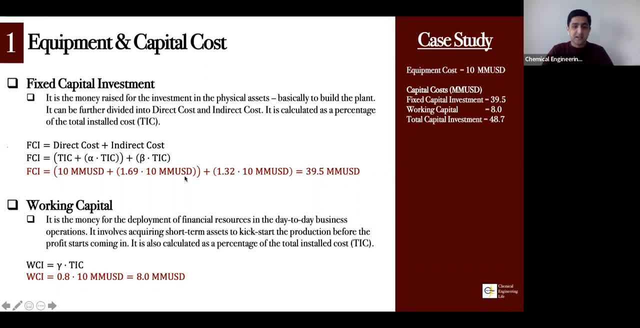 And that is something where a lot of people make mistakes that they may forget to actually add the equipment cost within the direct cost, thinking that it's covered, but it's not. 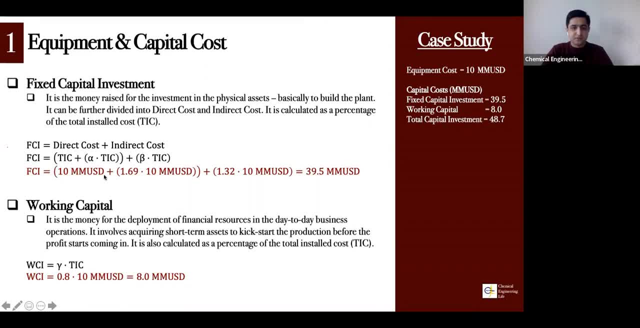 It's very important that you add them up together. And then you can see we have done the calculation here. So we calculated the direct cost plus the indirect cost. And that gives us the fixed capital investment of 39.5 million. OK. 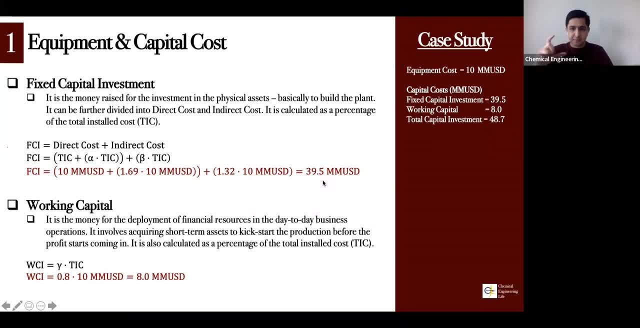 So that is our fixed capital investment. That means that I'm building up my plant. I got 40 million. 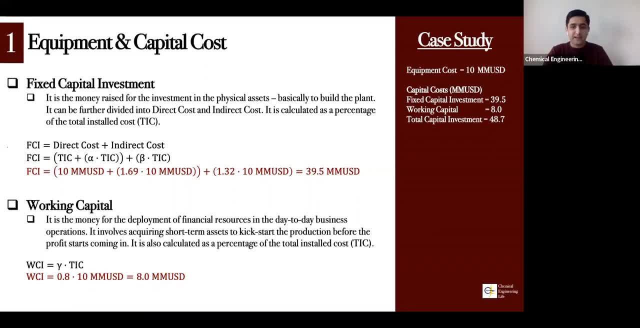 I built my entire plant. I have all my equipment. I have all my legal department ready. I have everything I need. I got the keys. Then you come down to the working capital. And the working capital is the money that you need in hand to actually kickstart your production. The working capital is also calculated as a fraction of your equipment. 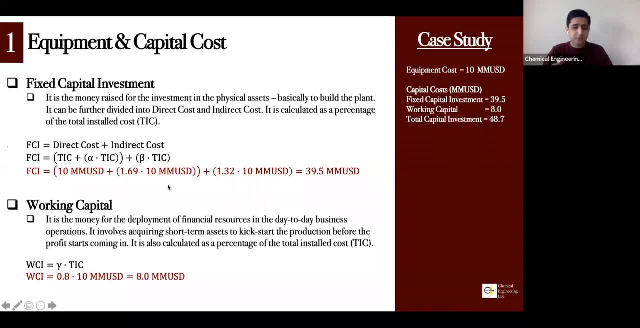 And as you can see on the screen, I have used 0.8 of the 0.8 as a factor. 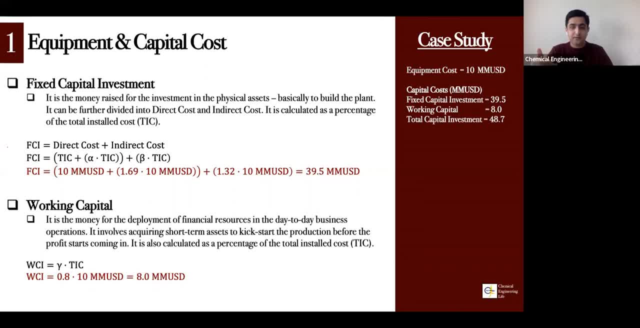 So 0.8 times by 10 million. That means that our working capital will be 8 million. 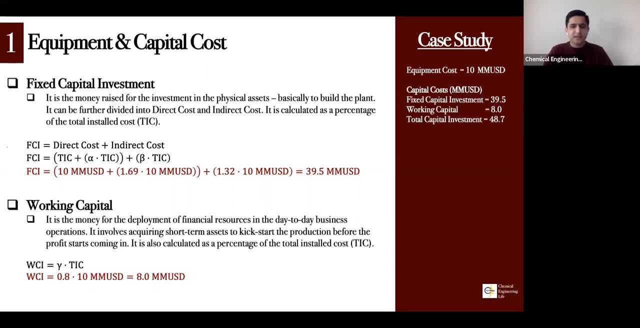 So what exactly does working capital cover? It covers everything that you need to kickstart your production. 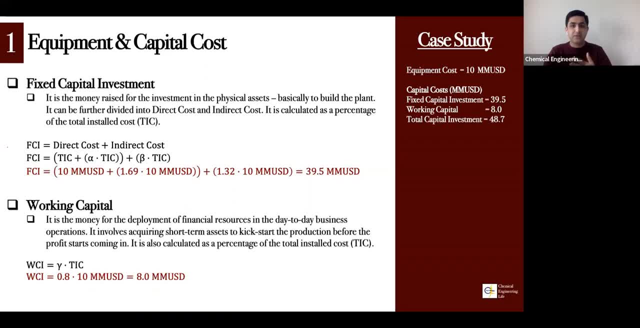 So I need to buy my raw materials. I need to buy my utility. I need to pay off my bills. I need to, you know, hire people. I need to pay people off for their salaries. I need to pay off the engineers and the operators. And you need to do it for at least six months. You need to do it for at least one year until you start making profit. 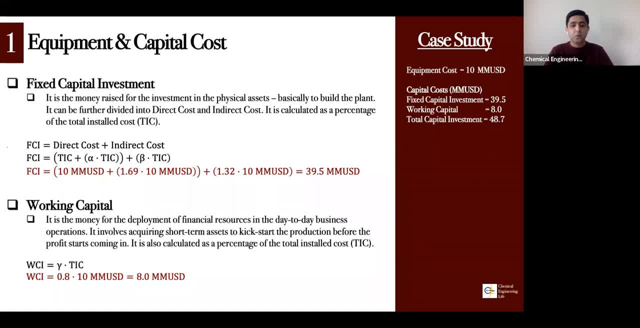 That money should be covered by the working capital. The working capital should more or less cover all of your expenses that you need to literally kickstart to your production. And in case you don't make a profit for the first two, three, six months, that should be covered by the working capital, because you cannot expect, and this is something we'll get into later on as well, that let's say you build the plant today. 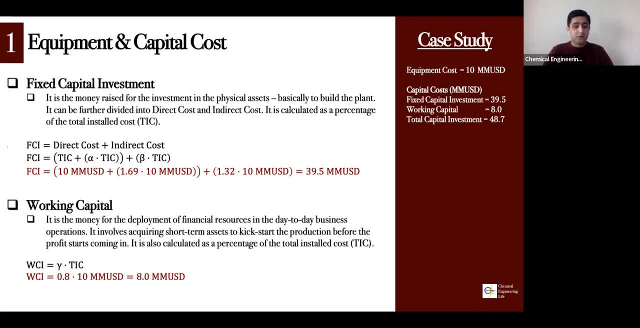 You can't expect that from tomorrow, you're going to have 100% production. 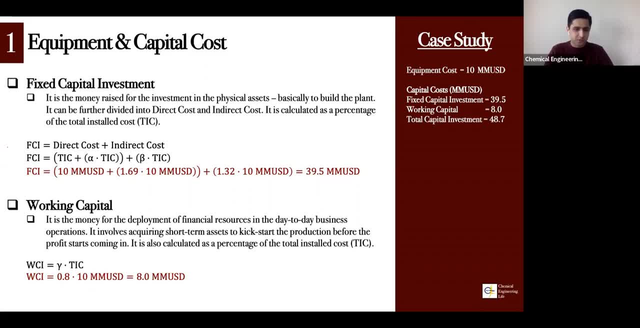 But instead, in the first year, you only have 80% production. In the second year, you have maybe 90%. 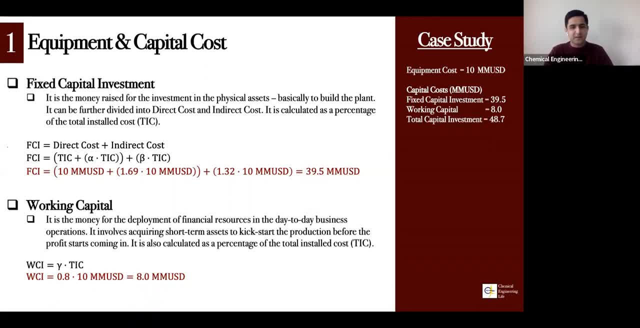 In the third year, maybe you might have 100%. So therefore, keeping that in mind, you need to use working capital to cover off the costs that might not be covered by your working capital. 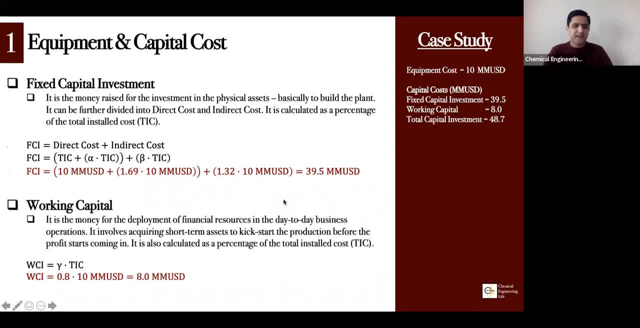 And like I said, it is around 0.8 factor multiplied by the equipment cost. 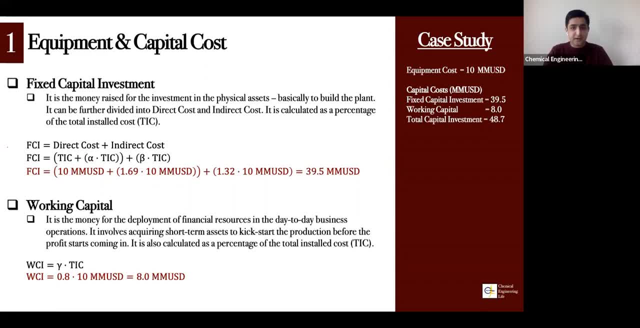 But just so you'll know, these numbers that I have used, they are all taken from literature, literature that I have found. 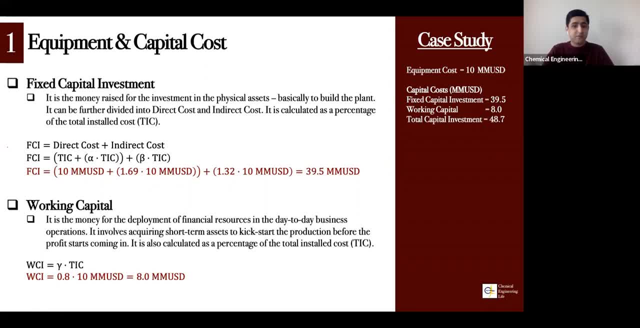 So you could also go ahead and find different literature, different values, different sources, and this entire analysis would look a lot different. 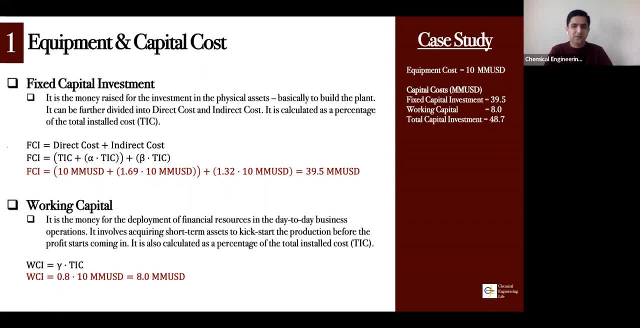 Like you could have used 0.9 for working capital. There is no fixed numbers. These are something that are taken off from books and from literature. 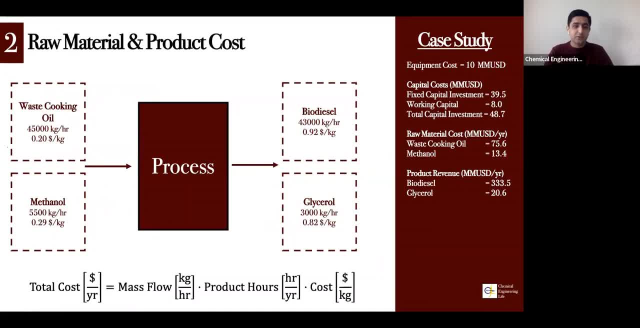 Moving on, then the next step that we need to do is, like I said earlier, we need to create our mass balance. And once you have your mass balance in place, then you are going to have your prices, your requirement per hour, and then your prices for each material. 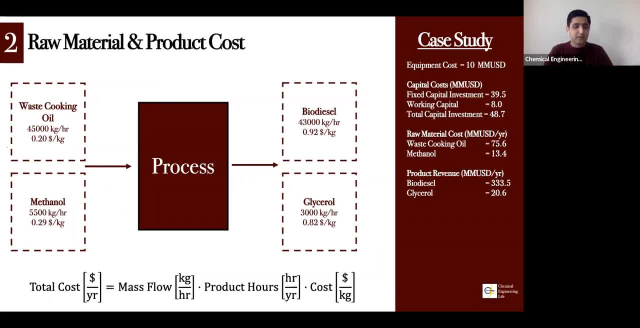 So as you can see here, for the process, we need waste cooking oil and methanol as our raw materials. And we are producing biodiesel and glycerol. The mass flow is given in hours. 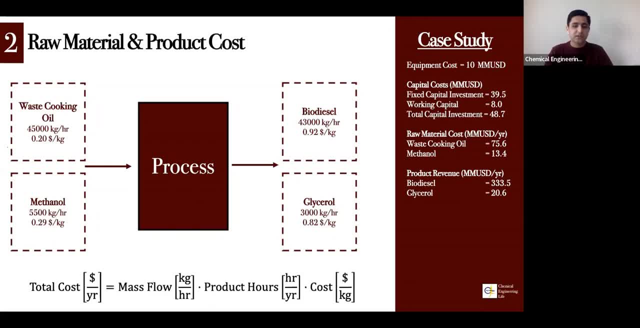 But when you're doing the technical economic analysis, you need to convert all of this into per year instead, because it makes a lot easier when you're calculating the economic metrics, which I showed you earlier, because the economic metrics are based on annual income, on annual cash flow. 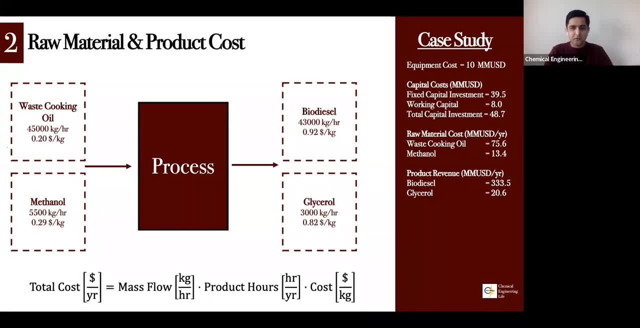 Therefore, it's a good idea to convert all of that into years. The way you convert it into years is that, first of all, you have to calculate the total cost. 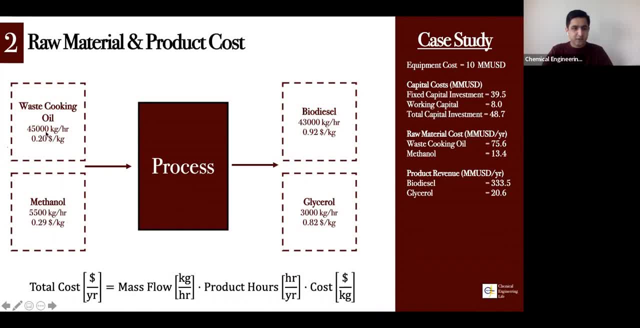 So you have the total cost. That is calculated by the mass flow, which we have right here. 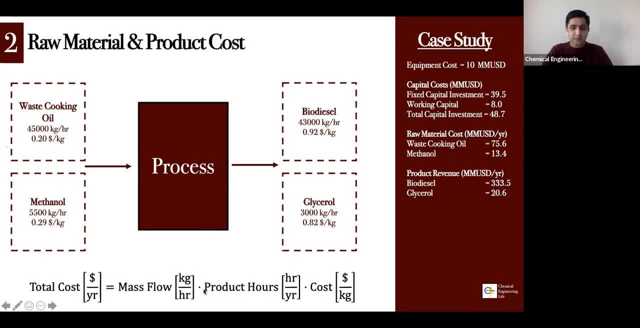 So we have over 45,000 kilograms per hour. You multiply it by your production hours. 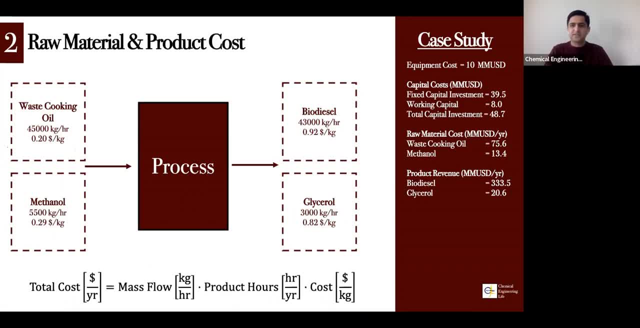 So let's say how many hours you're going to be running your plant per year. So let's say you say that you're going to be running it for 24 hours for 350 days. For these calculations, I have selected that we're going to be running it for 24 hours for 350 days per year. 15 days are then kept aside for maintenance or cleaning or whatnot. 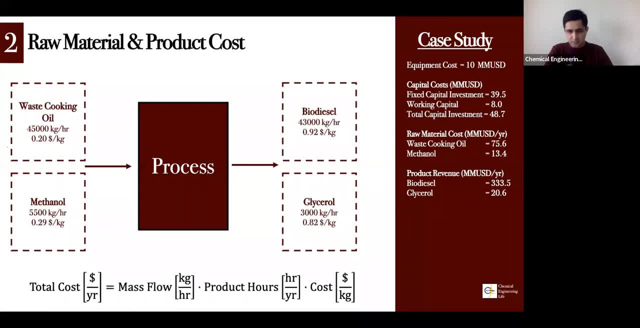 But we're only going to be running it for 350 days. Then you do 24 multiplied by 350. That would give you your production hours multiplied by the cost. 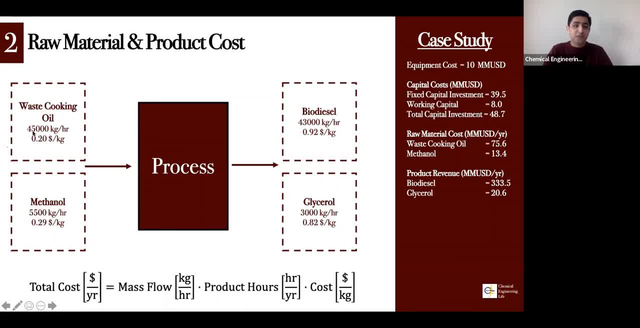 Now, you can see that we have a waste cooking oil. It is 45,000 kilograms per hour. We multiply it by our hours. 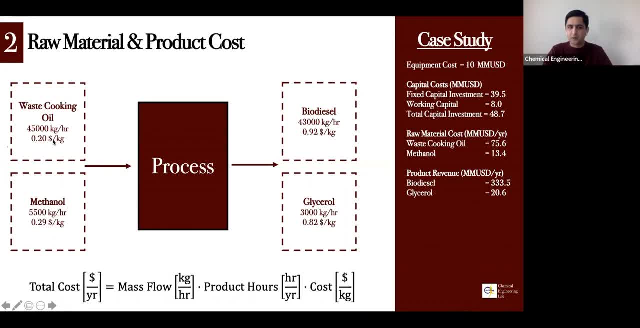 Then you multiply it by the cost. It is $0.2 per kilo. 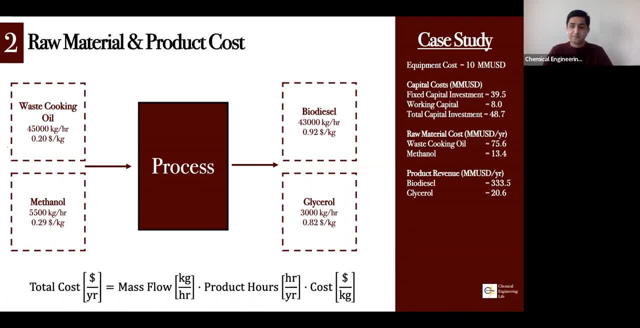 And you end up getting your dollars per year. And you do that for each and every raw material and for each product. The raw material cost is your expense, right? 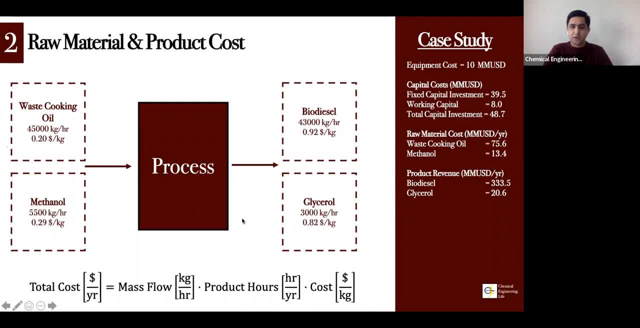 Because you have to pay that from your own pocket. And your product cost, that is your revenue that you're going to be raising by selling your product. 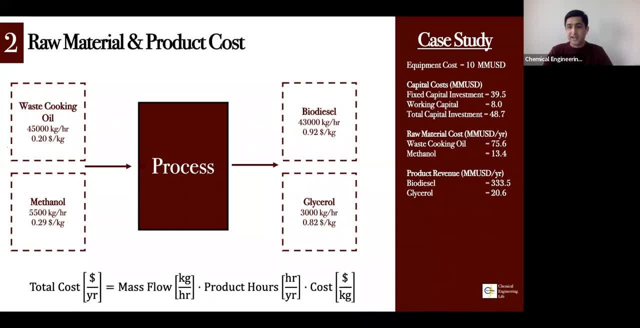 The more expensive your product is, the better it is. And the cheaper your raw material is, the better it is. 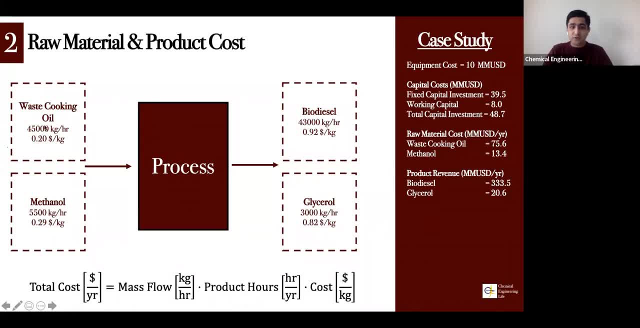 Like you can see already here, for example, the waste cooking oil, it costs $0.2. It's very cheap. The reason it's very cheap is because it's a waste stream. 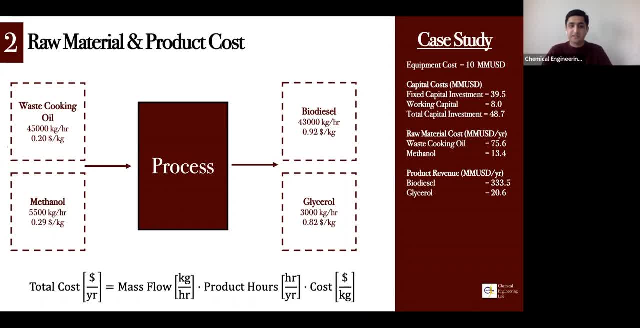 It doesn't possess any useful needs in the market right now. It's a waste stream. 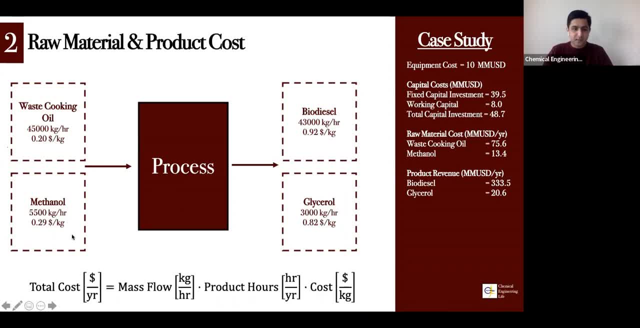 So you're buying it off very cheaply. Methanol, again, it doesn't cost that much, around $0.3 per kilo. 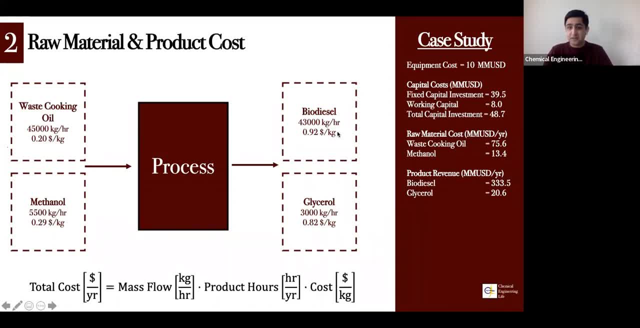 And of course, biodiesel, it has a very strong market. Even today, it is very expensive. It is $0.9 per kilo. 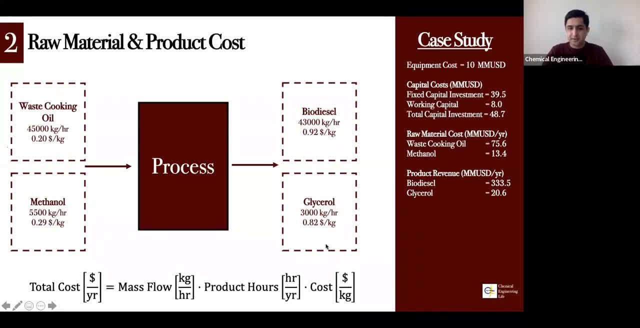 And then we have glycerol, and the glycerol is $0.8 per kilo. 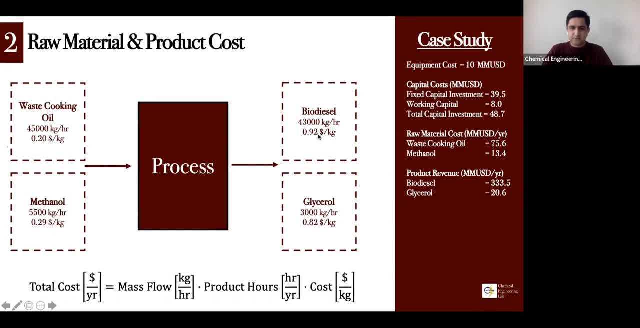 The way we find these prices for each of these materials, it is not simply enough that you find the cost of biodiesel 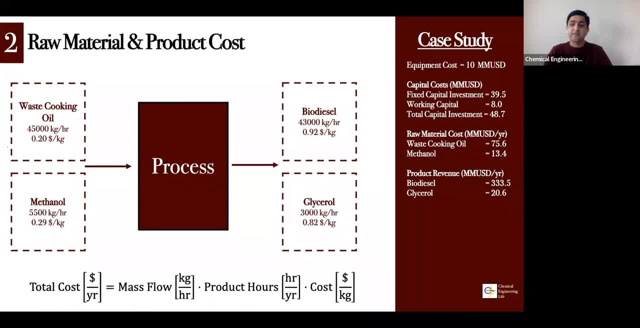 on the 8th of May, 2022, and you select that value. 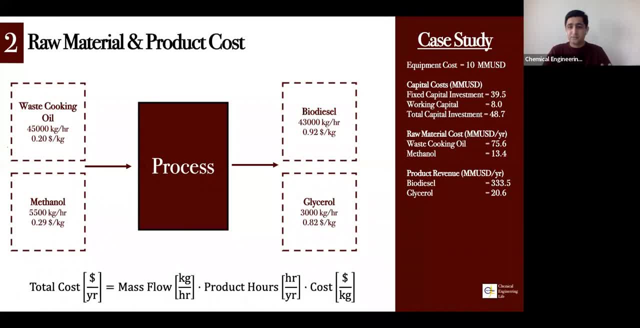 Because these values are entirely dependent on the market. Therefore, the best way to do it is that you find the prices of your product for the past one year, or for the past six months. The longer back you can go, the better it is. So you pick the... 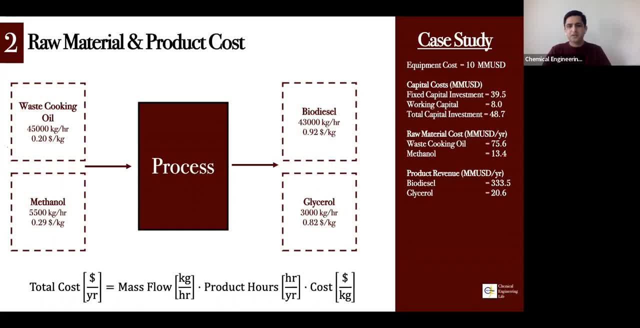 So let's say if you go back one year for 2021, so you select the period between January, 1st of January, 2021, up until 31st of December, 2021. Then you find your maximum price of biodiesel, and you find your minimum price for your biodiesel. And then you find the middle line for the top plus min divided by two. 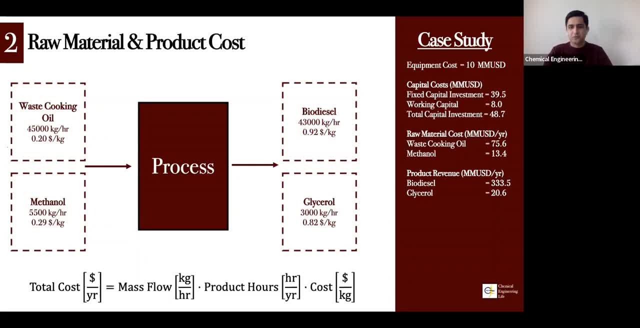 And then you can use that price as your cost for the technical economic analysis. 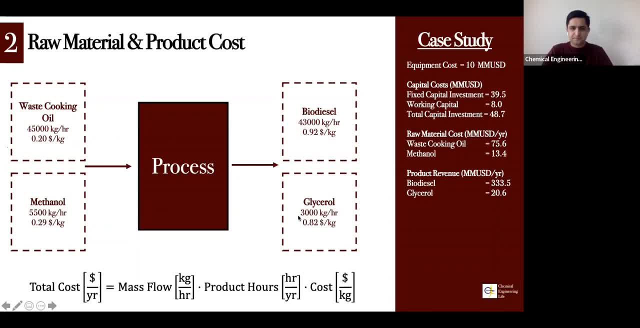 And we have done that, and I've done that for all of them. 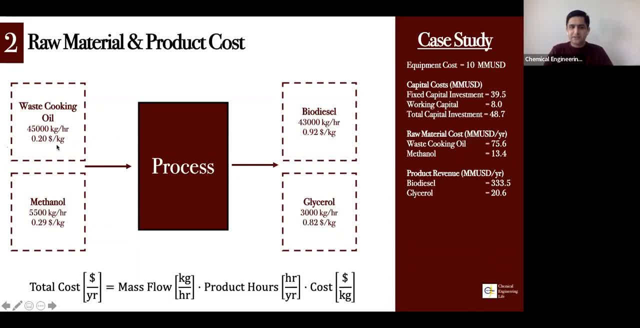 The waste cooking oil, sometimes it's not very easy to find the prices for some of these materials like waste cooking oil. 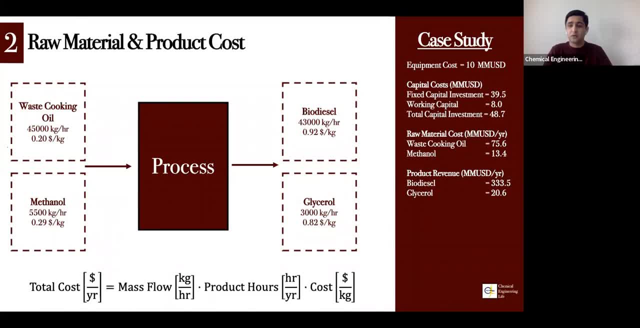 You can't really go in and find the price of waste cooking oil on how much it cost it a year ago, or how much it costs now. 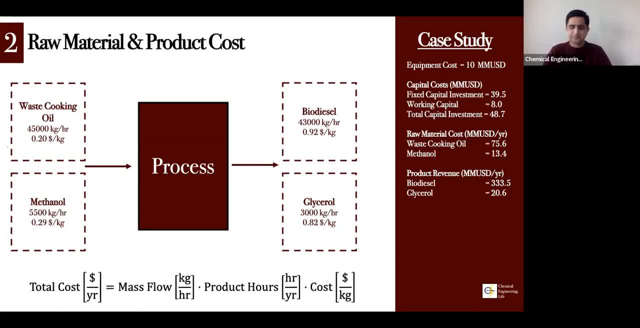 Therefore, you can always use the price that you find from the source. 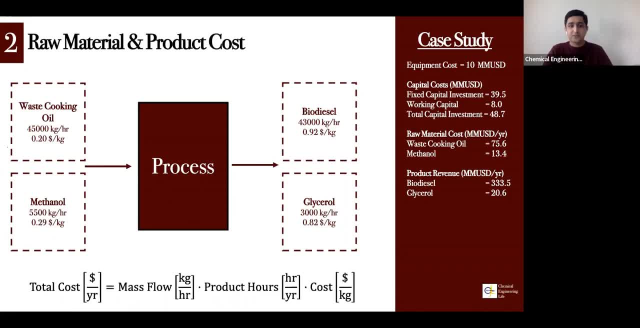 And of course, if you're using a price from let's say 2015, then you need to account for that you convert that price using the inflation factor to the year that you are doing the technical economic analysis. 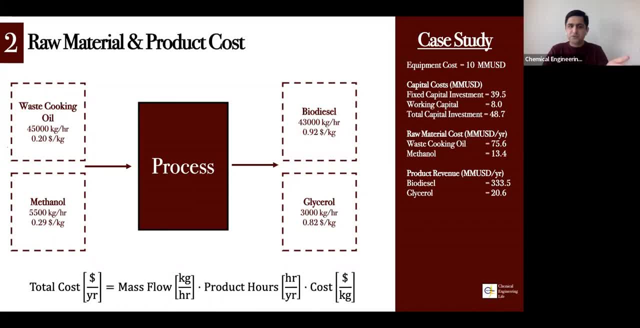 So for example, if waste cooking oil costed 0.2 in 2018, and you're doing the analysis now, then it's a good idea to multiply it by the inflation factor. 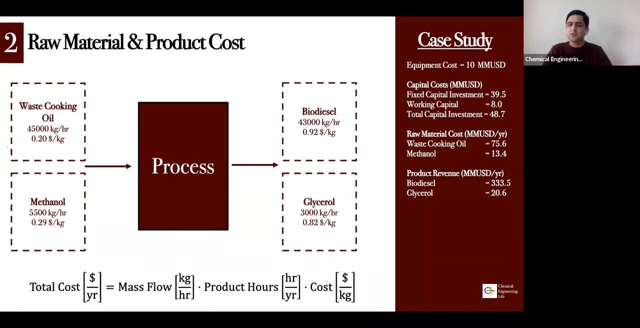 And the inflation factor is, you can just find that to Google. 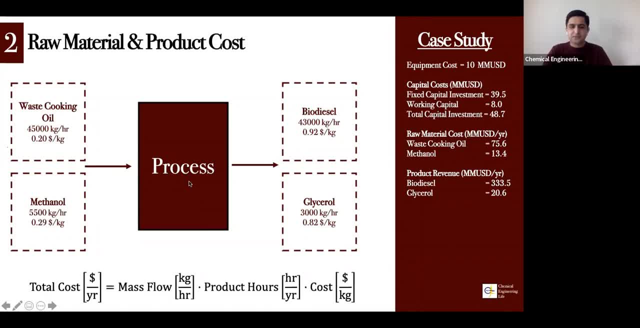 And then you just multiply the inflation factor with your price. 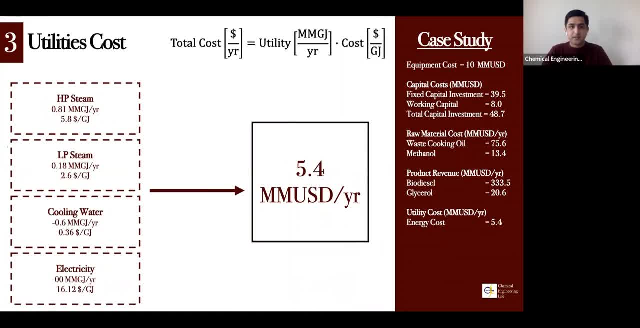 The next phase, the next step, then that is the utilities cost. 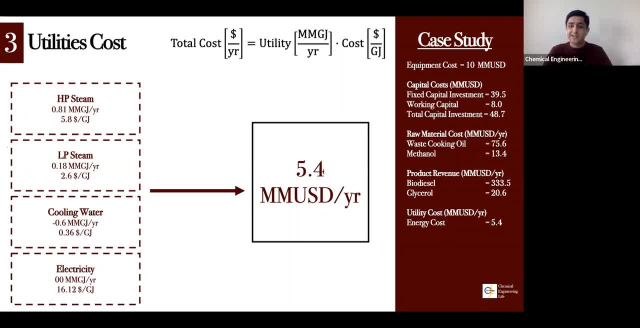 And the utilities cost, these are very important because the utilities is what is going to keep the plant running. 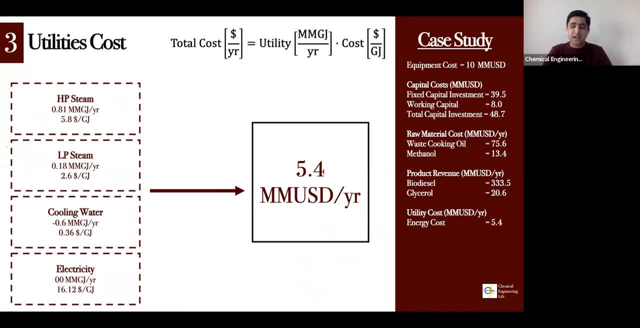 The main utilities that we have in our plant, that is the high power steam, the low power steam, cooling water, and electricity. 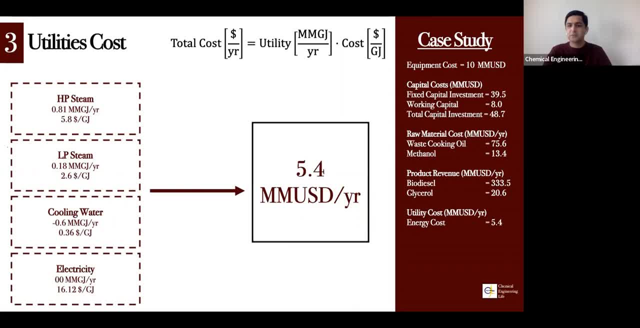 And they also tend to be refrigerant if you are cooling something below zero degrees or so. Luckily in this case, we don't have any, so I have not added that into the slide. 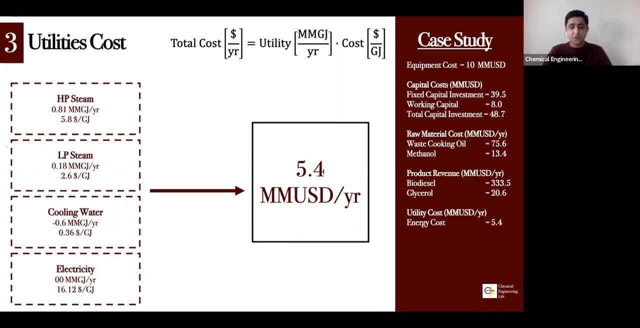 The high power steam and the low power steam, they are two different, they differ in temperature and pressures. 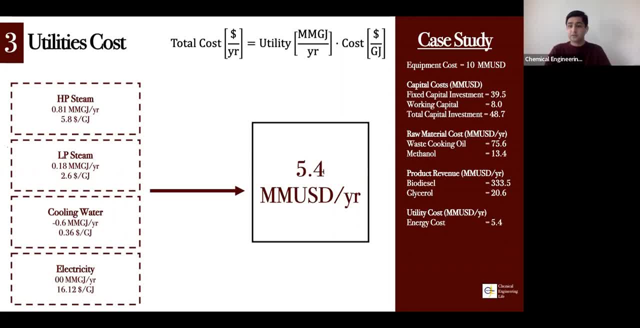 So if you are, if you want to heat something up to, let's say 300 degrees Celsius, 400 degrees Celsius, then you have to use high power steam. 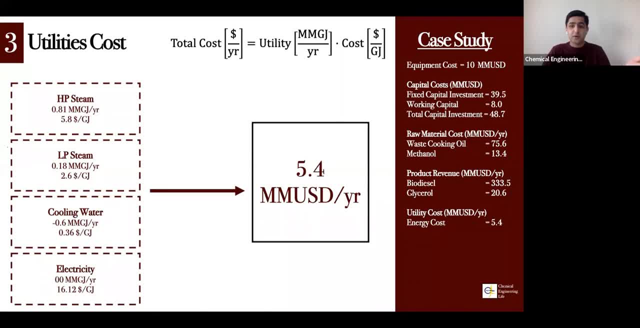 Anything at a very high level, you need to use high power steam. 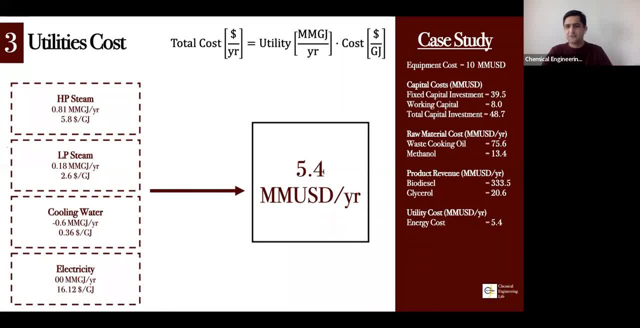 But if you're using, if you're heating something up to only, let's say 50 Celsius or 100 degrees Celsius, then you can, then you can enjoy it with a low power steam. So a low pressure steam. 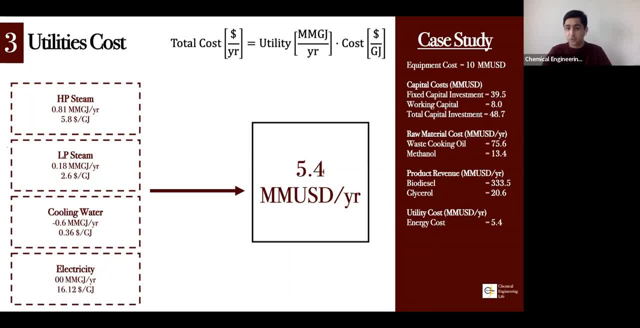 And then of course you have cooling water. The cooling water is again to cool, your equipment, streams and whatnot. 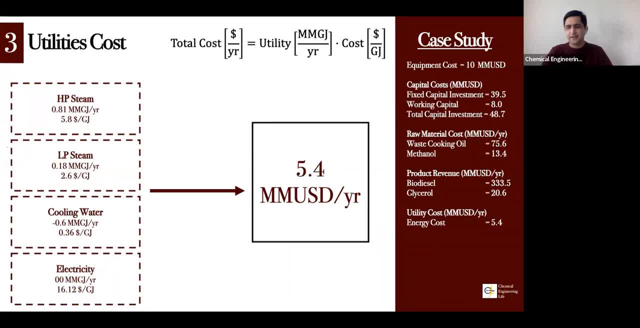 And then you have your electricity. Electricity is only mostly used by pumps. 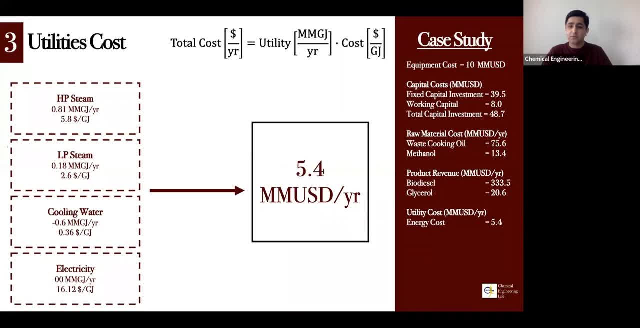 And then every production facility does have a requirement for electricity. Like you have your computers, you're going to have your automation system. You're going to have your process control. That also needs electricity. And that is also taken as a percentage of our total capital investment. 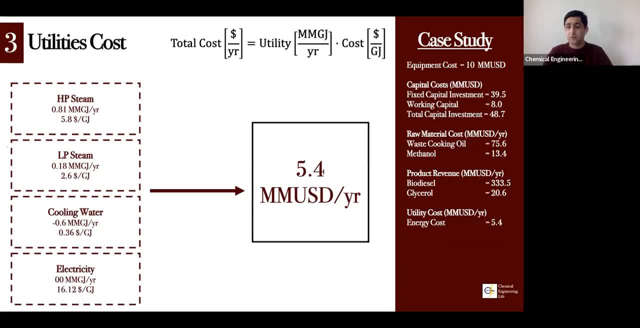 But majority of the cost for your electricity should come from your, actual equipment that you're using. 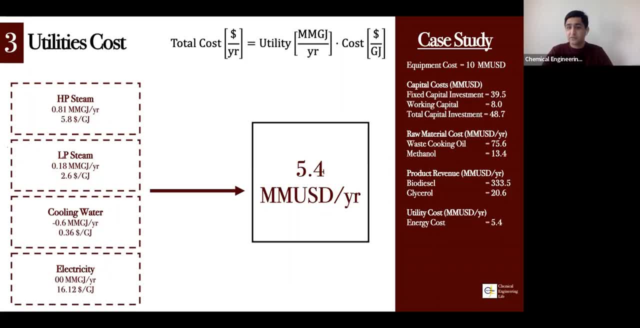 Luckily in this case, we only had a few pumps. So therefore there was not much of a need to actually use electricity. 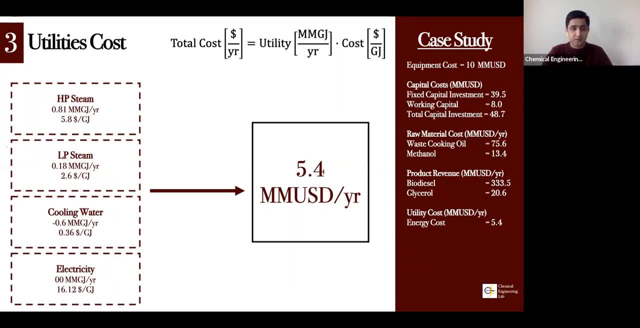 But there was a very high need of using our steam, low power steam, low pressure steam, high pressure steam, and also cooling water. 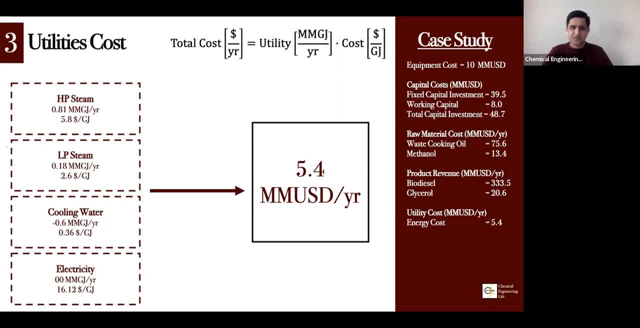 And these prices might look, also might change depending on what source you're using. Like I have, I found a source for high pressure steam to be $5.8 per, gigajoules and so on. 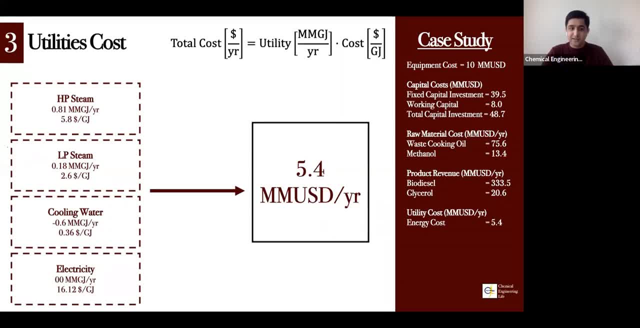 And when you are finding the prices, it is very important that you keep an eye on the units that you're working with. 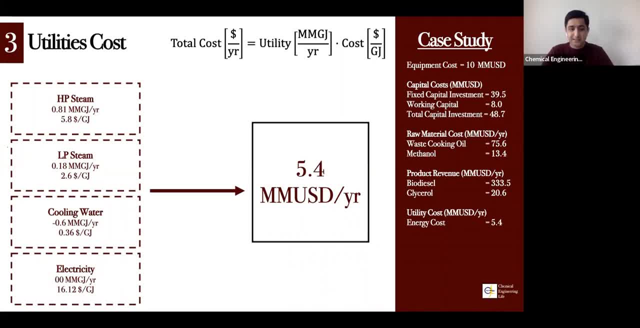 For example, you can see here for electricity, typically we use watts. But since I found the price in gigajoules, 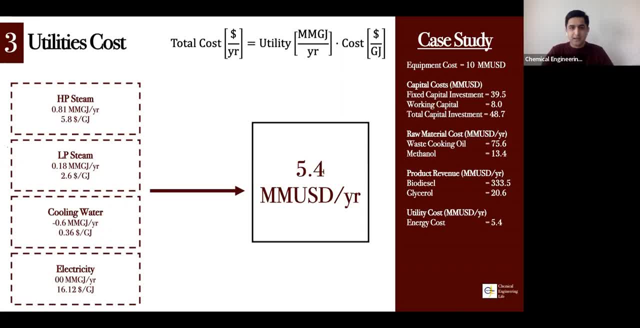 so I converted that into gigajoules. And the way, and then once you have your requirement, 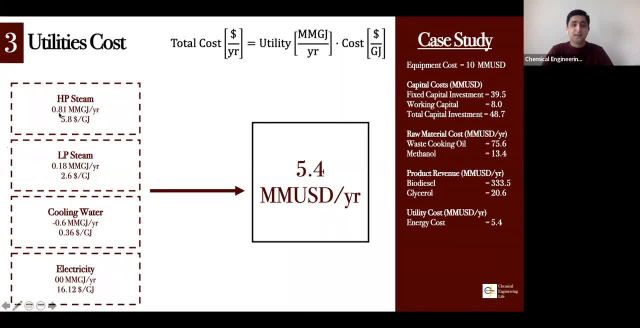 so for example, for high pressure steam, our requirement is, 0.8 million gigajoules per year. 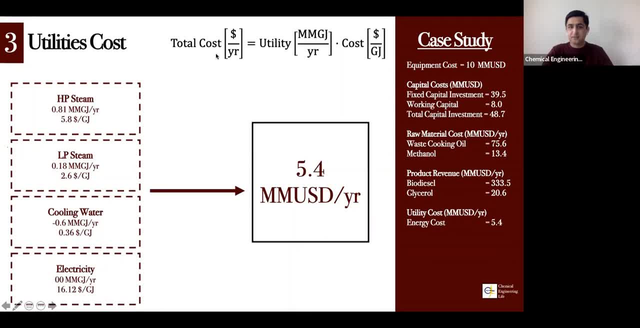 You multiply that with your unit price and you find the total cost per year. 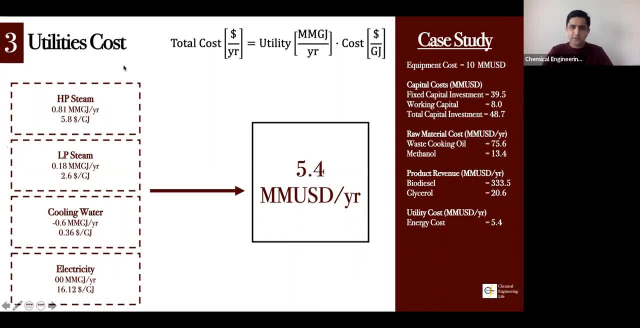 And again, just like our raw material and product cost, it's a good idea to do it per annum. 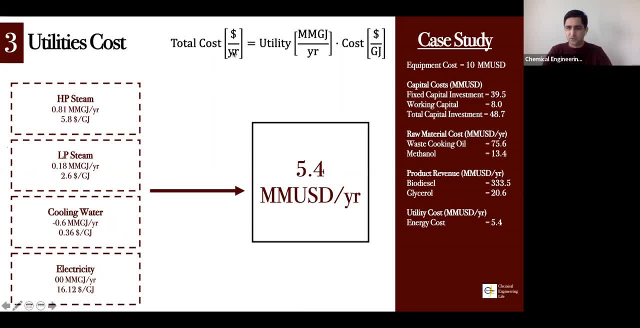 So you do it per year, instead of doing it for per hour or so. It just makes your life a lot easier afterwards. 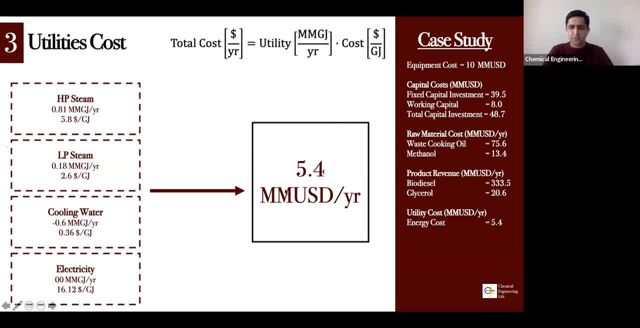 And then you calculate the sum of all of the costs and that was to be $5.4 million. 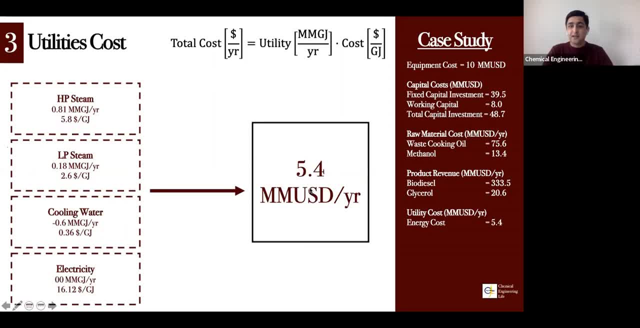 That means that for me to be able to pay for my utilities, it's going to cost me $5.4 million per year. After the utilities, then we come on to our waste costs. 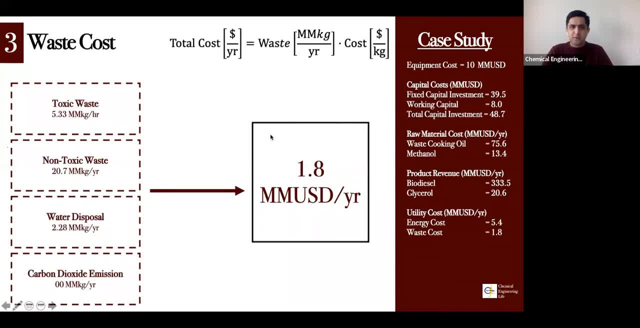 The waste, contrary to what many people might believe, you're not allowed to simply throw your waste into the rivers. You're not allowed. That's not allowed by any, by any law. 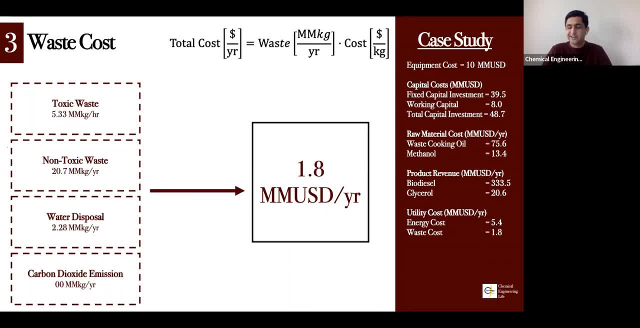 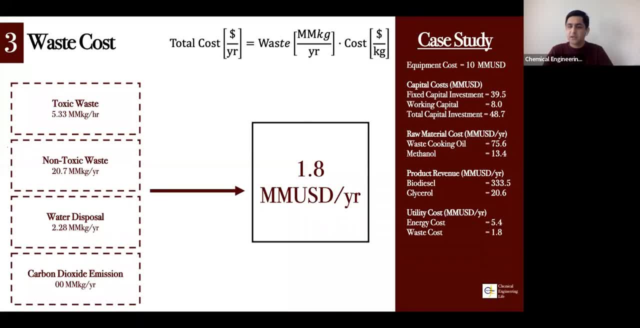 Toxic waste is everything that is considered to be toxic. For example, carbon monoxide, that is a toxic waste. Non-toxic waste could be something that's not considered not toxic. I believe ammonia is not considered to be non-toxic waste. So if you have ammonia, waste that you will only have to pay the price that is required for non-toxic. 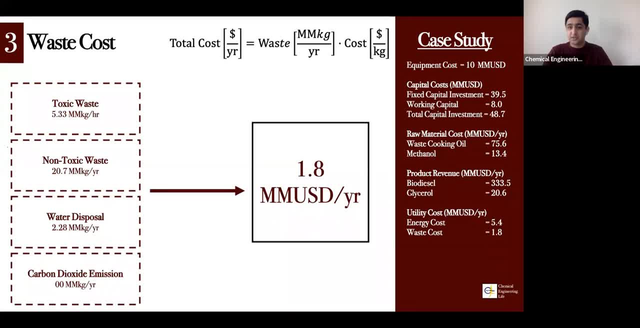 But if you have carbon monoxide emission, then that actually comes into toxic waste that we need to pay for. And of course, a toxic waste costs a lot more than non-toxic waste. And that is also to, to encourage different facilities to reduce their waste production as much as possible. 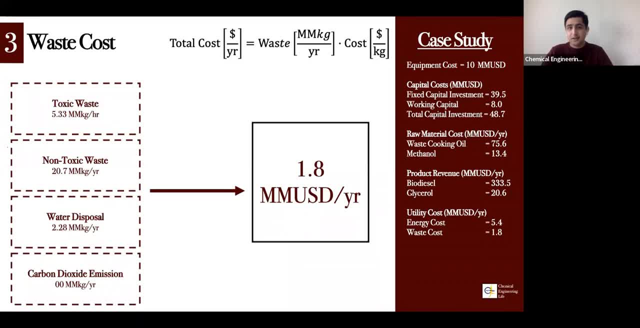 But then of course we have our water disposal. Every water that you use, all the water that you're using in your production for cooling, for cleaning, for all the uses, again, you have to get rid of it. 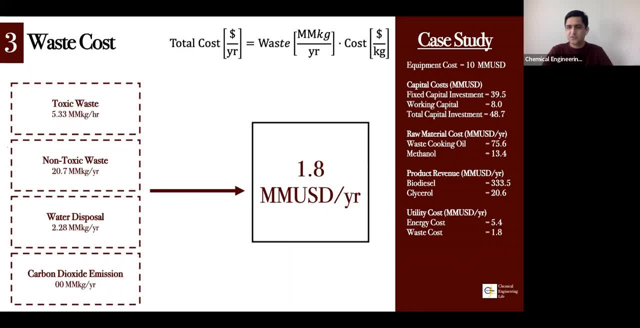 And that also costs money. The money can be in terms of transportation costs. You need to take it away. You need to give it to someone else. That needs to be covered. 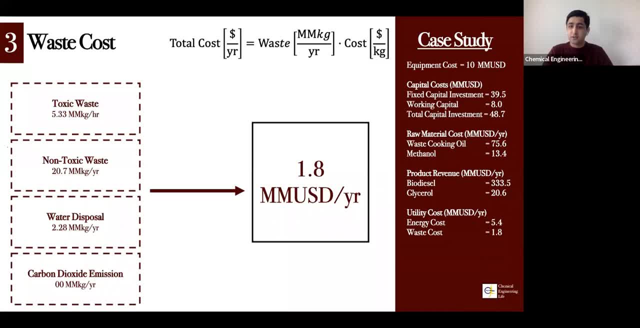 It is always a good idea to explore the possibility that you can treat the water instead of just disposing it off, because if the water is clean, you're only using it for, for example, if you have a fermentation reactor and you're only using water as a, to dilute the, within the reactor, then you can always treat it and reuse it back into the process. 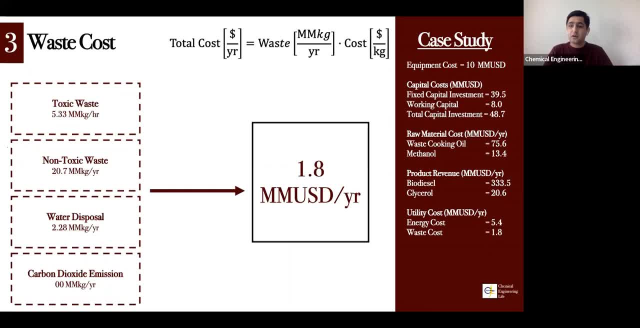 It does seem that the water treatment might cost you more in terms of the disposing it off. But in the long run, you actually save a lot more money and your sustainability metrics are going to look a lot better if you're reusing that stream of water back into your process. Okay. And finally, 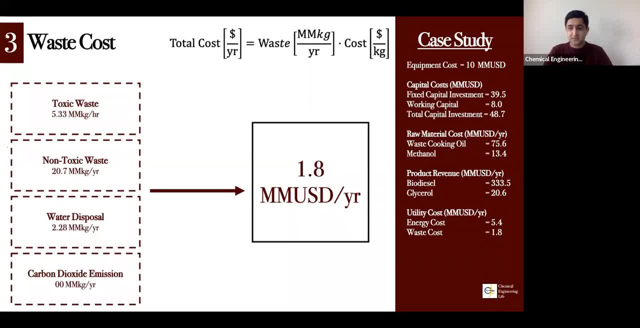 we have this something called a carbon CO2 tax. 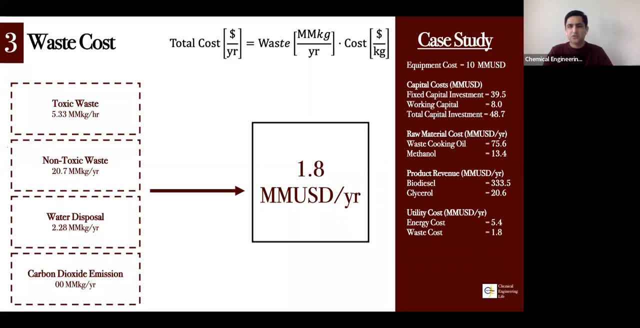 Did they have it in some countries? They don't have it in some other countries. 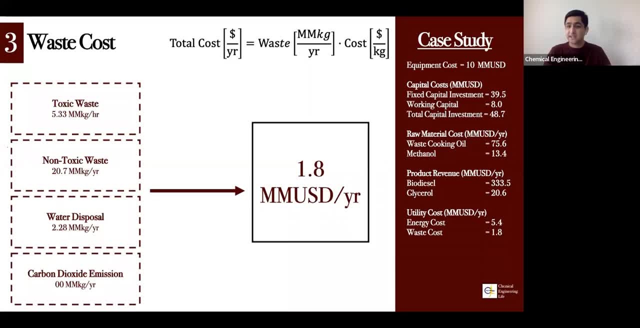 So if you're doing your production in the US or in Texas, Americans, they have a carbon dioxide tax. That means that if you are releasing carbon dioxide into the environment, depending on the emission level, you need to pay a certain amount per kilogram. And that is something that you need to check. And that is something that you need to check on. Instead, 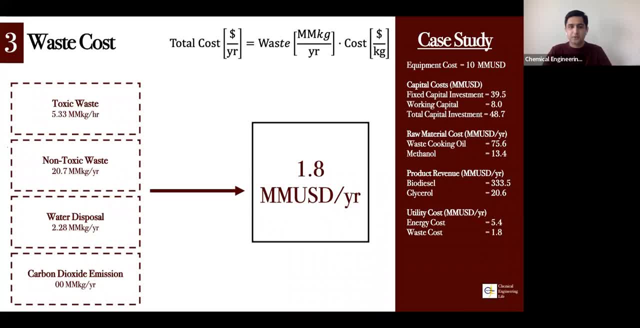 if you're doing, if you are analyzing your plant that is being produced in, in let's say Germany, then they have a different carbon dioxide. Some countries don't even have it. Like I believe if you go in, in some countries, I believe I checked in Nigeria. They, they don't have, they don't implement a CO2 tax. But some countries do. 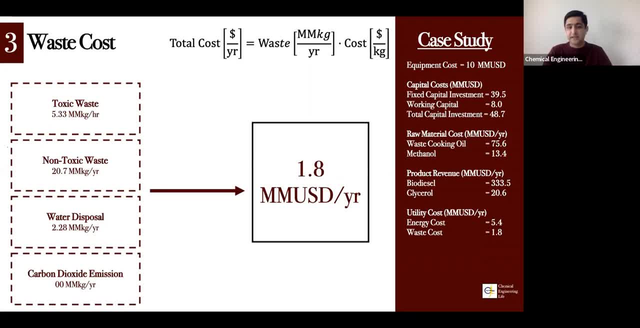 And that is very important that you check it out. If they have it, they need to include it. 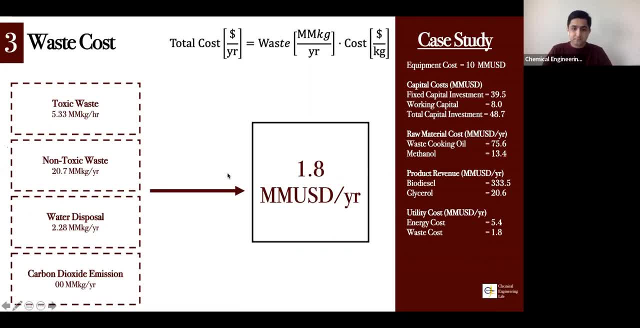 If they don't have it, then you can get away with it. 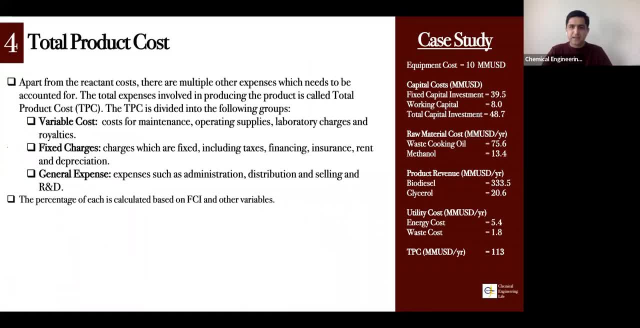 So now we have covered our investments. We have covered our raw material costs and now we have our utilities costs and we have our waste material costs. These are the costs that are important for our day-to-day operations. 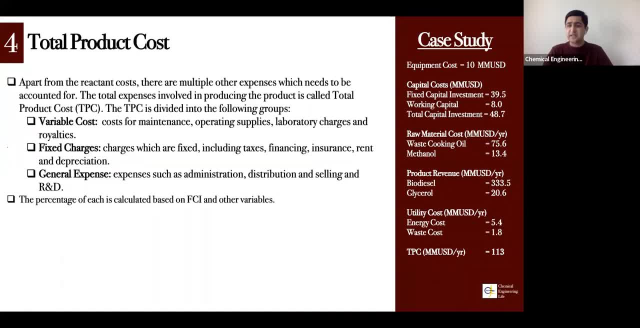 There are no other main major expenses other than these three areas. 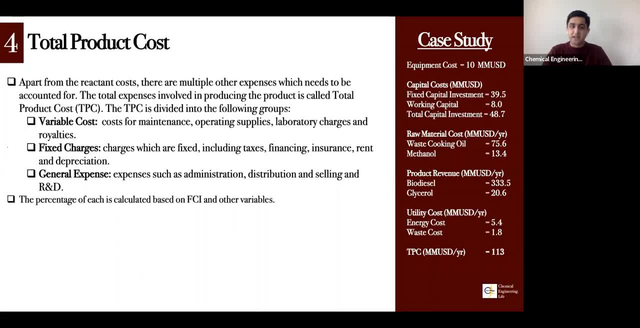 So using those values, and we can then calculate our total product cost. The total product cost is, is the amount of money, is your total expenditure per year that you need to run your facility or run your production. 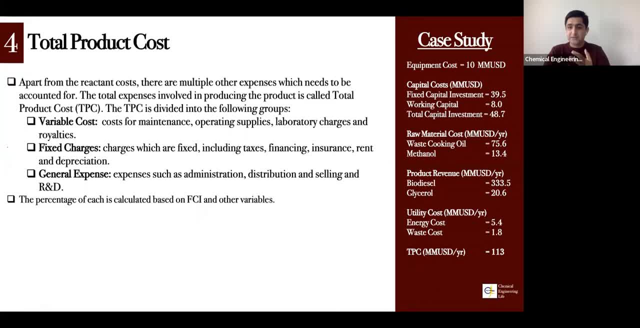 It covers everything from raw material, waste, utility, but also all the other admin expenses that you might have that are, that are important for running a production facility, like, for example, you need R&D expenses, you need marketing, you need distribution, you need to hire people, you need to have, you need to have tables, you need to have screens, you need to have seminars, 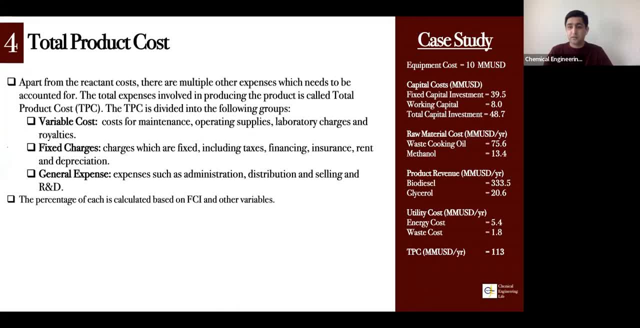 you need to have safety additions. All of that needs to be covered by the extra expenses. 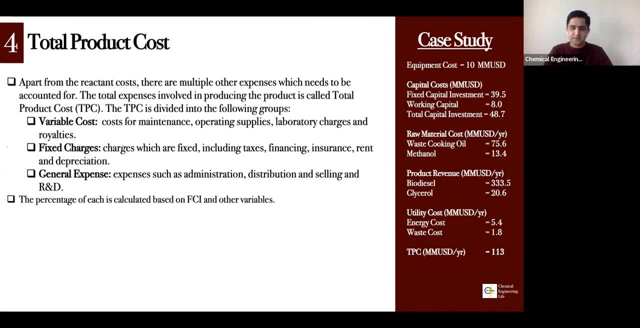 And that is calculated as earlier than you were calculating the capital investment. So, 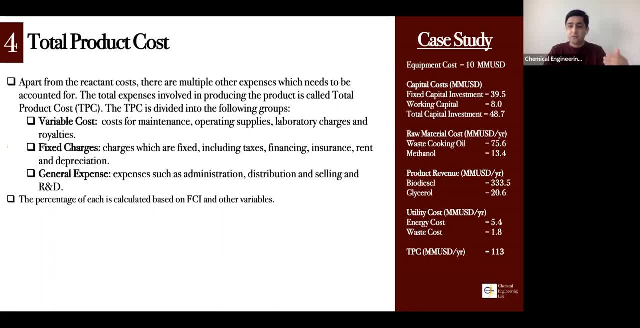 we used our equipment cost as, as a basis for calculating our capital. But when we are calculating the total product cost, then we need to use our fixed capital investment as a basis. 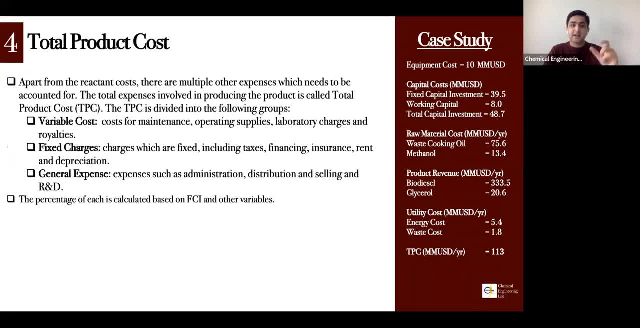 And then we find the factors multiplied by the fixed capital investment to calculate all the other variables. 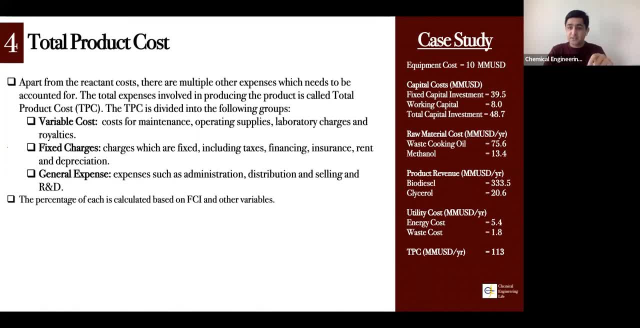 So our variable cost or fixed charges or general expenses, they're all calculated as a factor of, as a factor of our fixed capital investment. 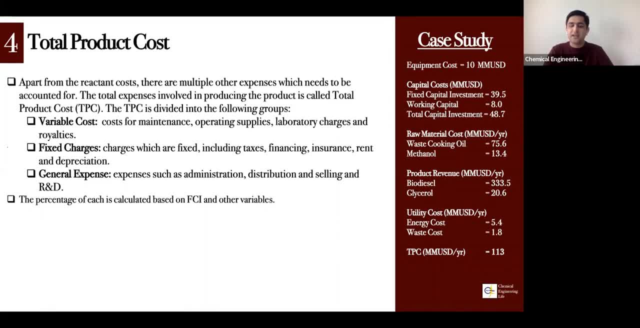 And upon doing so, then you can, then you can know how much money you need. 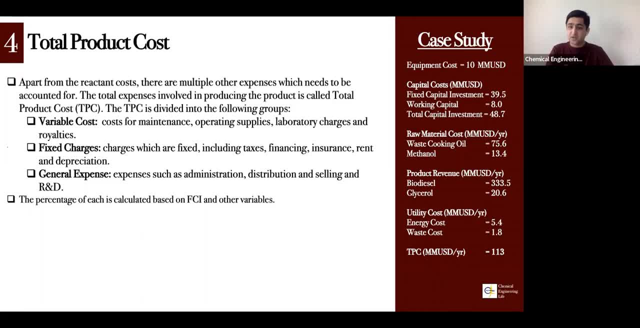 And it will always be higher than the sum of all the other expenses that we have talked about so far. So if you can see on the screen right here. 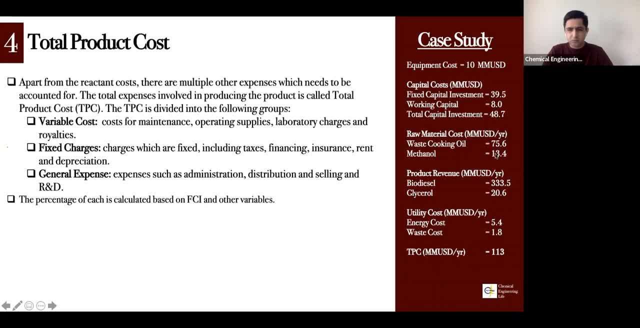 So, our raw material, it costed about around 88 million. 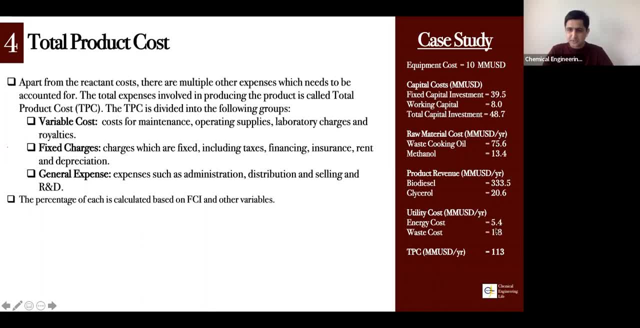 Our utilities, it was around 7 million. 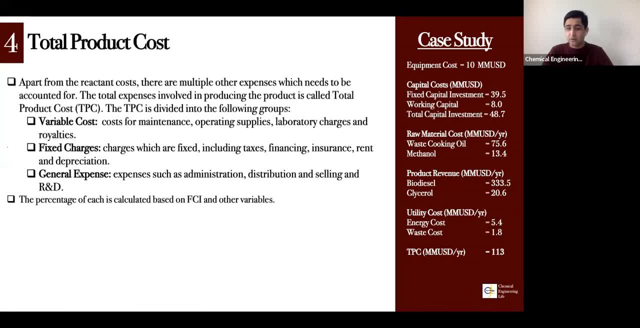 So if you add them up together, you have around 94, 95 million dollars per year as the sum of utility cost and the raw material cost. 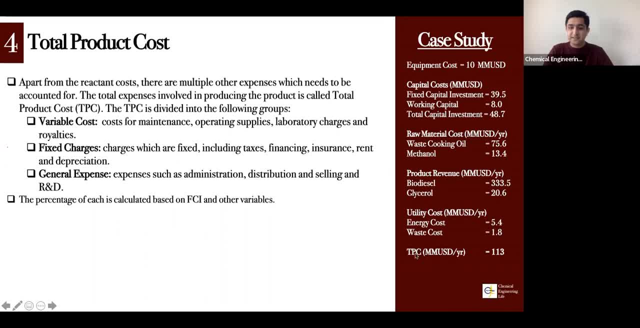 But doing all the other calculations, our TPC ended up being 113 million dollars per year. So that means the additional 20 million that came on top of this, that came from all the other expenses that we have talked about here. 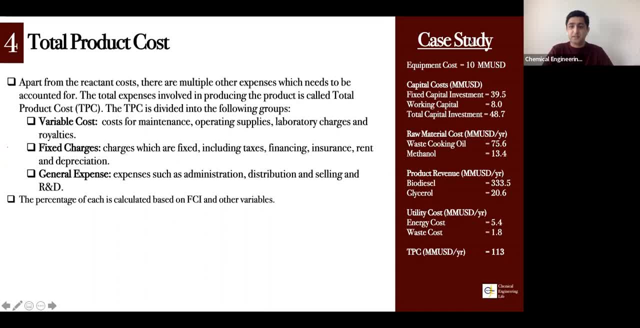 The variable cost, fixed charges, general expenses, that calculated as a factor of our capital investment. 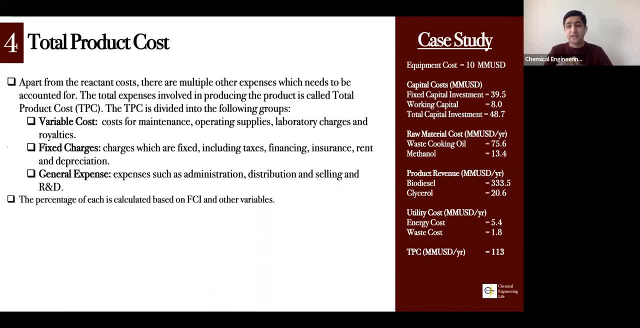 And again, all these charges, all these factors, they are to be taken from literature. 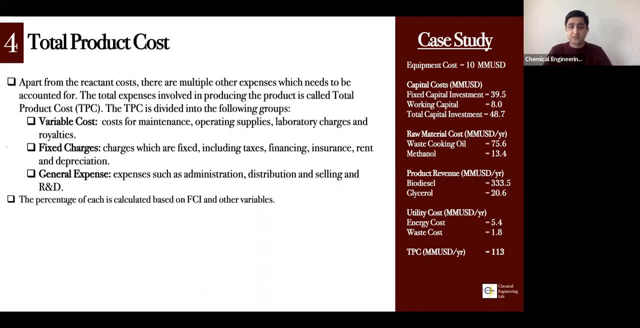 I would highly suggest if you are looking up, if you are designing the process, then you use this book called Plant Design and Economics for Chemical Engineers. 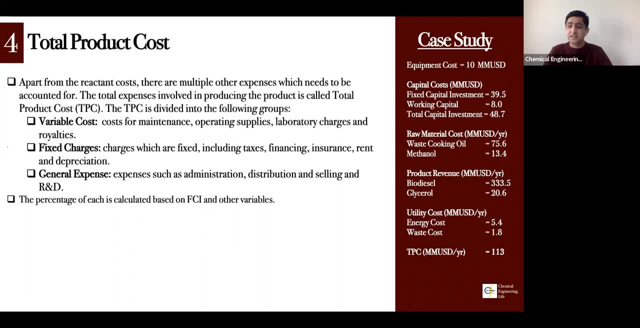 They have, they have an edition from 2015, I believe. 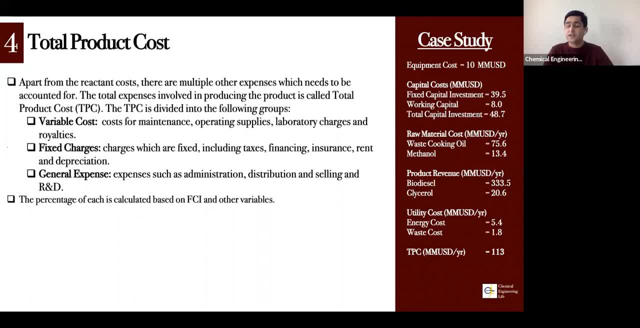 And they had, they have provided with all these other variables and all the factors that you might need in calculating the total profit. And if not, then if you find any literature, any research paper that have done this technical economic analysis, they always provide these factors that they have calculated. 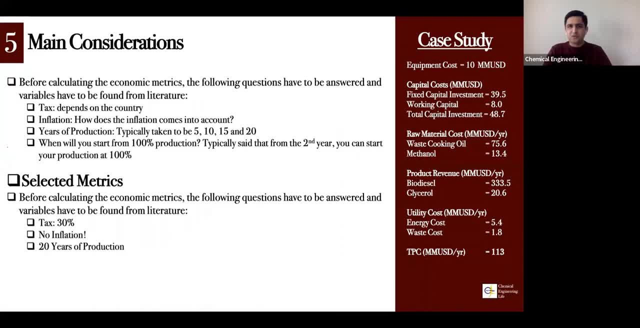 And of course, these factors, always remember that these factors, they're always given within a given bracket. 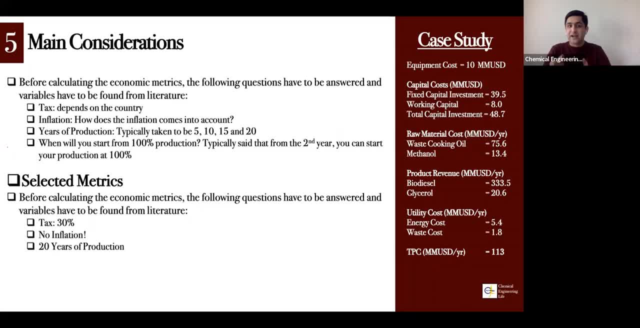 So you can't just say, I'm going to pick 500% of my capital investment will be my gain. My investment will be my general expenses. They are always within different ranges that you need to select. 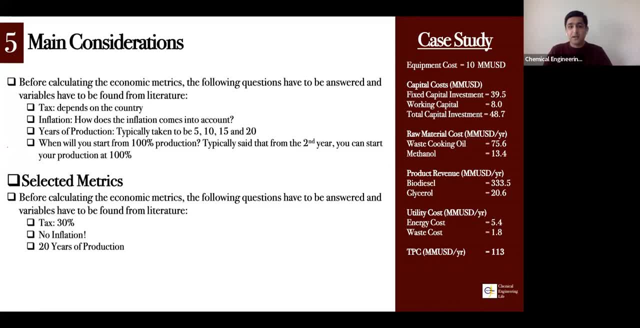 So, so for now, we have our TPC, we have our revenue. 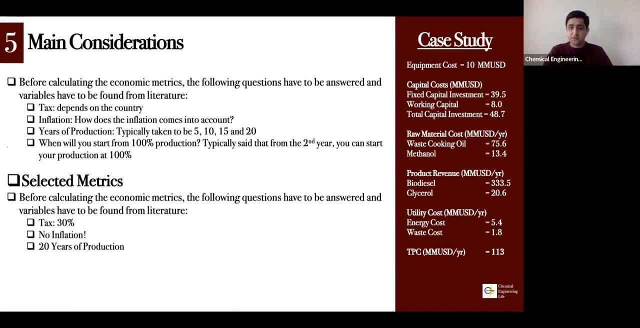 But before we go into calculating our economic metrics, we need to, to take something into consideration. 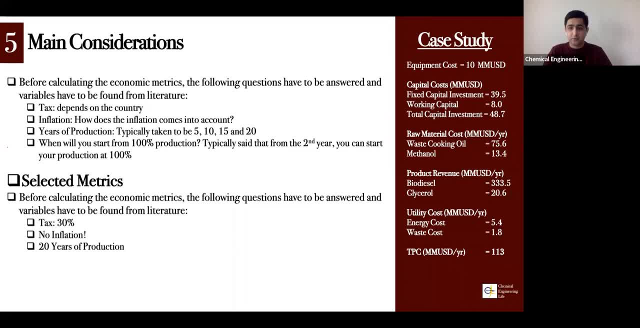 The first thing that we need to take into consideration is how much tax you will be paying for your production. If you are, for example, in Denmark, you need to pay around 25% tax. If you are designing a plant in the US, you need to pay around, around 30% tax. 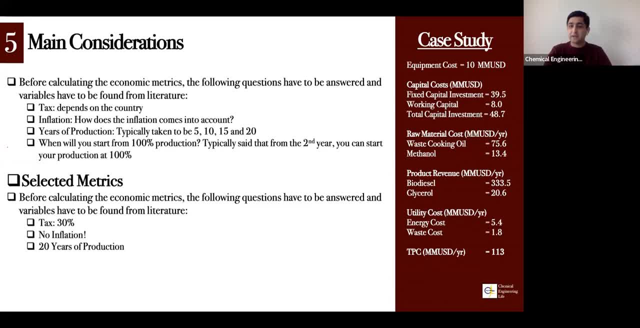 Again, for example, when we are working with biodiesel, the biodiesel is eligible for subsidy by the federal government. 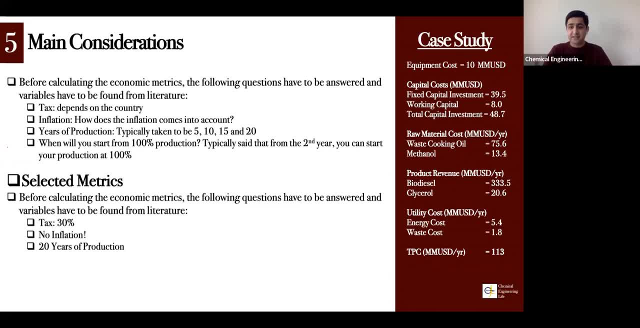 You can also take that into account. That means that you will not be paying as much tax as the other production are paying. 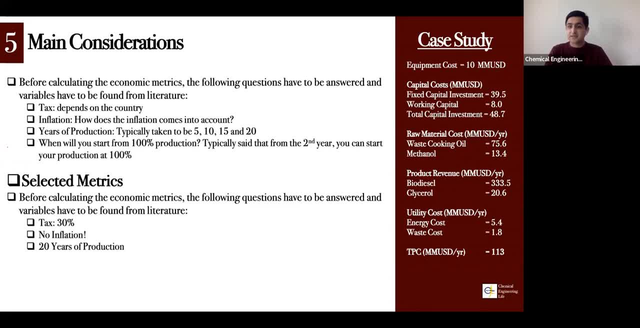 But, you know, but the idea is that you need to find the correct tax that you're going to be paying off, because it is the money taken off from your profit. 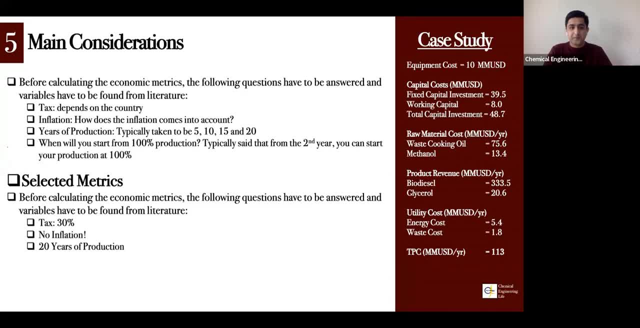 So it's very important that you put in the tax. Inflation, you can take inflation into account. And the way you take into account is that there are two ways of doing it. Either you can take the inflation for your product. So that means that if I am selling my biodiesel today for $0.9 per kilo, due inflation is going to get more expensive, right? So next year it's going to be more expensive. The year after it's going to be more expensive. And that's a great thing. That's great. 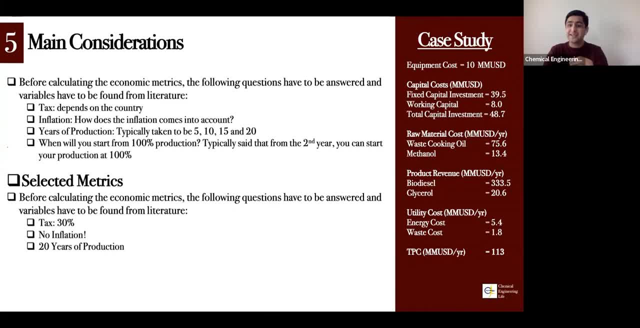 But at the same time, inflation is also going to hit our raw materials cost, our utilities cost, our waste cost. So therefore, we need to remember that when we take inflation into account, it's going to affect all of our materials, all of our expenses equally. And that's the first part of it. 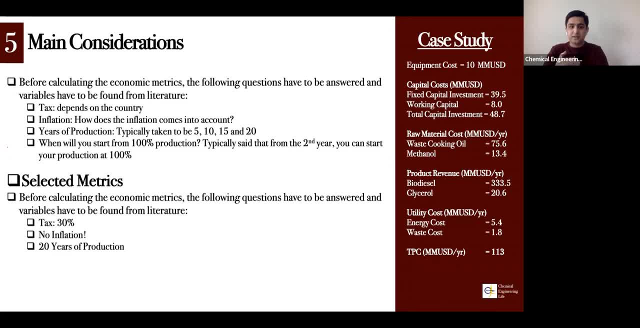 The second part is that you could also take, take inflation. Like for example, when we are building our facility, you need to identify how long will it take for you to build your production. So let's say you build your plant in three years. In the first year, the cement was, they had a price X. 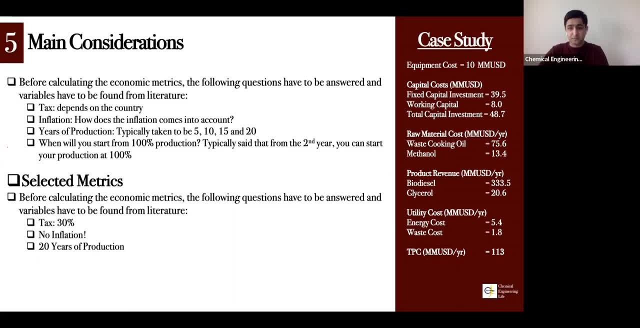 The second year, it got more expensive. The third year, it got more expensive. 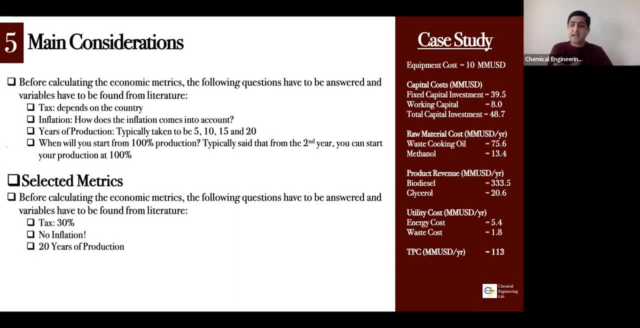 So you also need to take into account for inflation for that area as well. And so that means that you need to divide it up into two different parts. 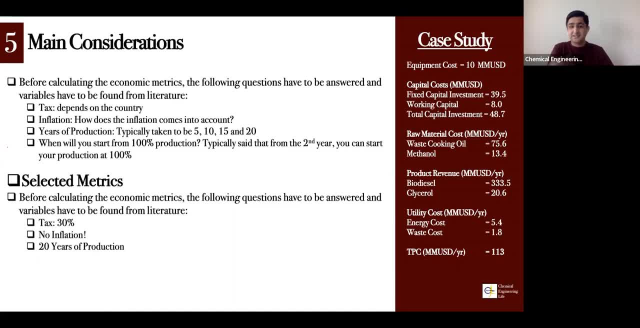 For the first part is when you're building your facility. And the second part is when you're running the day-to-day operations of our facility. 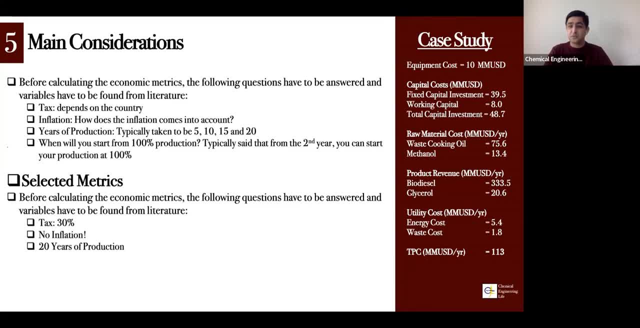 For the purpose of this study, I have taken inflation to be zero. 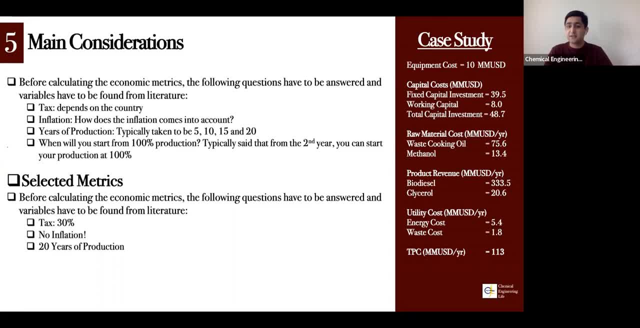 So that we assume that we will not be affected by inflation. Everything that costs today will cost the same in 20 years. 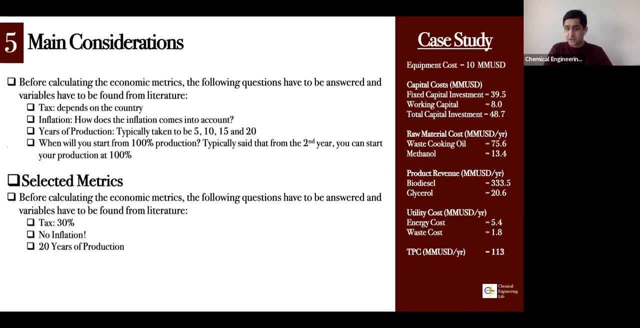 But if you do want to take inflation into account, but the problem is that it is very difficult to, 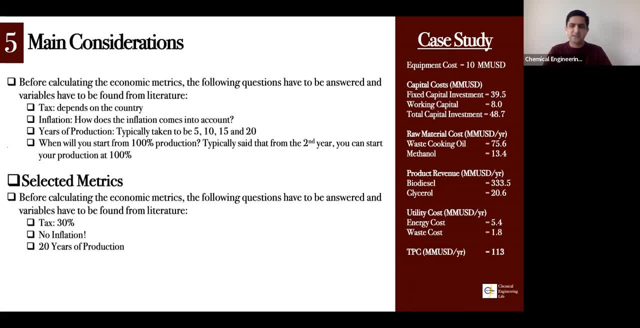 to see how inflation will increase in the next coming five years, the next 10 years. 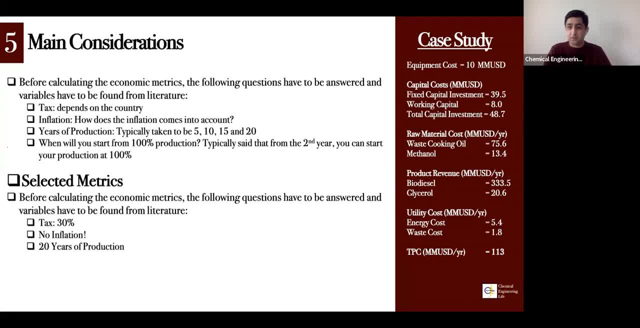 Something that we saw during this COVID crisis, for example, inflation has skyrocketed because inflation is directly dependent on different international political instability, instability, and so on. 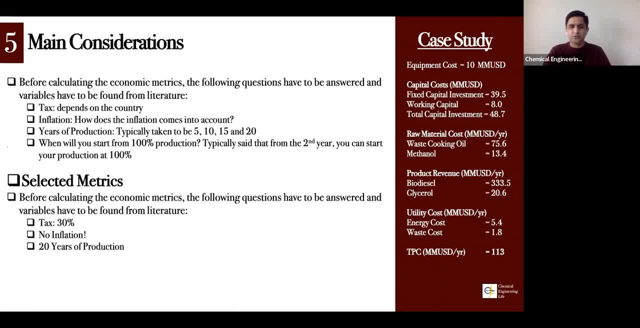 So therefore it can get slightly difficult to find a value that you want to use. One way to do it is that you can look at how inflation, has changed in the last 10 years, in the last 15 years, and then you can use the same model, the same value for the next 15 years. 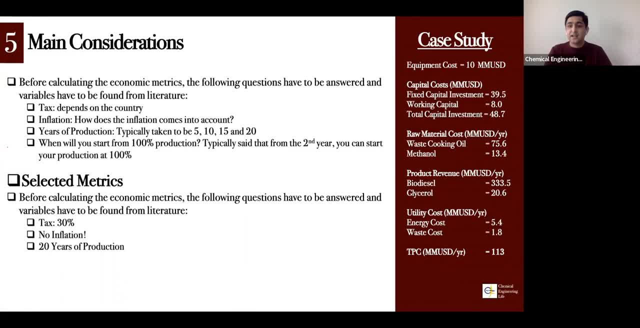 But again, that is again, a huge assumption, assuming that inflation will be the same in the next 15 years as it has been in the last 15. 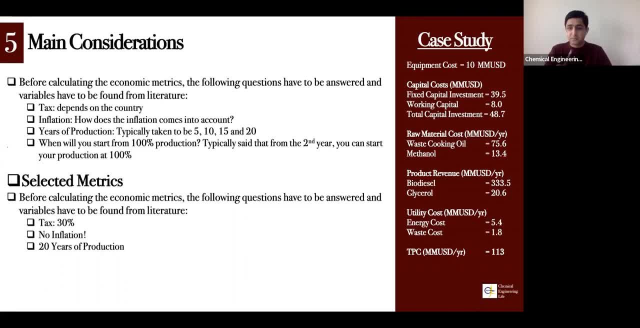 But that is one way to do it. But like I said, for the purpose of the economic metrics that I have calculated for this webinar, 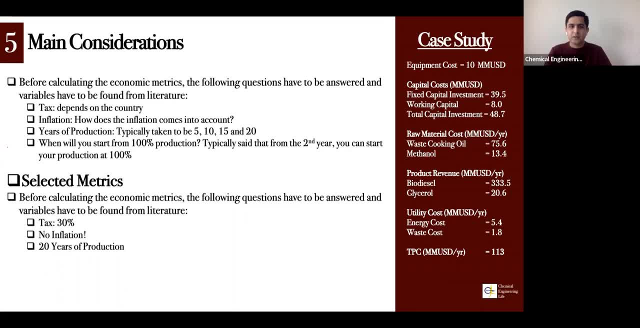 I have taken inflation to be zero. So I did not take that into account. 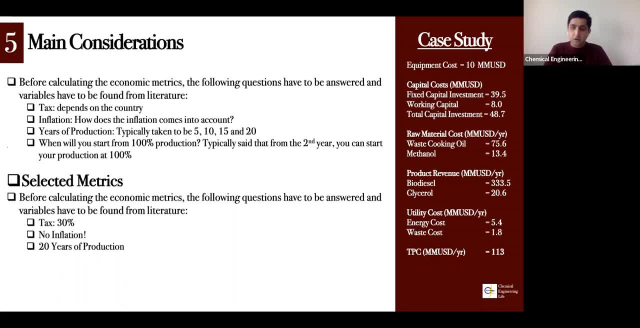 Then you need to, then you need to calculate, consider, consider how long do you want your project to be? 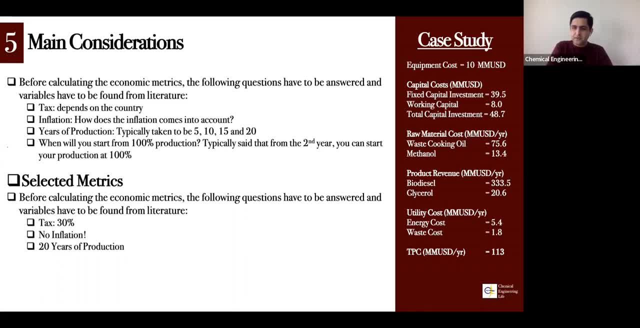 And so typically it's five years, 10 years, 15 years, and 20 years. 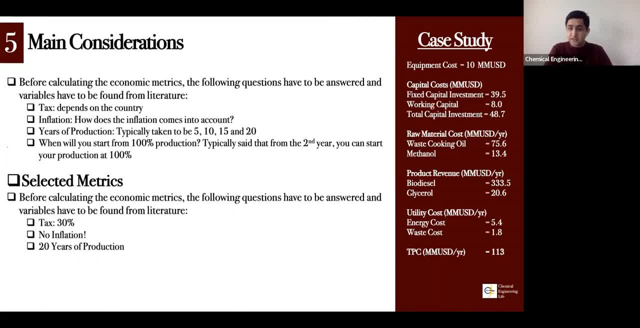 Now, the thing is, the shorter project time you select, the less money you'll make. So that's a given. 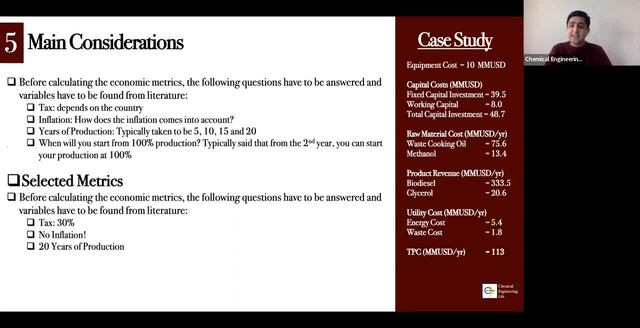 If you select something, a production facility for five years, it might prove not to be so profitable because you don't really make that much profit in five years. 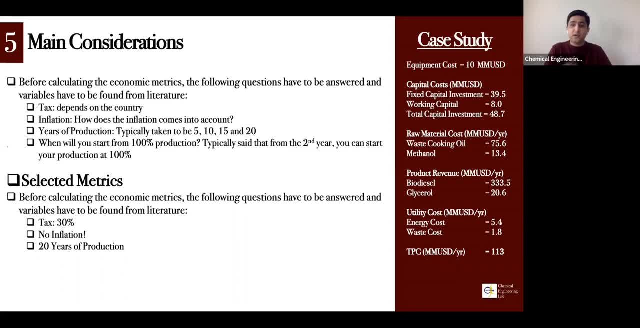 If you were to do something in 10 years, your NPV would be a lot higher. You would end up making a lot more money. If you do something for 20 years, then you end up making a lot more money in that way. 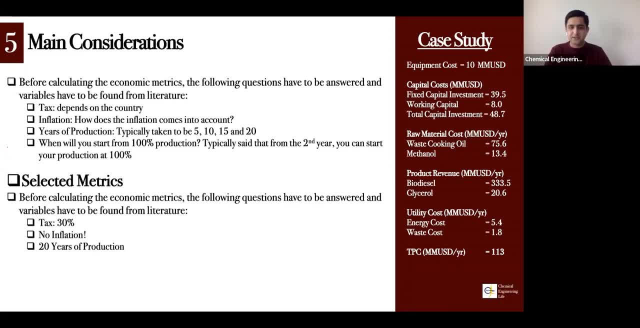 But when you are selecting the years, it's not enough that you just say, oh, I'll just select 20 years because I'm going to make more money in 20 years. Because in that way, you can also do a project for 50 years and so on. 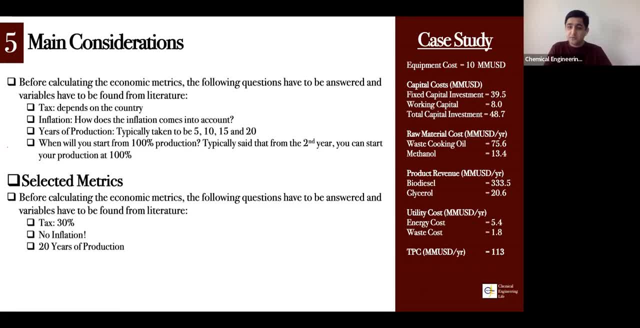 It's best to select 10 to 15 years, because the numbers, like I said, in the case of inflation, it is very difficult to assess how things will look like after 10 years, after 15 years, or after 20 years. 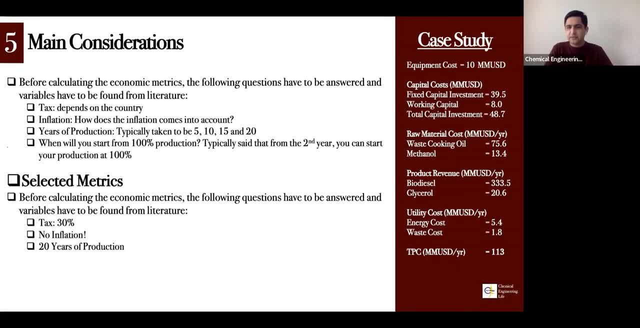 So therefore, it's a good idea to maybe always select between 10, 15, 20. 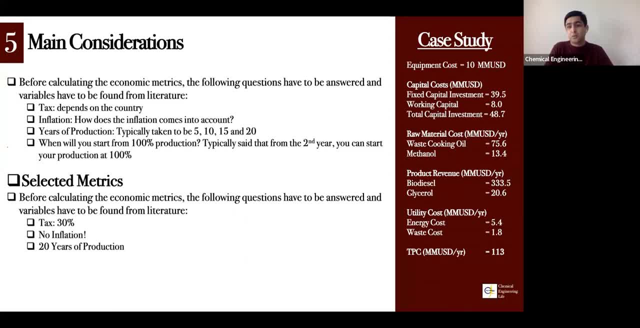 Majority of the projects that I've looked upon or worked on, they were between 15 and 20. So not even 10. So it's always 15 or 20 years. 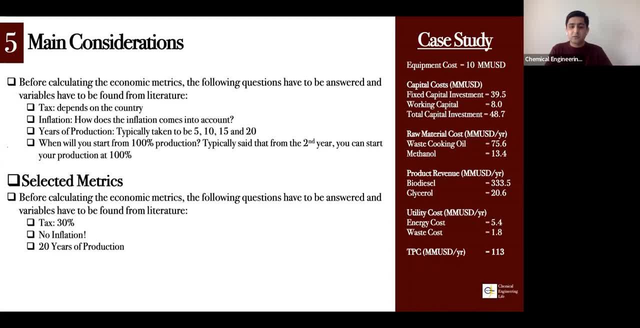 And that is an acceptable criteria for technical economic analysis. Anything more than 20 years, that's more of a stretch. And that's something that is not recommended. 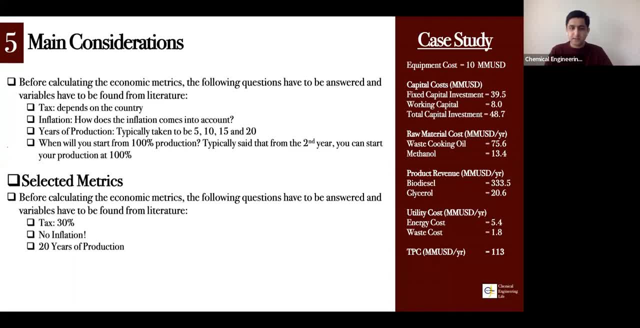 Once you have done it, then you need to select and consider about, like I said earlier, you cannot expect that already by tomorrow, you're going to have 100% production in your plant. 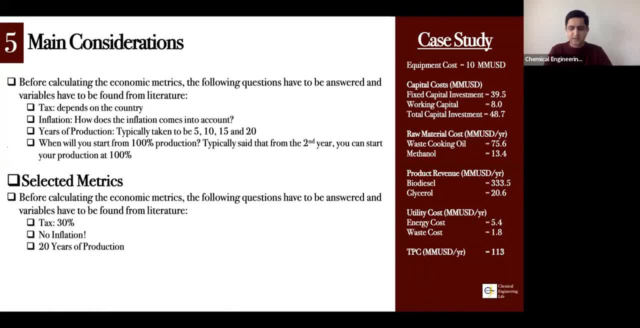 Instead, you need to identify, okay, so let's say we build my plant this year in 2022. 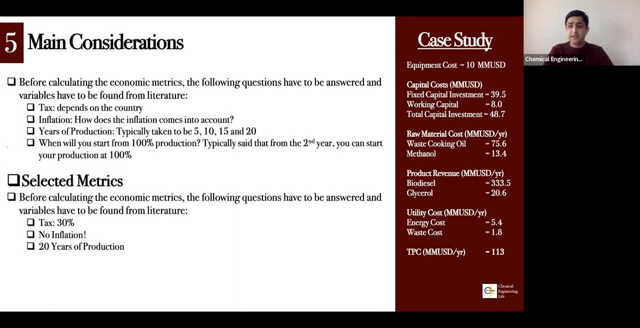 This year, we will only be hitting 50% of our production. 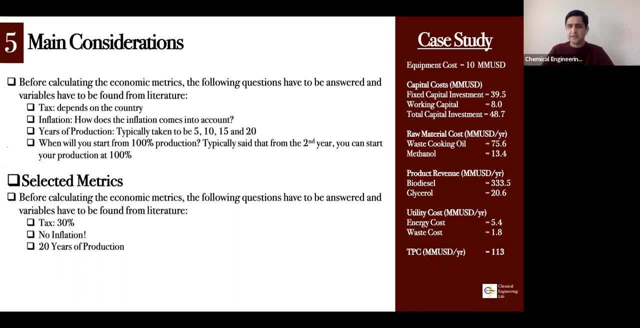 Next year, we'll try to hit 80%. 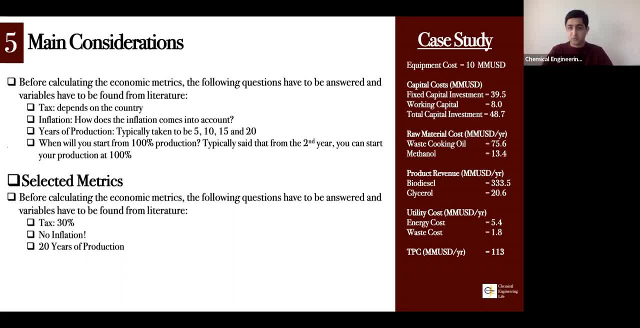 And by third year, we'll be able to reach 100%. 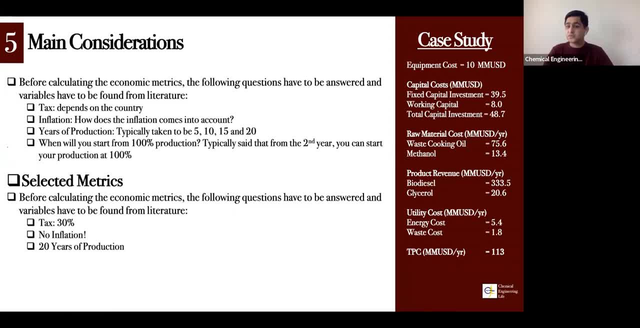 Or you could also say this year, we'll hit our 80%. Next year, from next year, we'll start with 100%. And that is why five-year project time does not make much sense, because if you were to select, 80% now and 100% next year, you have already lost one year of the profits. 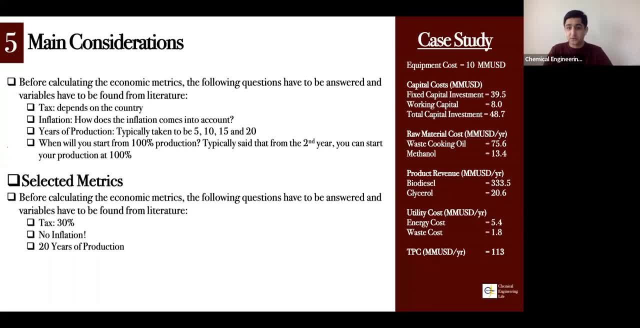 So that is something you also need to consider when you are doing the analysis. 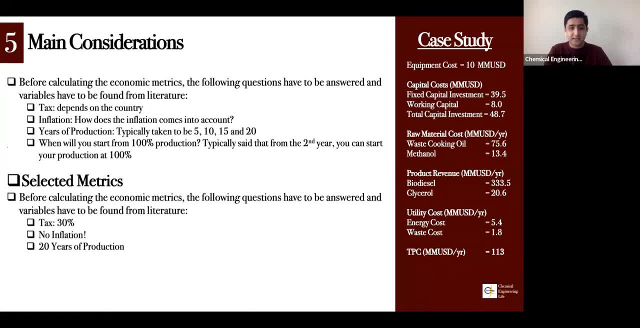 So for the purpose of this webinar, I have selected the tax to be 30%, inflation to be zero. 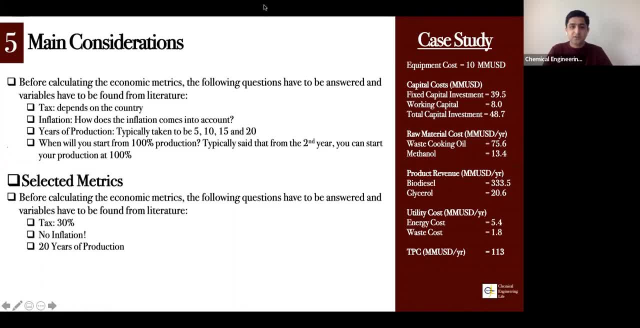 So we assume that everything that costs today is going to cost the same for the next 20 years. Okay. And so I select 20. 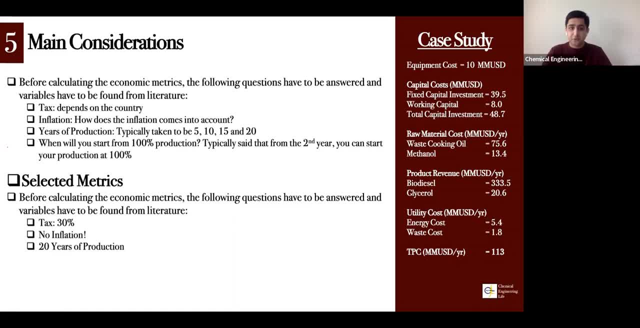 And then I said that in the first year, we are going to have 80% of our production rate. From the second year, we are going to start producing with 100%. My facility will be built in three years. So in the first year, I spend around 25% of my capital. In the second year, I'm going to invest my, 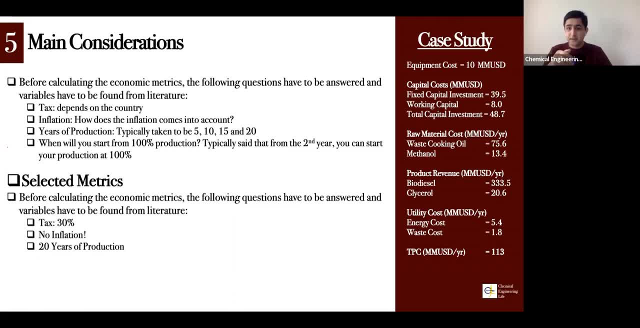 again, 30% of my investment. 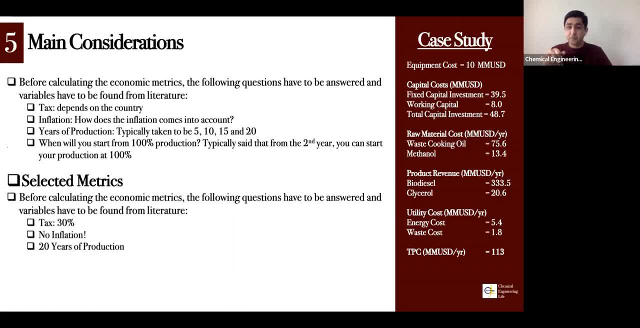 And then in the last year, we're going to invest 50% of our investment. 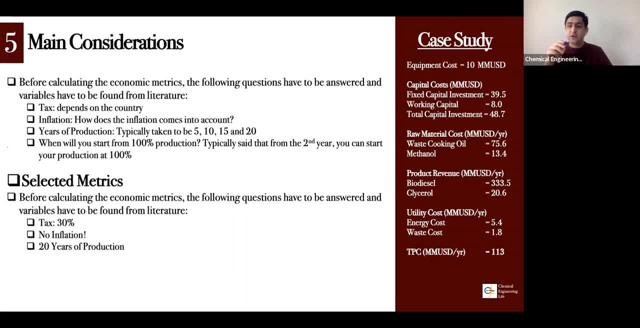 So the facility gets built in three years. We're going to have a project for 20 years with no inflation. We are going to pay a tax of 30%, no subsidy. 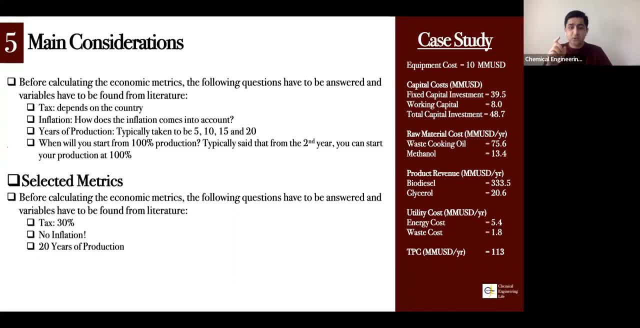 And it is only from the second year that we are going to start with our 100% production. And these are the main considerations. 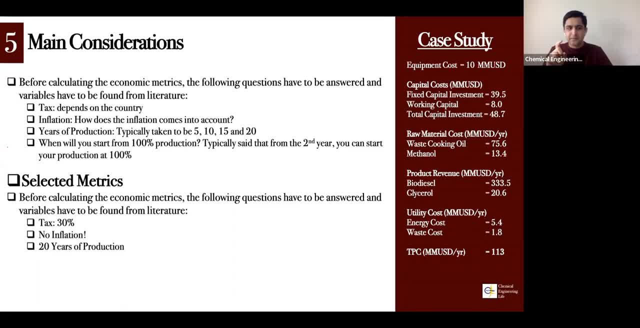 And also, lastly, the discount rate that we talked about earlier, when we had to calculate the net present value, I have selected the rate to be 11% 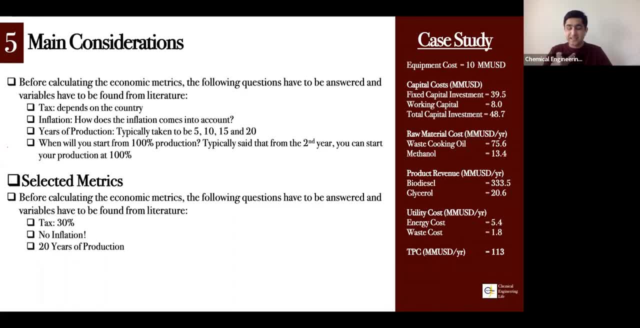 because the investment required for biodiesel is neither very low. 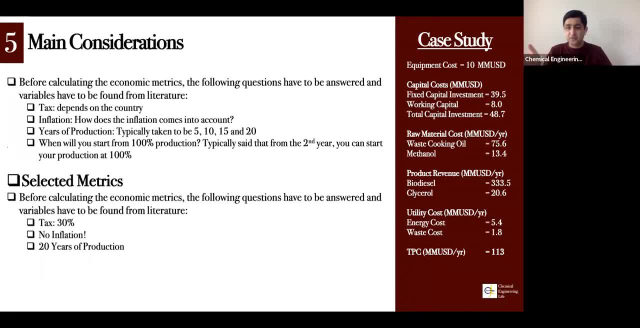 The risk is not very low because it doesn't really have a very strong market as of right now. 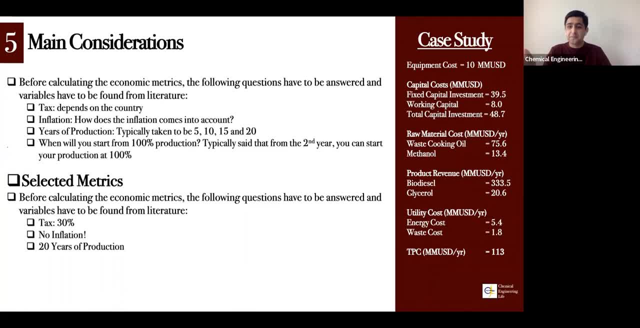 Not all of the countries are interested in biodiesel, but it is not a very high risk either 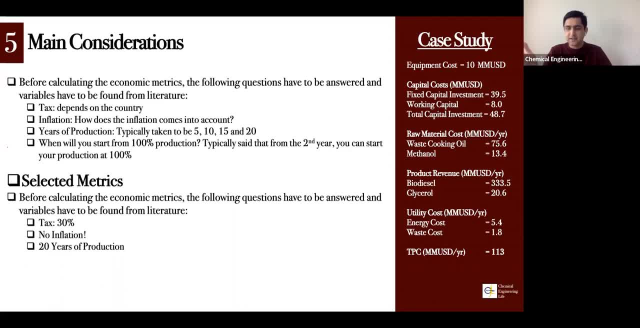 because it's not something that we can expect in the coming years due to climate change and environmental challenges that more and more countries, especially EU and the American government, they are moving towards using biodiesel. 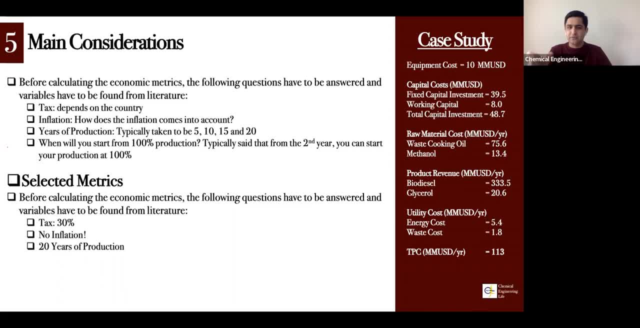 So that's why I have selected 11%, which kind of falls right in the middle of, in the category of median. 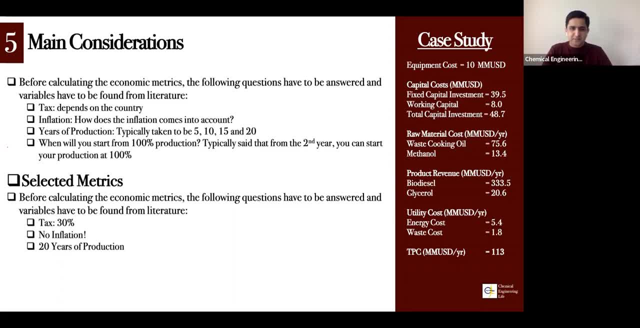 So the next step is then to convert all this data into a calculation and I strongly suggest that you do it in Excel. It is very easy to do it in Excel and it's very easy to keep track of all the calculations when you're doing it in Excel. 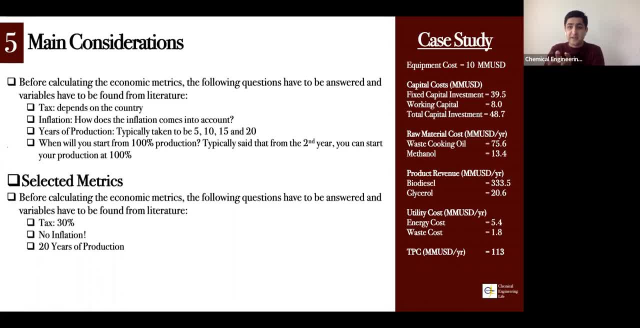 I have myself, I have done it in MATLAB as well. 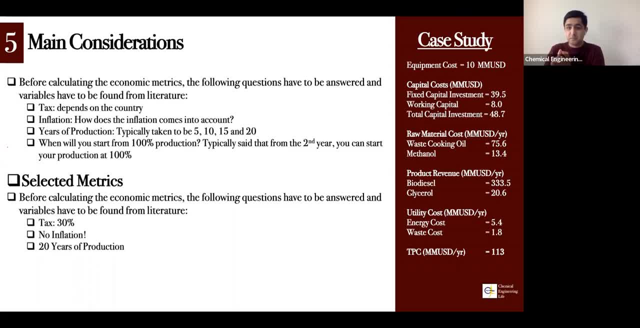 I have met a lot of people that tend to do it in Python or in MATLAB, 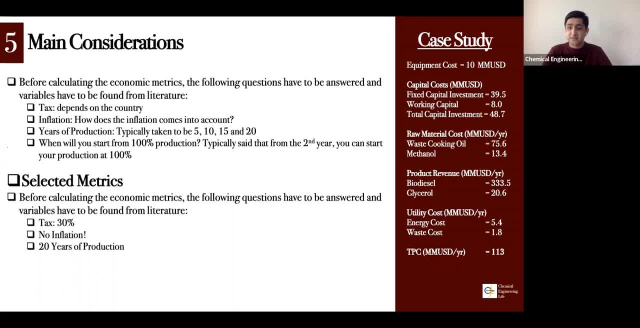 but in my opinion, in my experience, the best way to do it is in Excel. 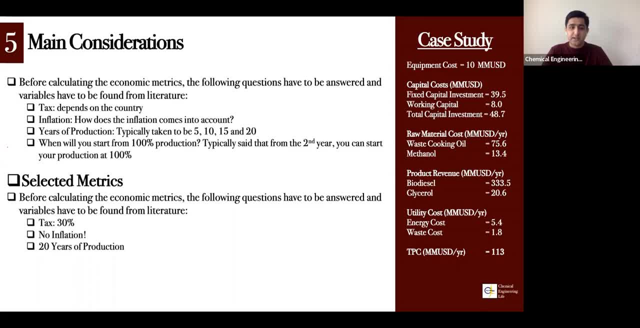 And the way to do it in Excel is that you create a calculation and you create one column, you call them column A, with all of your costs. 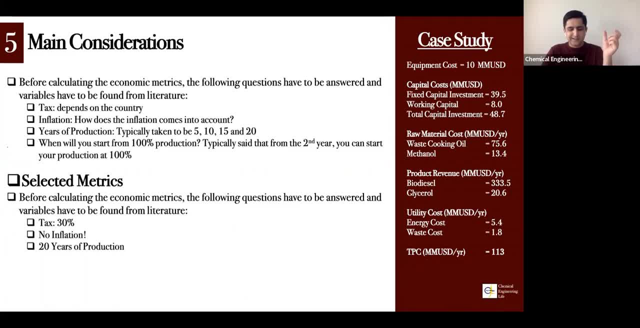 You could say like, what do you call it, like the TPC, your income, profit, tax, and so on. 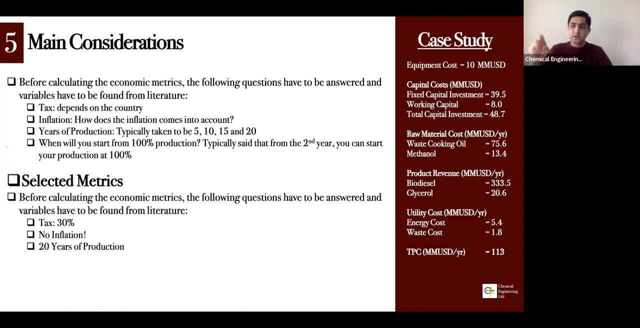 And then you make one column for each year. So you have year one, year two, year three, year four, up until year 20. 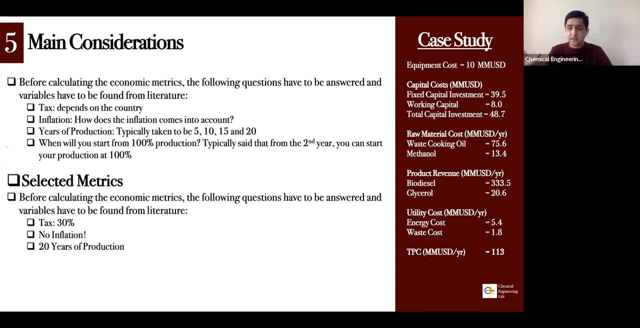 And for each year, you calculate how much money you make, how much money is paid off in expenses, into your TPC, how much money you are going to be paying off in taxes, how much money will be paid off or will be taken in from depreciation. And depreciation is also taken into account when you're doing the technical economic analysis. 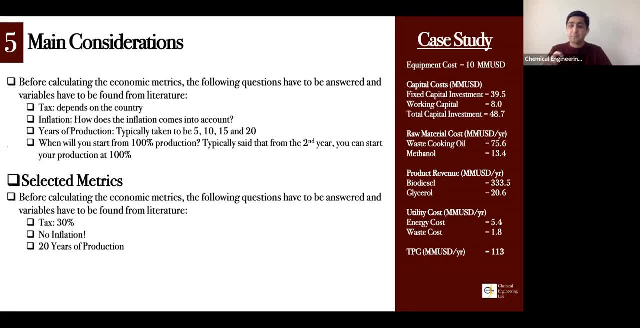 And then finally, how much money did you actually end up making from per year? The reason I'm saying per year 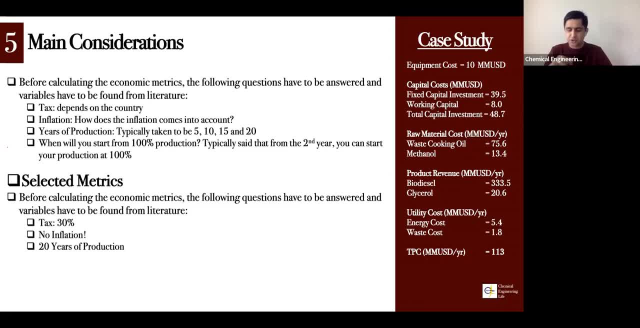 is because many of the metrics that I'll show you now, 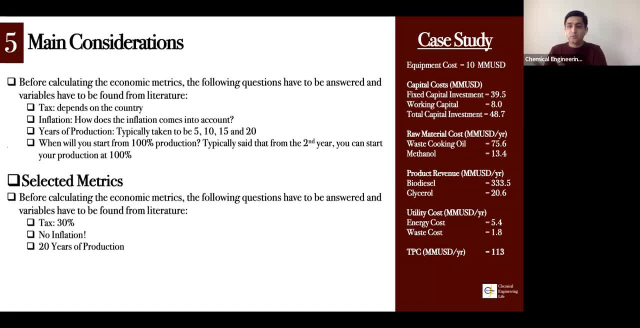 they are dependent on annual, annual basis. 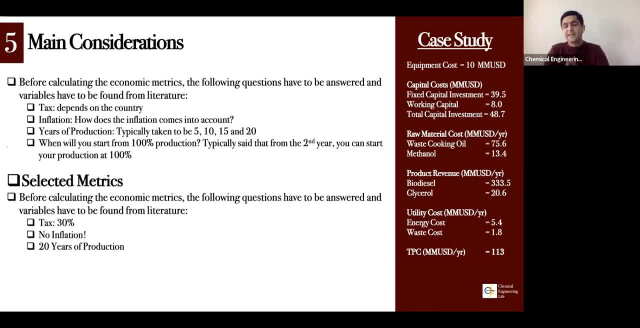 So if you have the numbers lying around for per year, it just makes it a lot easier for you able to calculate them later on. 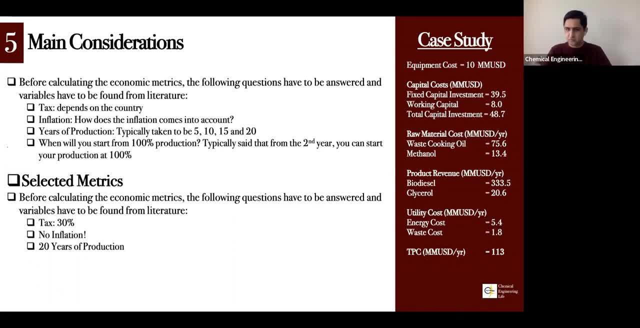 And then of course, you can always sum them up in a cumulative sum or so on. 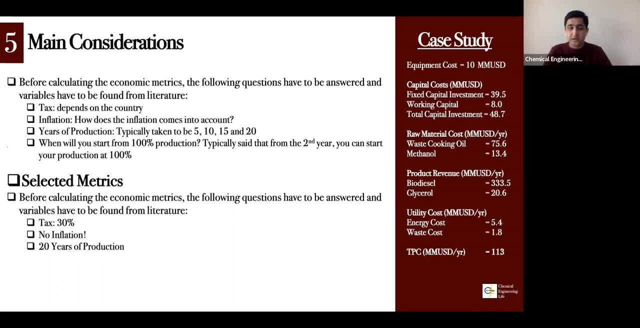 So in that way, it's always best way to do it is in Excel. 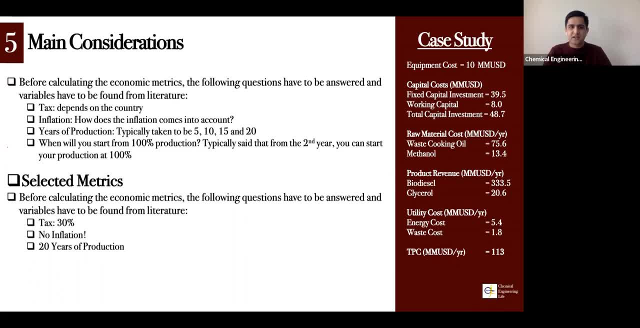 And I can't stress that enough that it makes your life a lot easier when you're doing it in Excel. 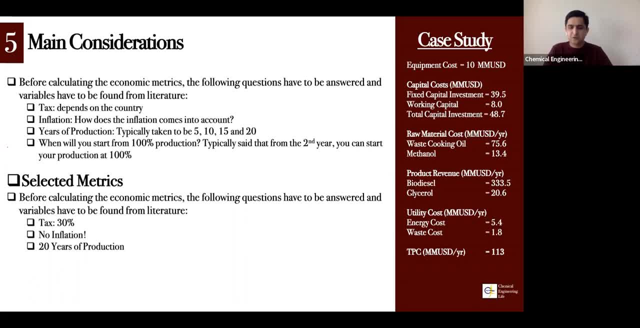 And just a quick suggestion, when you're building up your file, 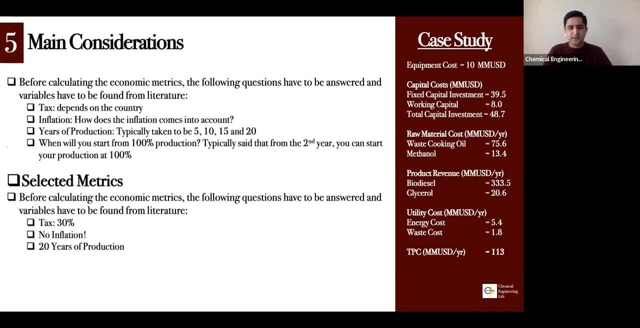 in Excel, it is just a good practice of doing it is that you create one tab with all of your variables, all the input variables. 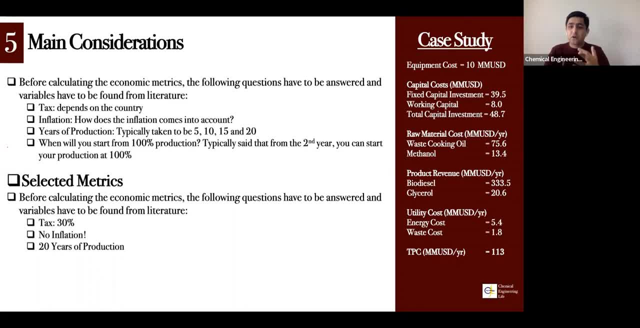 That means your raw material balance, raw materials cost, your product materials, your cost, utility requirement, the cost, the sum, the variables that we have selected here, inflation, tax, and so on. 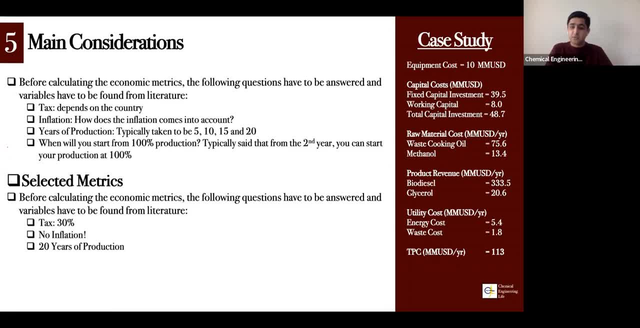 I have seen a lot of people, they make multiple sheets and then you need to go in into each individual sheet to change a number. And that is just very difficult to manage 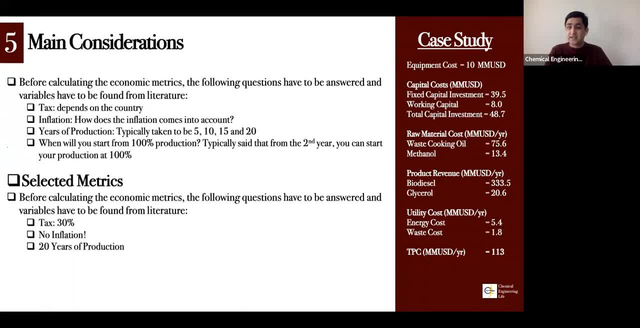 and very prone to mistakes and errors. 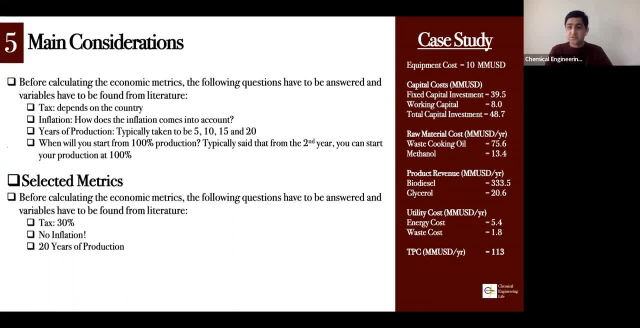 Therefore, the best way to do it and the best way I would suggest you to do it and the way I do it is that you go in and you create one sheet with all the numbers, all the variables that you need. 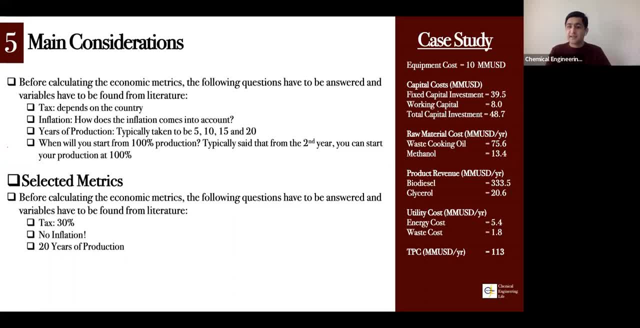 And then you make a second sheet with all of your economic analysis or economic modeling. And economic modeling 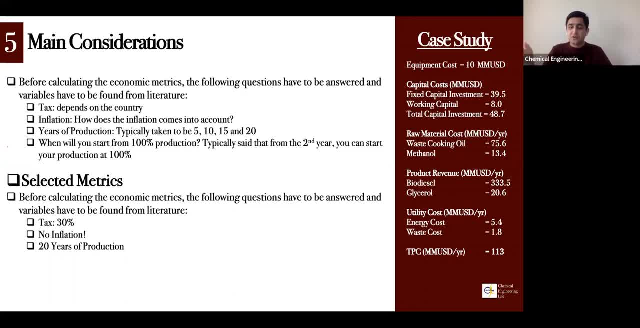 is of course where you make one column for one year, for each year. And then in the rows, you write your variables. 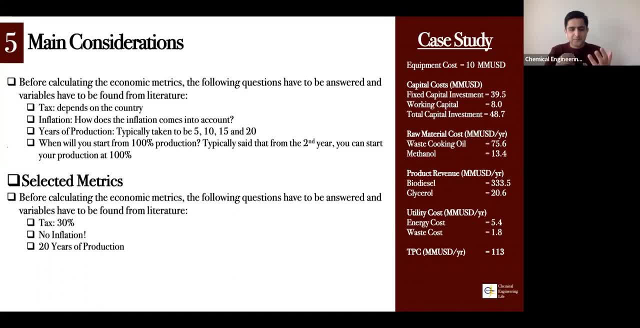 And the variables, they are, like I said earlier, you need to remember for your income that you're producing and that depending on how much production rate you have, it is 80%. 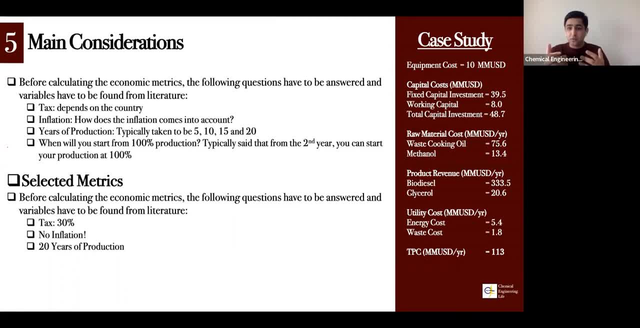 Then you're only going to be selling 80% of your annual product. 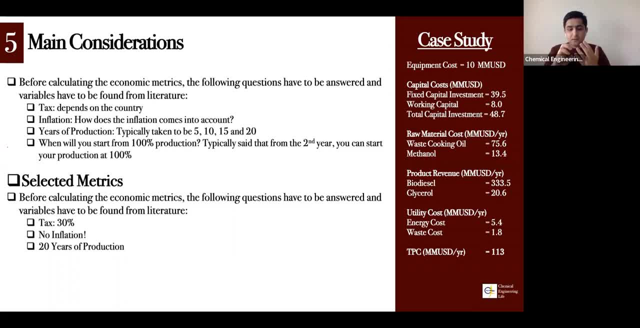 But, so your annual income, then you need to have a row for how much money, how much expenses you have paid. That is your TPC. So then you do your annual income minus TPC. Then you would have one row with how much money you have left. Then you need to pay off taxes. Tax will be taken away from that money as well. Actually, sorry, it's the other way around. So when you have your income, the first thing you do, you pay tax. And then from the tax amount, then you pay off taxes. 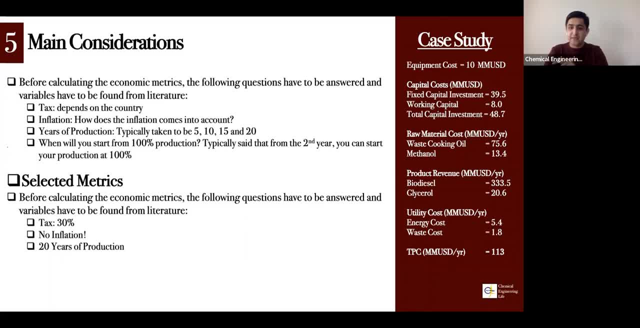 Then you pay off your expenses. Then the money that you have paid for your expenses, that money is your profit. That is the money that you can then keep in your pocket. 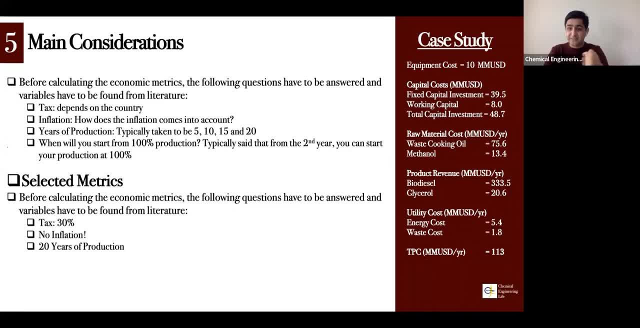 If you have investment, then you need to pay off your investment from that money. 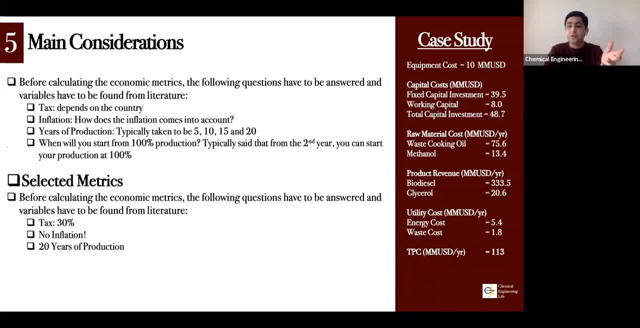 If you cover, if you pay off your investment in the first two years, 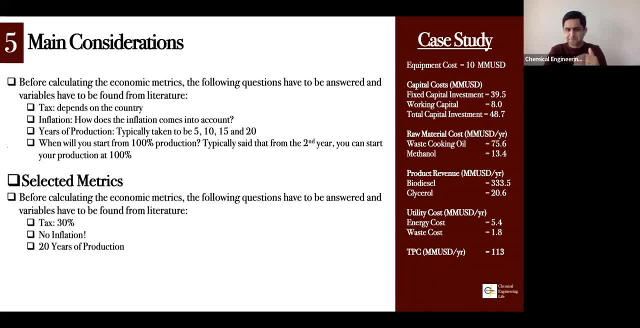 then after two years, all that money would go straight into your pocket. 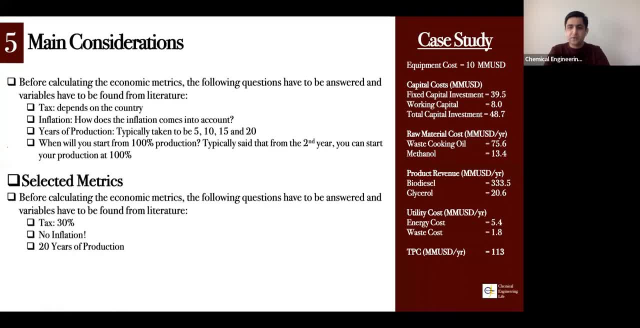 Once you have done that, then you move down and then you can calculate the cumulative sum of all of your profit. Because the profit is the thing that is going directly in your bank account. 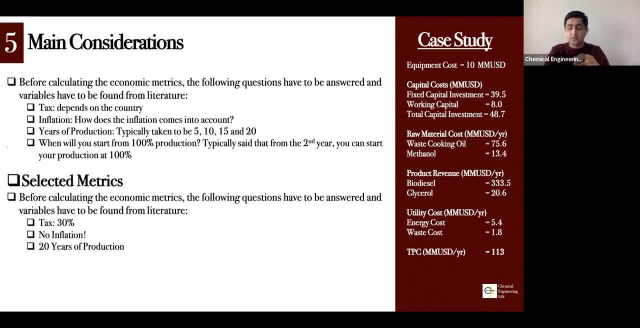 So that's the money that you don't need to calculate or subtract any longer. 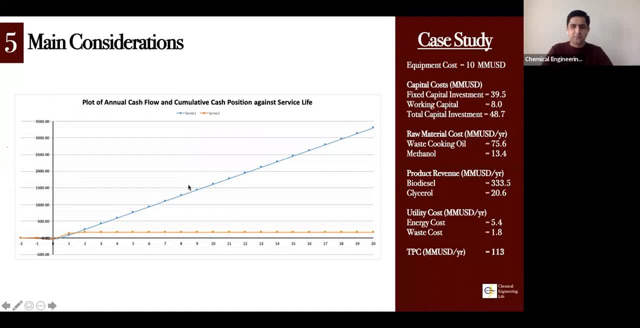 So the more money you add up, and I'll show you in our next slide right here. 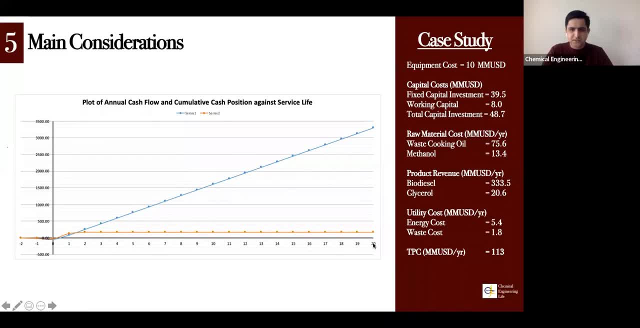 So this orange line right here, so you can see, I have done the exact same approach, the one that I described here. I'm not going to go deeper into the individual formulas because for the purpose of this webinar, the idea is more to have a look at the general methodology and the results. 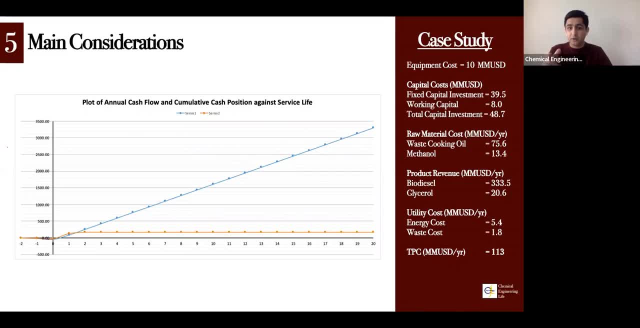 But I will share this slide with you all after the webinar, and then you all can go in and also look at the formulas if you wish. 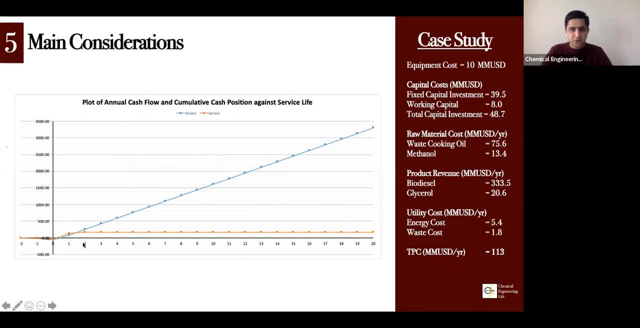 But if you look at this graph here, so we did it for 20 years that I calculated the amount of money that I'm generating per year. 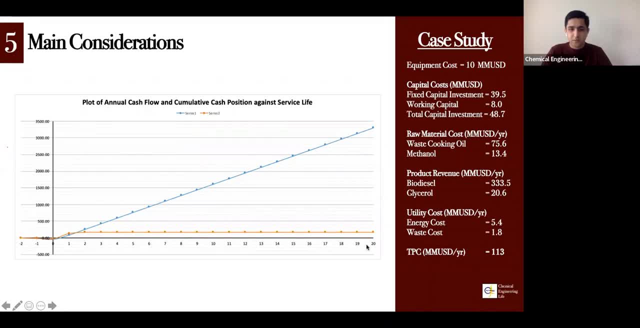 So you can see for the first year, second year upon the 20, it took me three years to build my plant. Therefore I have my minus two, minus one and zero. 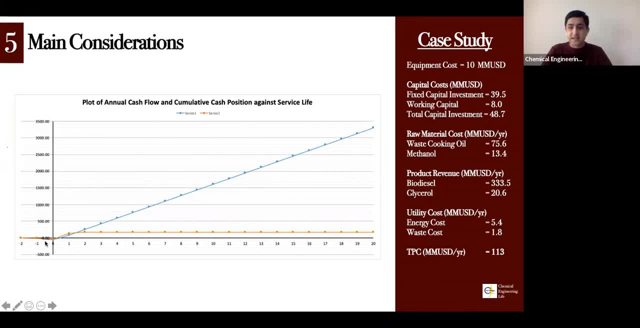 And there you can see the money is going down because that's where we are using our investments. 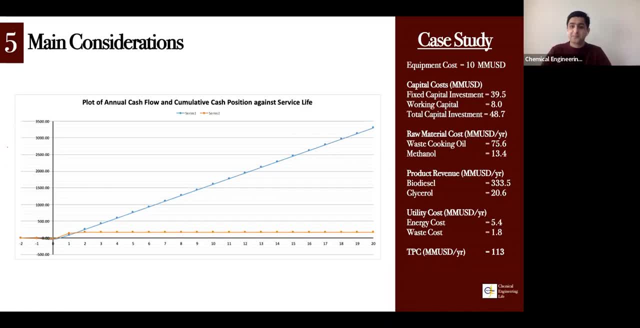 So that's negative, right? If I'm investing, like you can see right here on the slide, our investment was 48 million and all of that 48 million gets used up in this area. And therefore the line is going downwards because, you know, it's negative. 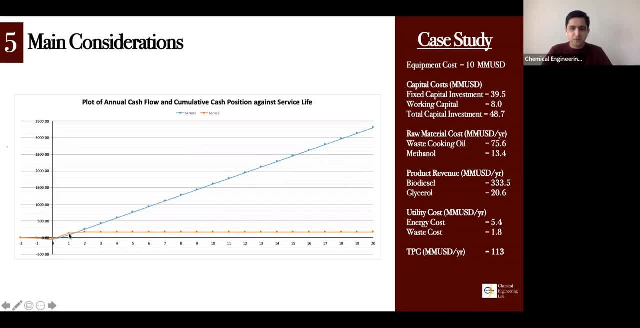 So right here, you can see this one is slightly below because here in the first year, we only have 80% production. From the second year, that's when we hit it off 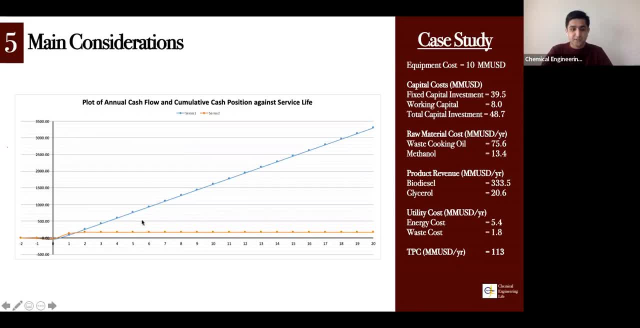 with 100% production. And therefore you can see the graph goes down and slightly curve and then becomes a line. 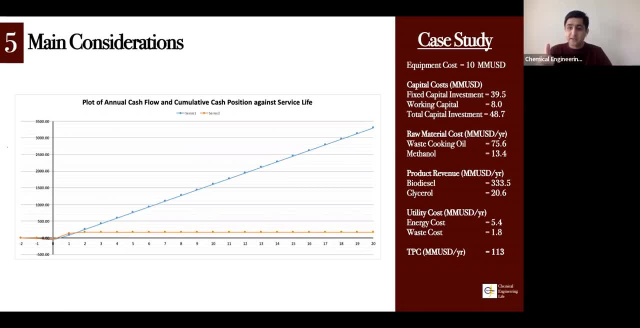 It may look like that we are making profit, but please remember, I have not taken inflation into account. 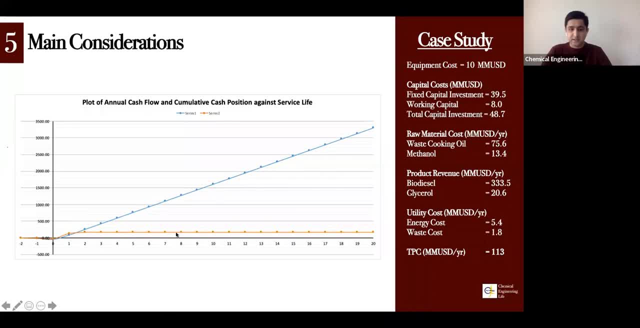 So therefore, if I had taken inflation into account, this line, it is actually my annual profit 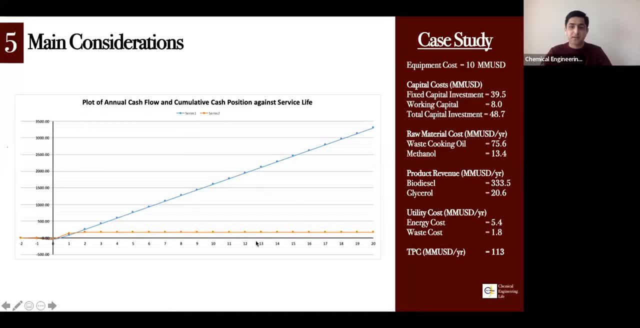 that I am getting in my pocket. So this is around $169 million per year. 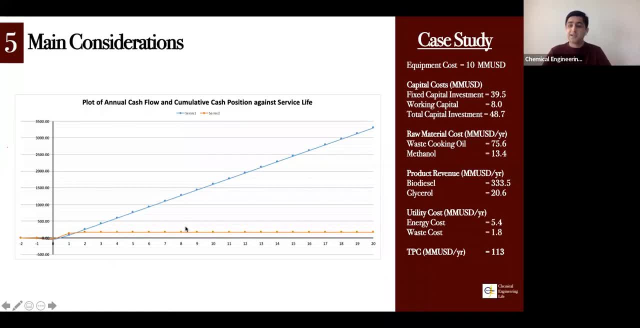 So that means after paying off all the expenses, my taxes, my TPC, everything, I get $169 million in my pocket. 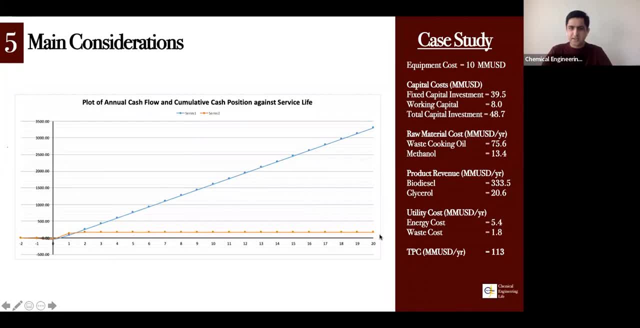 And that is this curve. And you can see it is a straight curve. The reason is because we are not taking inflation into account. 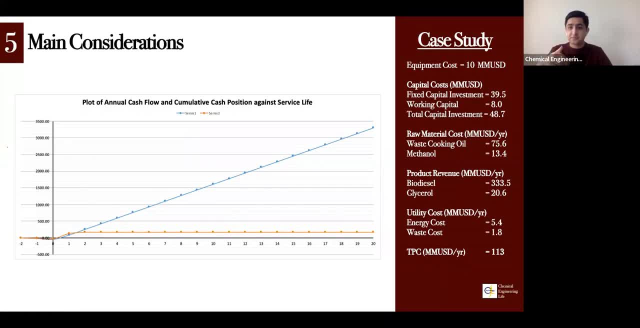 So the money, the things that I am selling today are going to cost the same next month. Therefore, it's the same. 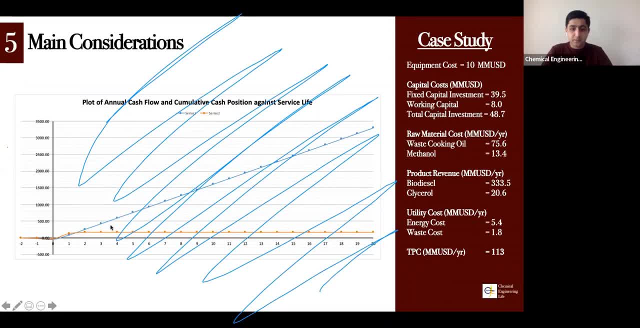 On the other hand, this line there, the blue line, it is my cumulative sum. 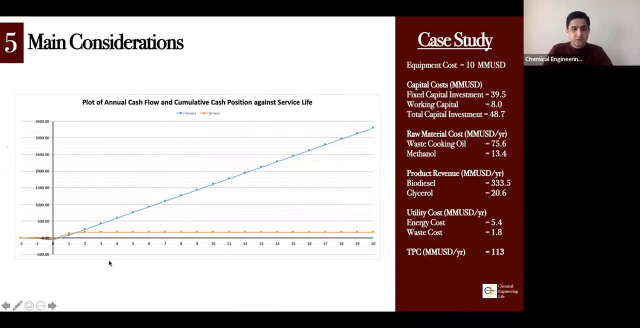 And the cumulative sum is like, so the cumulative sum is basically like if I made $169 million in my first year, $169 in the second year, we add them together. In the third year, I made $169 again. So I add all three of them again. And likewise, you do it for all the years, all the consecutive years. 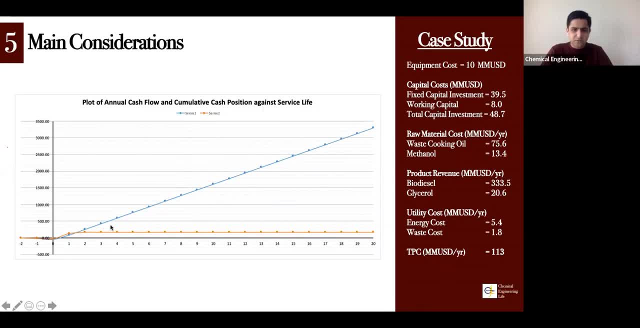 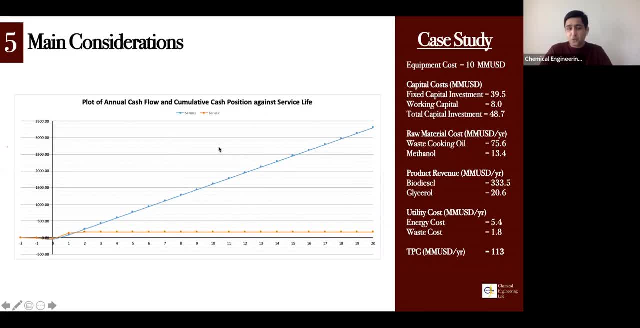 And yep, and this is a good idea to always plot this graph because already from this graph, you can take away a lot of considerations that you have taken into account. 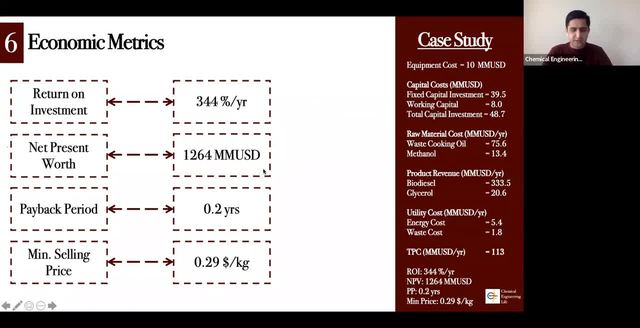 So then once we have done all of that, we can then move on and calculate our economic metrics. 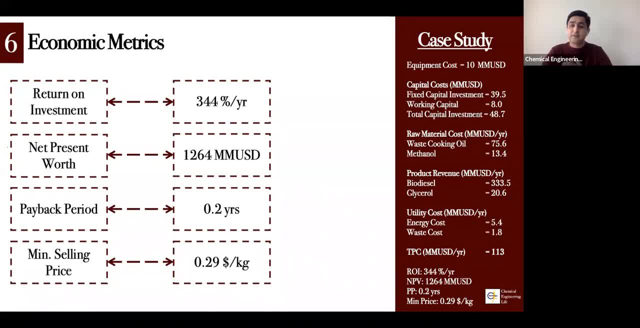 The economic metrics, the first metric that we have done, that is the return on investment. It is my profit divided by all of my investment. It turned out to be 344% per year. That means that my profit, because my profit per year, that was $169 million. 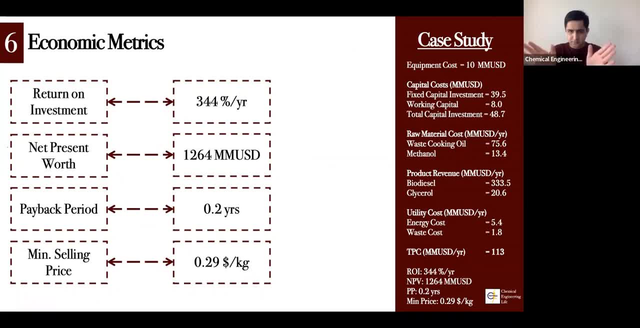 Million dollars per year. That's to say $170 million per year, just for the even number, even in half. 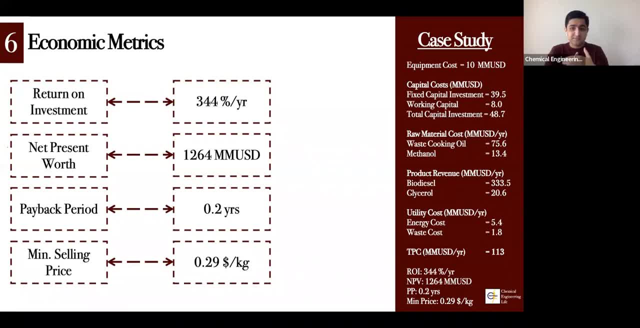 My investment was only $50 million. So you can already see right there, compared to that, it is 300% our profits 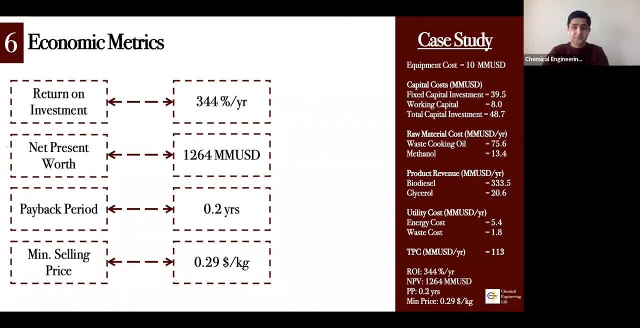 or 300% more than my investment. 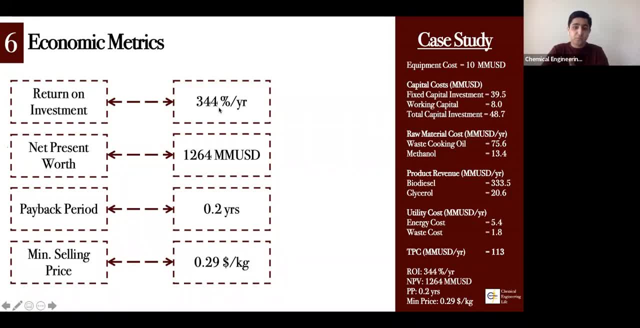 That is what this number means. And this is an average number. 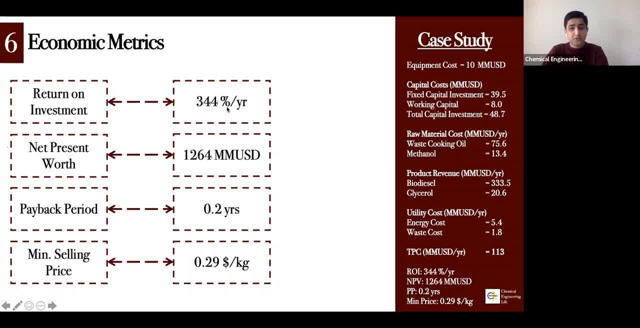 So that means annually per year, for 20 years, my profits, 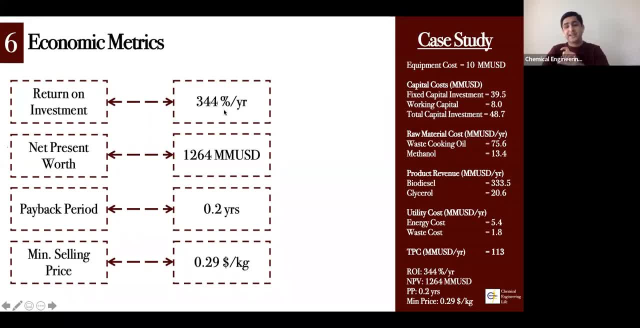 were 344% of my capital investment. 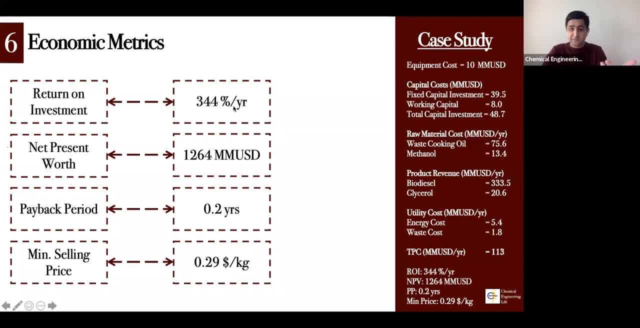 If you give that number to your investor, they're going to be very happy because that means that the money that they're going to be investing, they're going to be getting 300% more out of the business. So that's a great thing. And that is something that 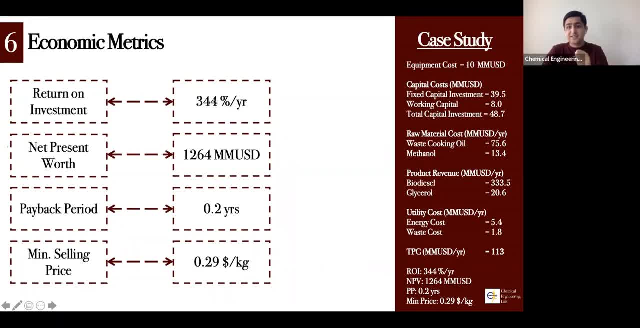 this should be more than a discount rate. So we selected the discount rate to be 11%. This is 344%. 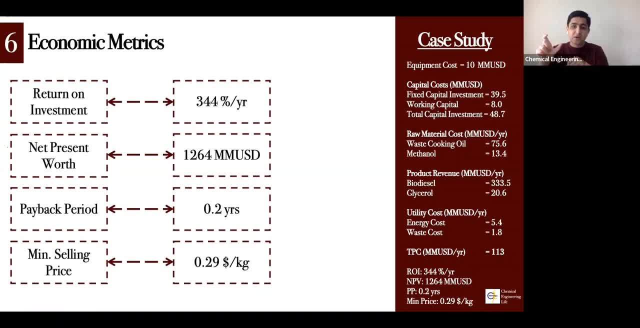 So if it's higher than discount rate, that means that this number or this metric is profitable. The second one that we have is called the net present worth. 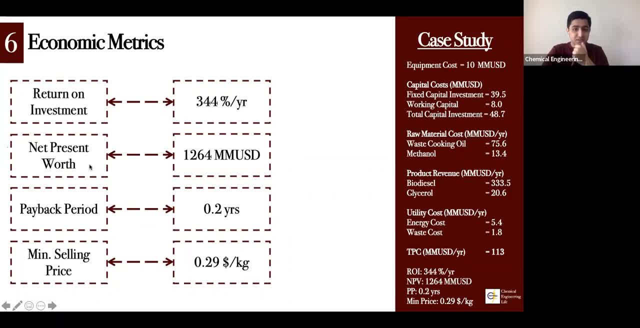 And the net present worth that I said earlier, it tells us how much, like how the value of money is going to change with each year. 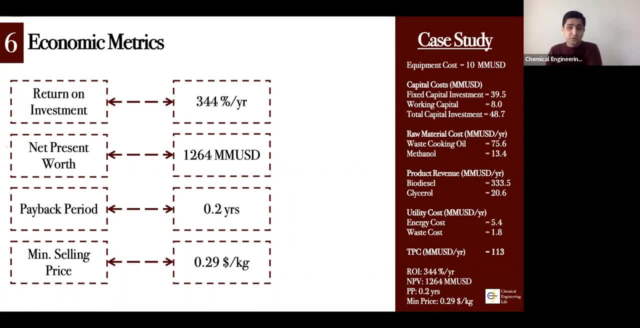 Like how much we will be worth after 20 years. And that is going to be, it's going to be $1,264 million after 20 years. 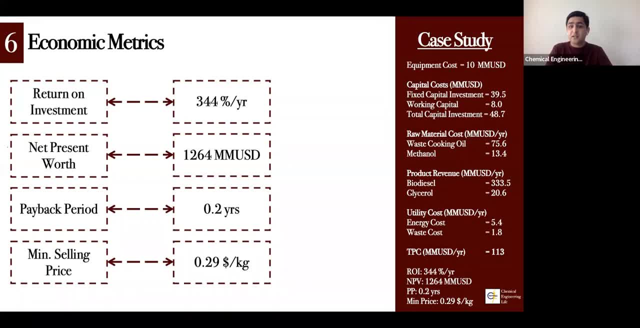 That means that after 20 years, we are going to be worth, the value, the time value of the money will be around $1,264 million, which again itself is a great investment. 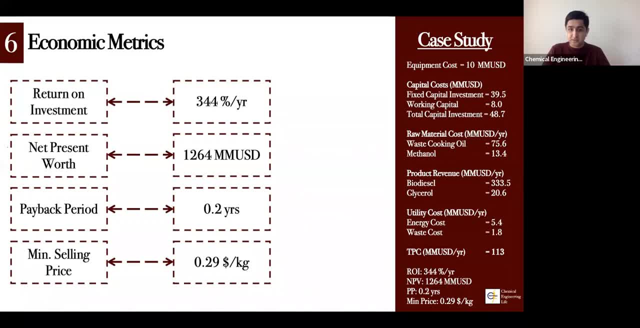 That means that in 20 years time, the project is not going to depreciate. It's not going to go down in value. 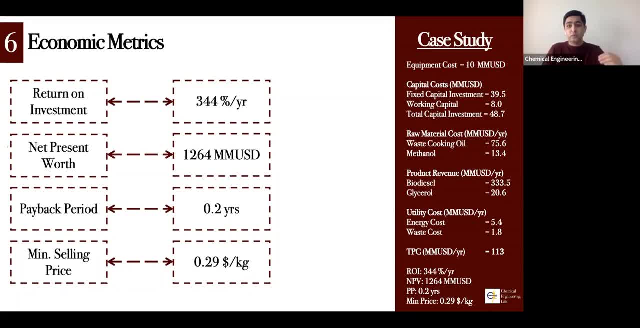 But instead, we are going to be worth a lot more than what we started off with. 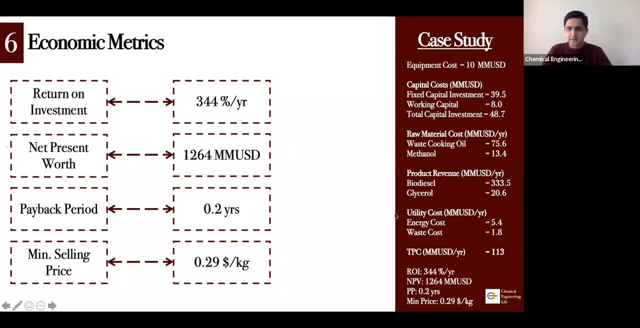 And of course we have our payback period. And the payback period, if you look at the metrics that we have on the right, 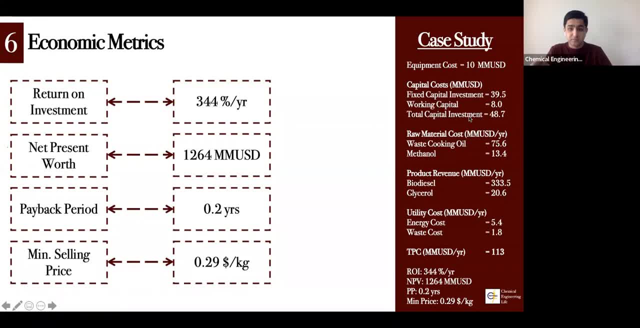 you can see that the investment was only $50 million, right? The total investment, the total loan that we got was $50 million. 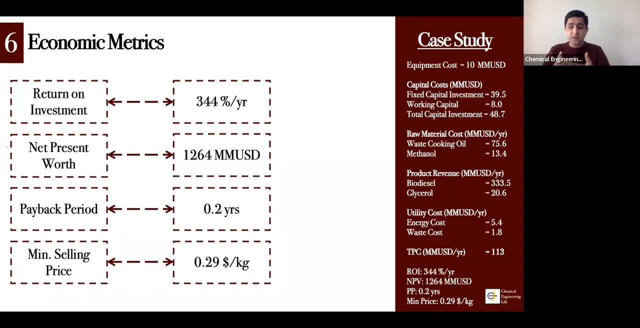 Our profit per year, it is around, like if you look right here, the products that we are selling, 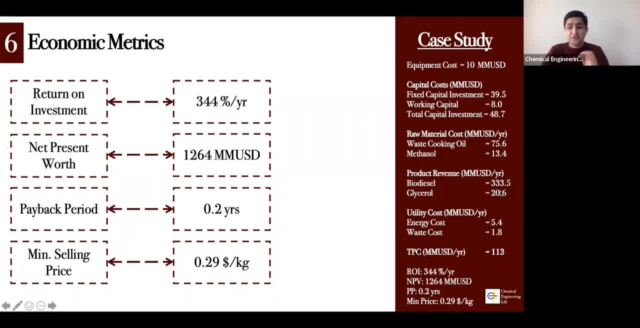 they are, they are bringing in $354 million per year. 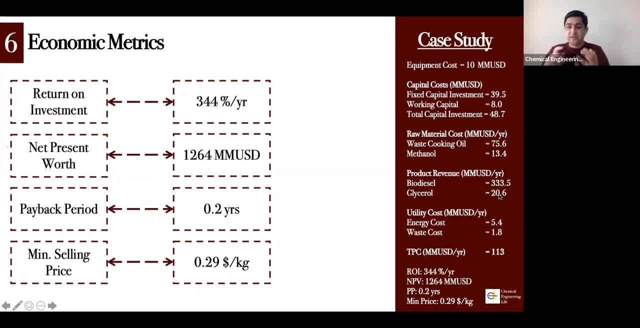 That means that we do have a great deal of money left behind. Even if I pay my taxes, if I pay my PPC, I still have around close to $200 million left around. 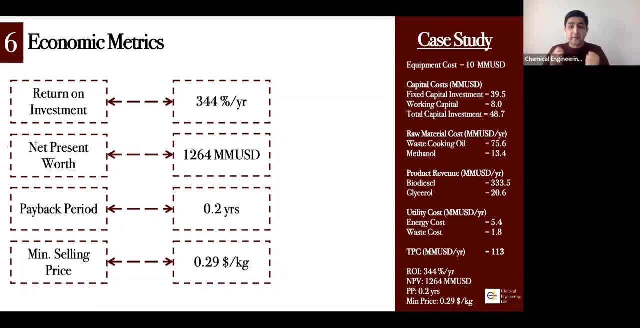 And that is why it is possible for me to pay off my loan within 0.2 years. 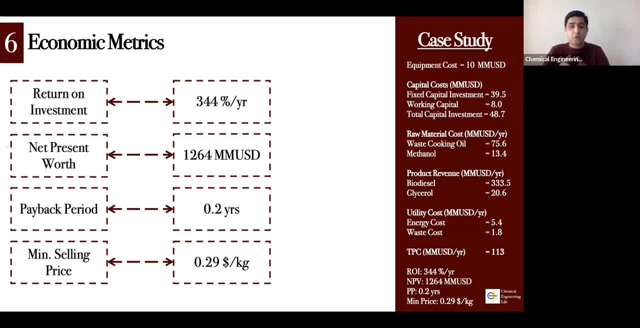 That means in 0.2 years, I'll be able to pay off all of my capital investments. 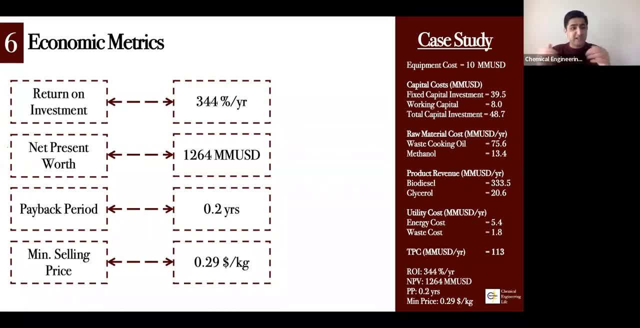 All of my investors, they will be paid off. All of the bank loans, they will be, that will be paid off. 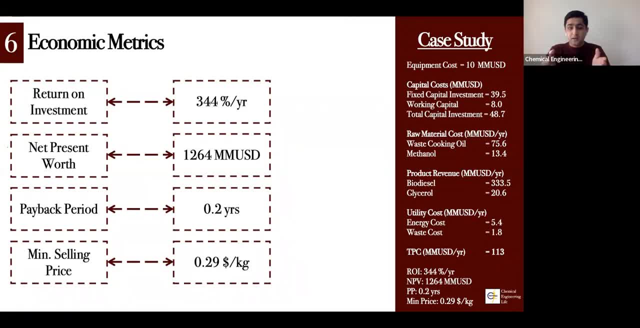 And I can start putting all that profit into my own pocket. The reason it is very low right now is because as you can see on the right, 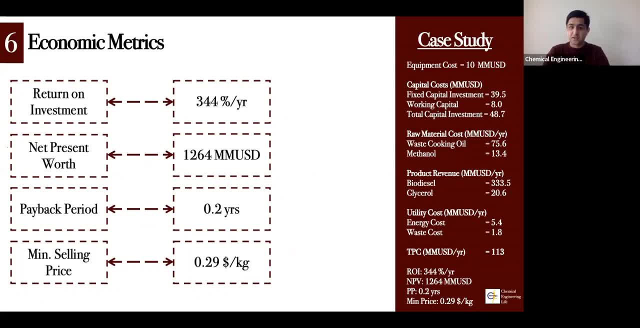 it's because we are making a great deal of money from sales. 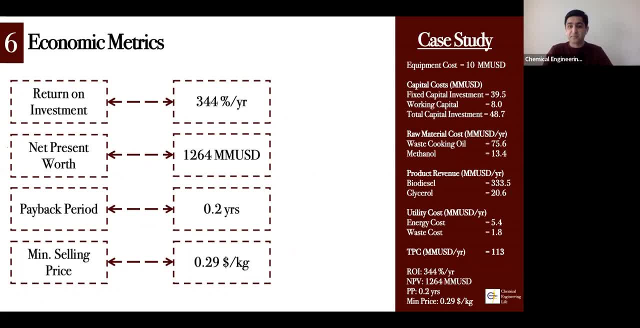 Sometimes I have worked on a project where the payback period is eight years. And if it is eight years, 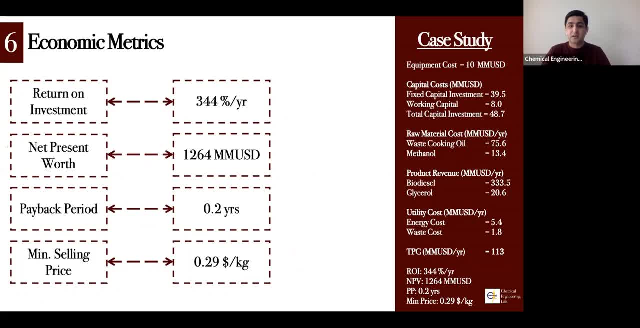 then it's not very acceptable because that means that you're not going to be making that, you will not be able to pay off your investors in a good amount of time. 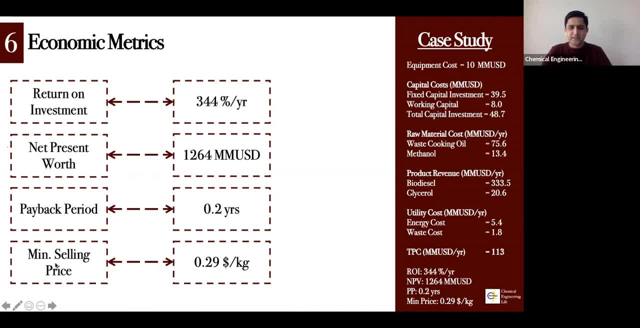 Finally, the minimum selling price, that is the price that we need to be selling our product, which is biodiesel. 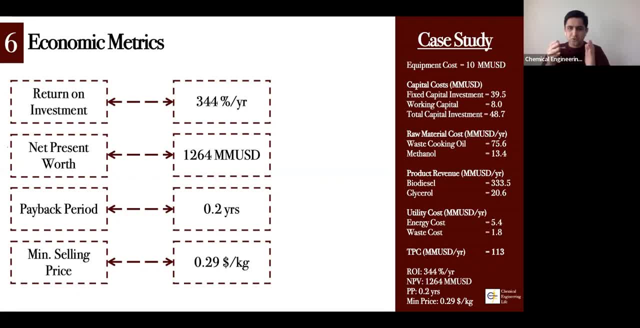 That means that in order for us to create a profit, we need to sell biodiesel at a minimum price of $0.29 per kilo. 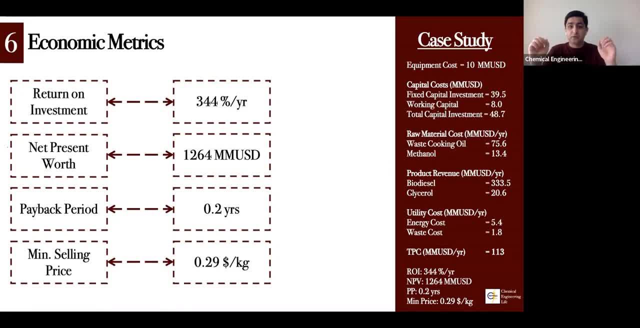 If somehow there is a market crash, somehow there is all of a sudden, too much biodiesel in the world, and the prices plummet, they cannot go below $0.29 per kilo. 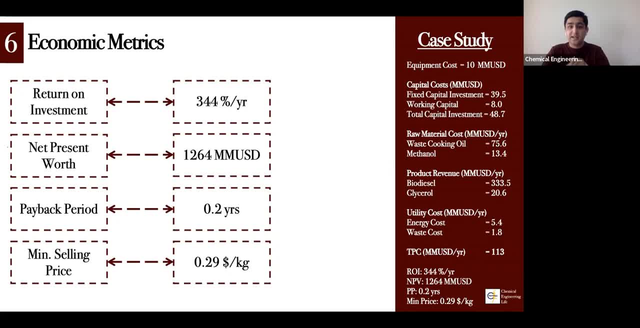 If they do go below $0.29 per kilo, that means that we will not be able to make a profit. 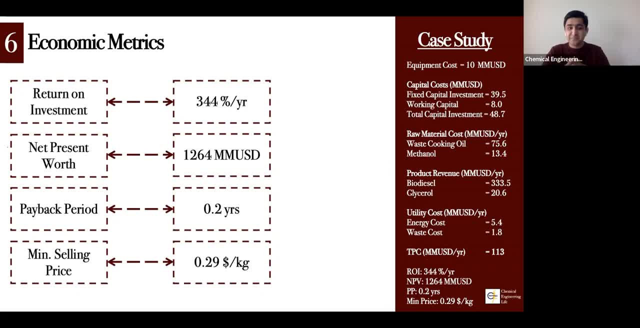 And that is what essentially the minimum selling price is. 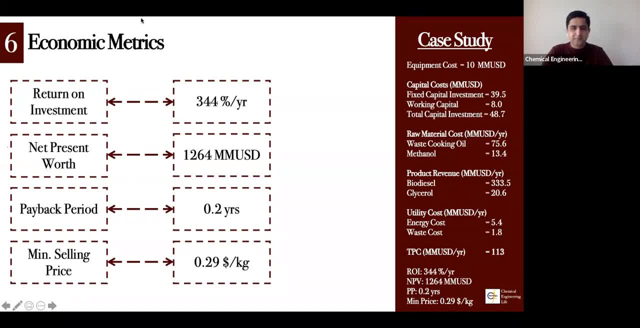 And if I just go back, I can show it to you right here. 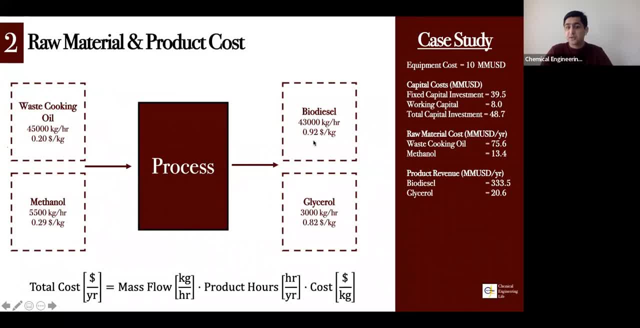 The price of biodiesel that we have selected is actually $0.29 per kilo. So already there, 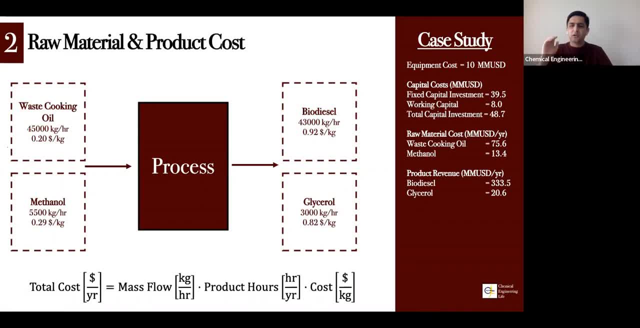 you can make an assessment and say that it would take a lot, a lot of uncertainty or a market crash to bring biodiesel down to $0.29. 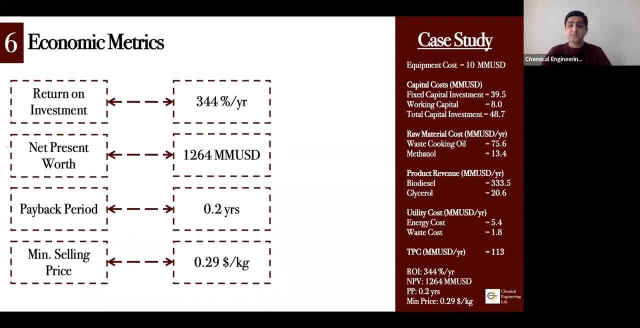 So in that way, you can always argue that our process is indeed very robust and profitable 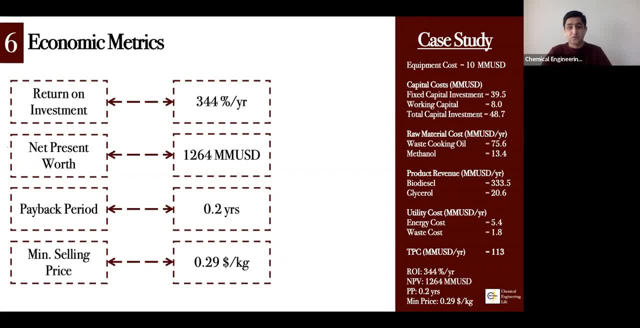 because we are in a very, very safe zone in terms of the minimum selling price. Now, 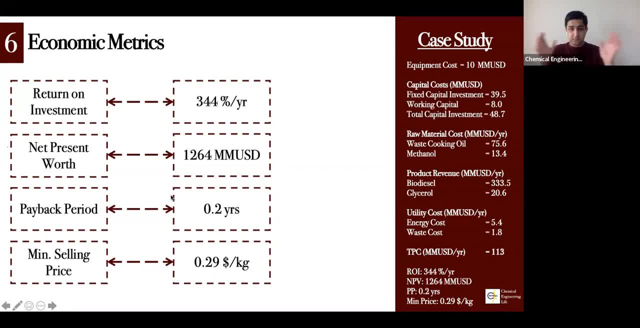 if you look at all of these metrics, if you take a general overview and a general assessment, we can conclude that our process, our biodiesel production is indeed a very profitable process. 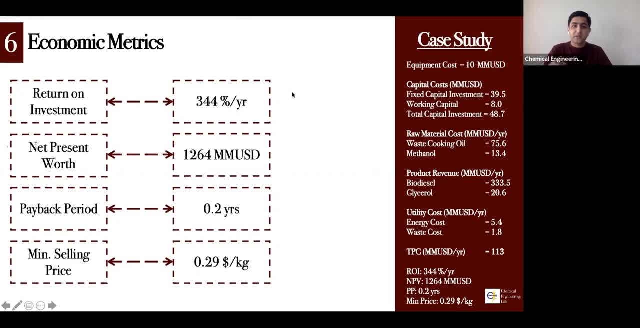 It is very profitable. The reason being that they all metrics, they agree with each other. 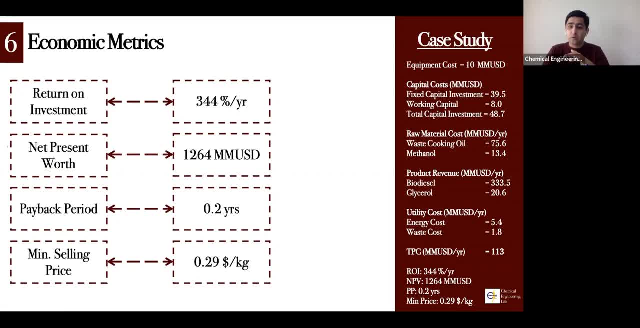 And our investment is, we are getting more and more compared to our investment. Our time value increases, increases all the way up onto 1264. We are going to be, we're going to be able to pay back our loan within 0.2 years. 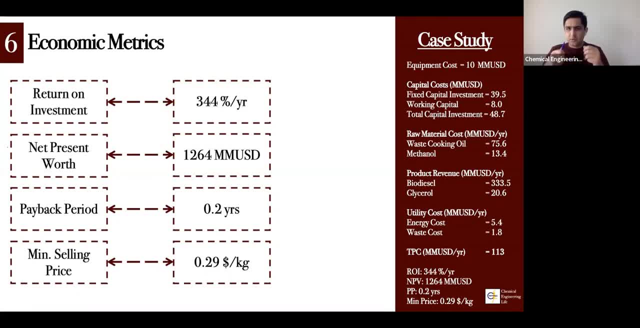 And the minimum selling price is way below our current selling price. So in that way, we can conclude that, you know, biodiesel production is profitable and whoever wishes to do it, 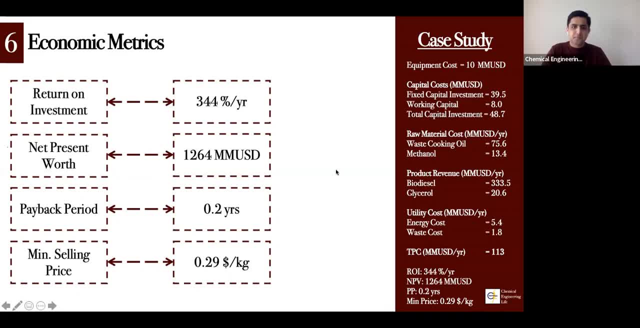 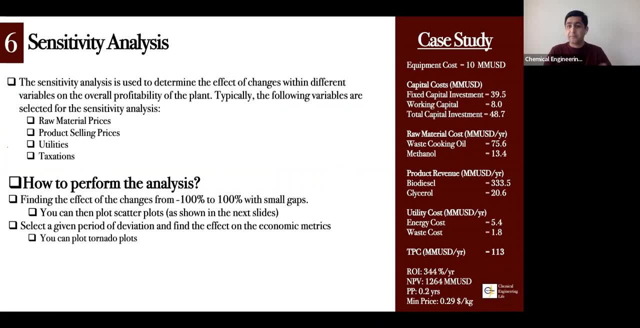 they're going to be making a great deal of money out of it. But the thing is that the calculations that we have done so far, they are all theoretical. They're all based on literature. They're based on sources. They're based on, 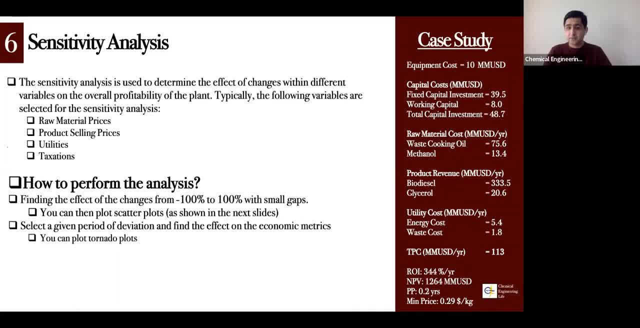 on different relations that we have found from different areas. 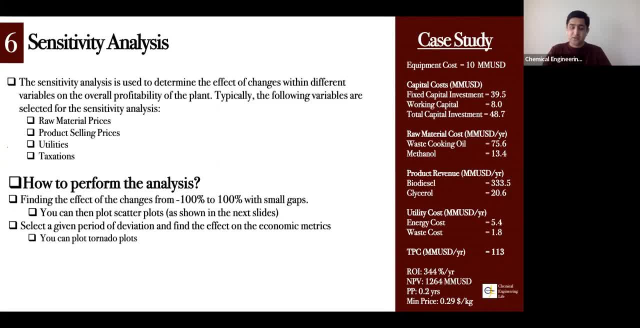 In reality, you have to be able to understand, you have to be, you have to be able to assess, you have to, and you have to understand as an engineer that these things can change. 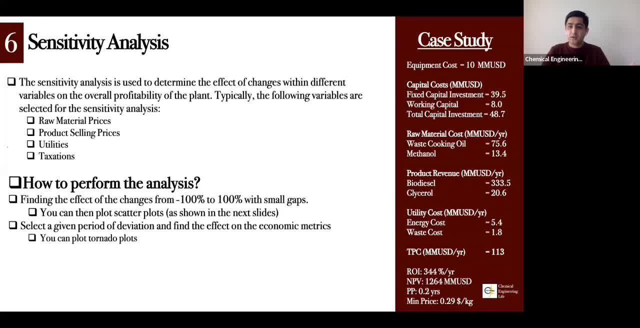 There is one thing doing the engineering legwork that, that is not affected. 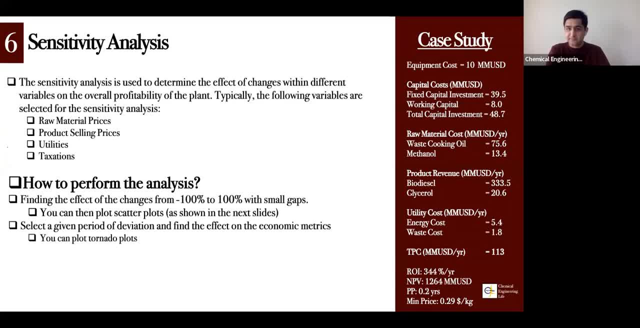 That is only under the command of an engineer. You know, you go in and you can change the variables as you like. The pressure, the temperature, they're not dependent on the outside world. 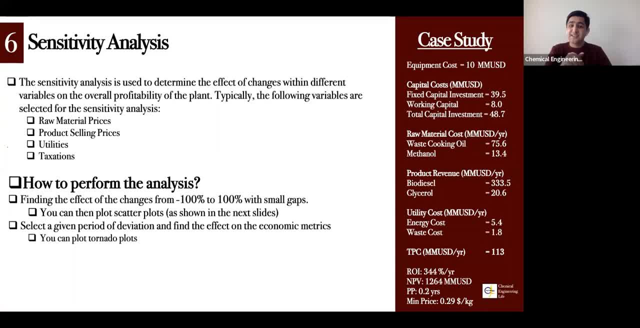 But the techno-economic analysis is something that is directly linked up with forces that we can't control. 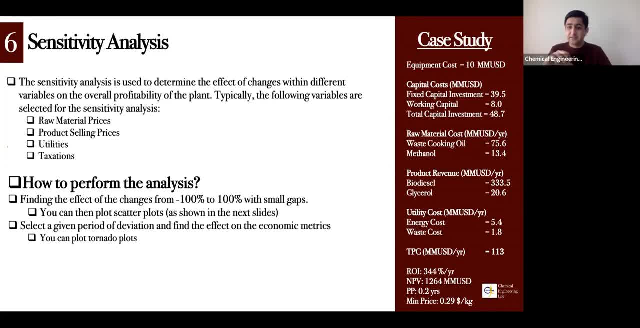 This entire process is dependent on something that is out of our control. The international market, the political stability of your country, the, you know, for example, when we saw the COVID crisis, for example, it came up, the prices, the market crashed. 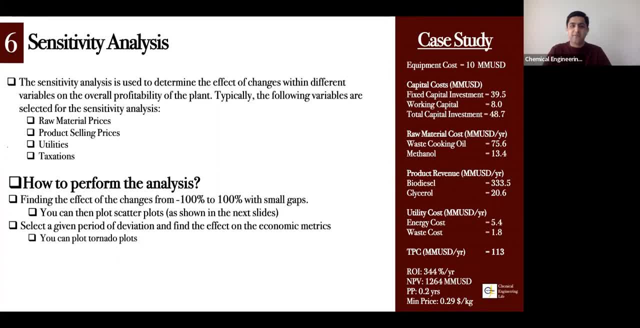 That is something that we cannot control. And therefore, we have to do something called a sensitivity analysis in order to understand how robust 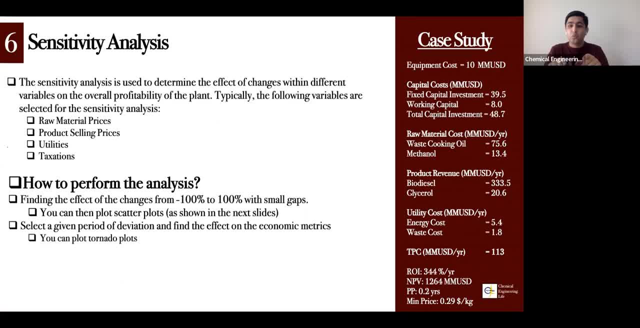 this entire process is. If there were to be any deviations within the prices of, let's say, raw materials, product, of our utilities, waste, and any other variable. 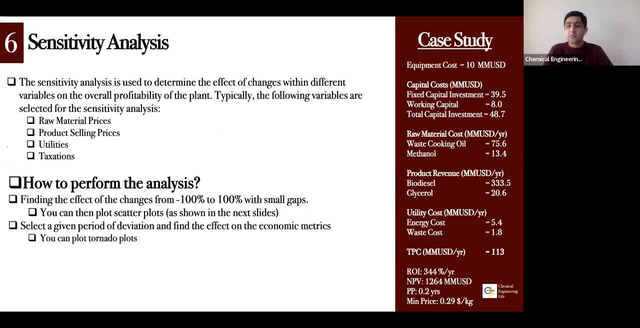 Let's say, if you wake up one day and your government decided to raise the tax from 30% to 50%, 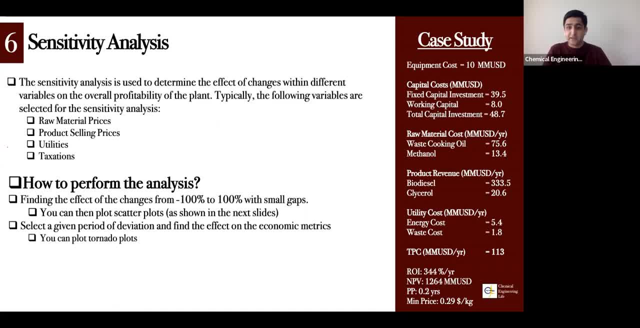 you know, you can't just go and say that I don't feel like paying tax because you have to pay tax. That is something that you have to take into account. Likewise, right now, we are buying waste cooking oil at $0.2 per kilo. 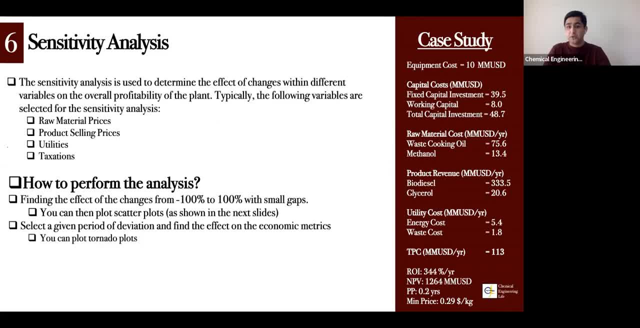 But what if your supplier gets greedy, and he finds out that you're making a great deal of money out of it, 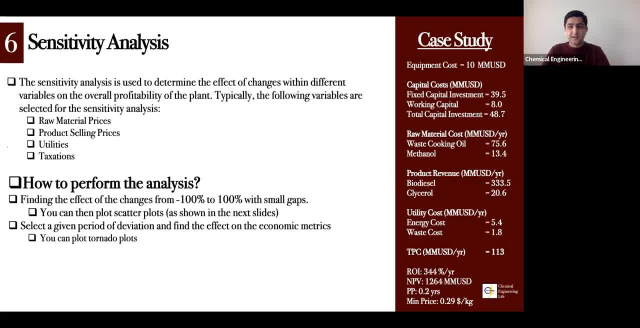 and he actually triples the price? Because that's how it works, right? If there is a very high demand, then the prices go up. 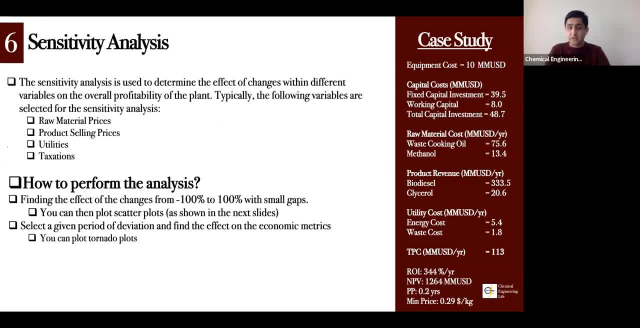 And that is something that will happen with waste cooking oil if this thing is commercialized. And that's why you have to take that into account as well. 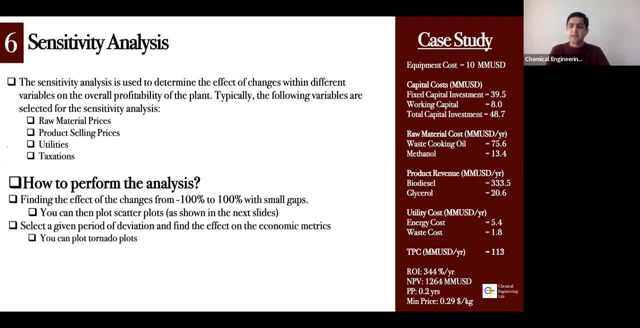 So therefore, what you do is that you select an interval. You select the percentage deviation within each of these variables. So then you say, and there are two ways of doing it. The first way is that you go from minus 100 to plus 100. So you select the value, the waste cooking oil, for example. 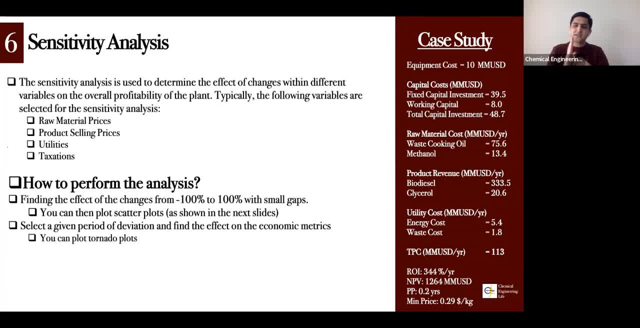 Let's say the cost is 0.2. You decrease it all the way up until minus 100. That means that, 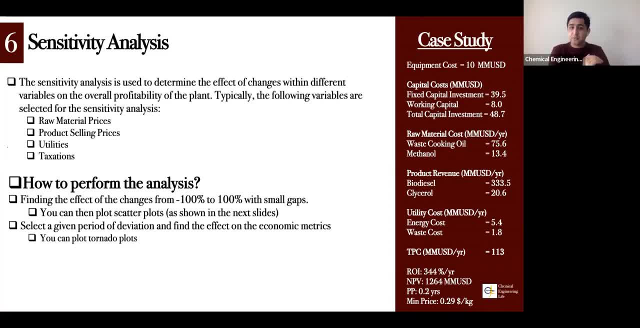 let's say the price decreased in value, decreased up until minus 100, 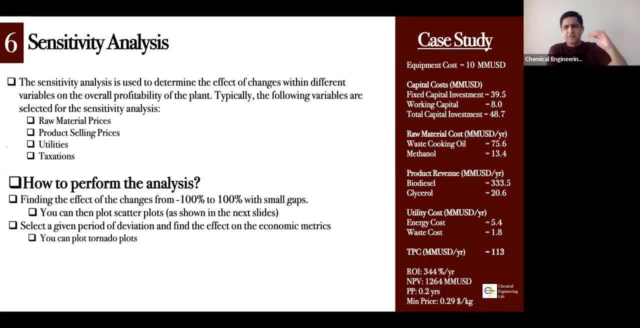 or it increased by 100% at different intervals. You could do 10%. You can do 5, 5, 5%. Anyhow, you go from minus 100 to plus 100. 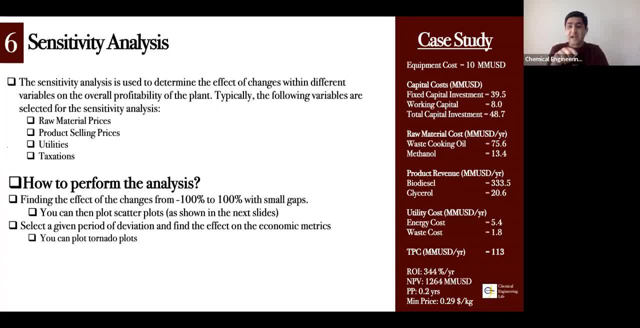 Then you can plot a series. You can use a scatter graph to show how it affects the economic metrics. 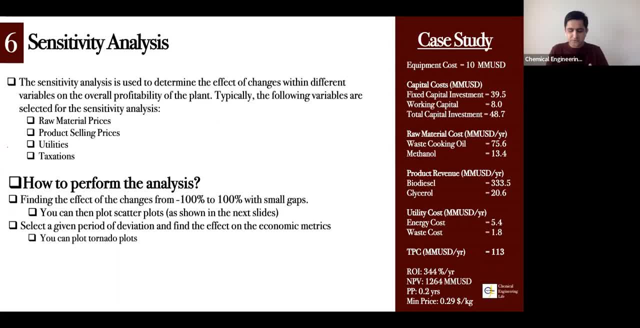 Or you can do something where you select a predefined percentage, let's say 30%. Then you only do minus 30% and plus 30%. 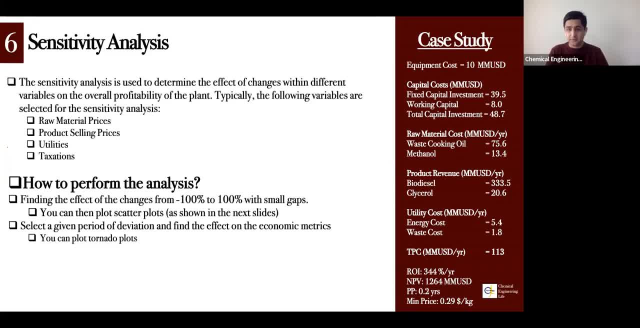 When you do those, then you plot something we call a tornado plot. 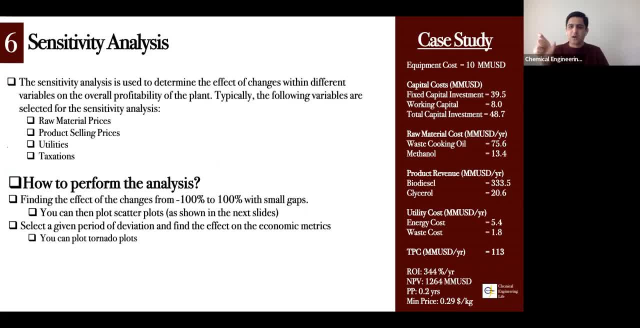 There you have a line in the middle, and it will show you how it deviates on both sides. 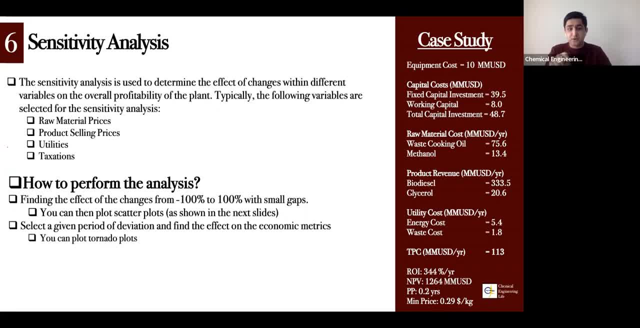 For the purpose of this slide, this webinar, I have decided to go with the minus 100 and then plus 100, 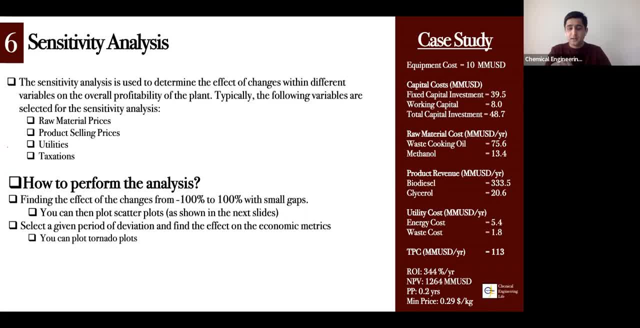 because the research paper that I shared with you before the webinar, they have done tornado plots. Therefore, 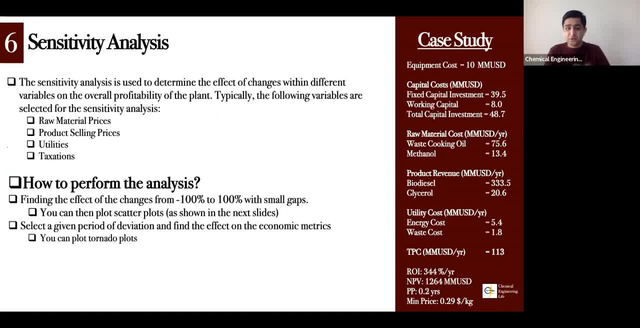 I thought that you could have a look there and see how it works, but they have not used the approach with the minus 100 and the plus 100. Therefore, I decided to go with that. 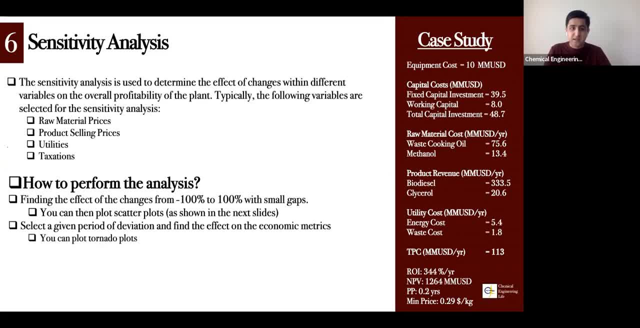 The majority of the time, the changes that will come, they are in the raw materials, product price, utilities, taxes. They are the only ones that are mostly uncertain when it comes to your economic analysis. 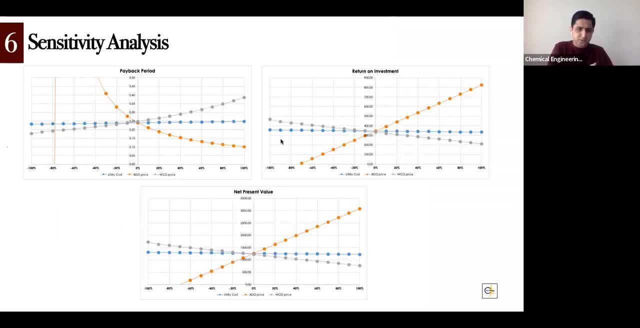 Like I said earlier, you can do the minus 100 and then the plus 100. 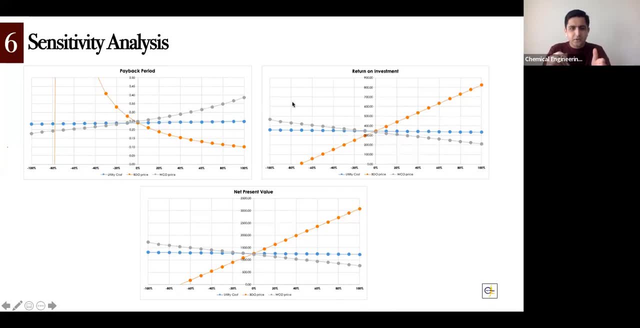 Then once you do it, the thing is that it's not simply enough to just plot line. 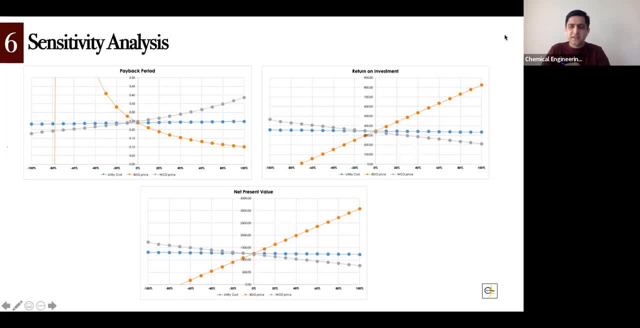 It is very important that you understand that what is the effect of each and every variable, on these changes. 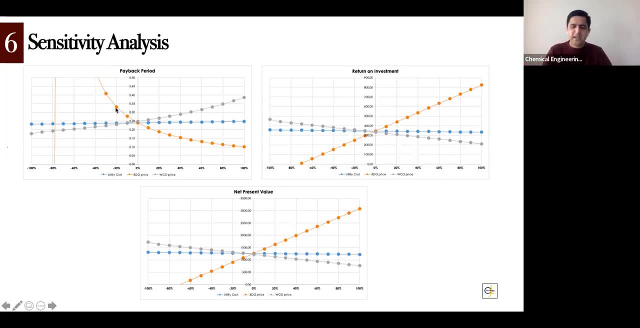 If you look at the payback period, the payback period is something that is directly related to our capital investment. The payback period is going to be more affected by our investment value, then it is going to be affected by our ongoing expenses. 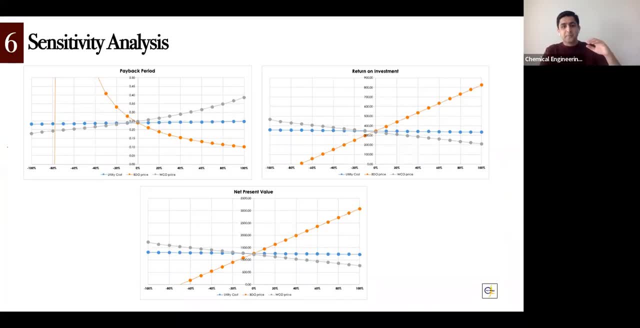 The reason being that, the ability, the expenses only affect our ability to pay back our loan. 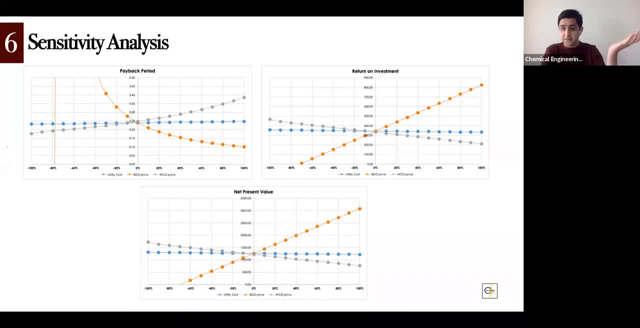 But if the capital investment is increased a great deal, that means that we will have to pay a lot more money back, and hence the payback period would increase. 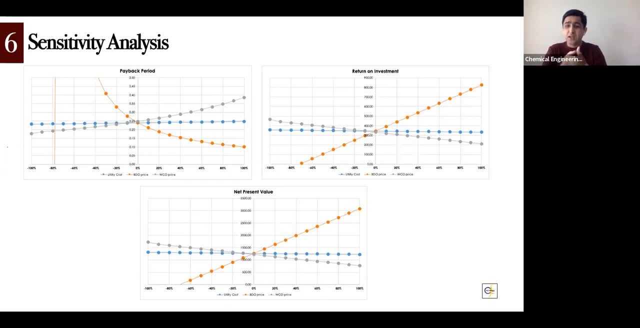 Typically, the payback period is much more sensitive to capital investment and essentially equipment cost, 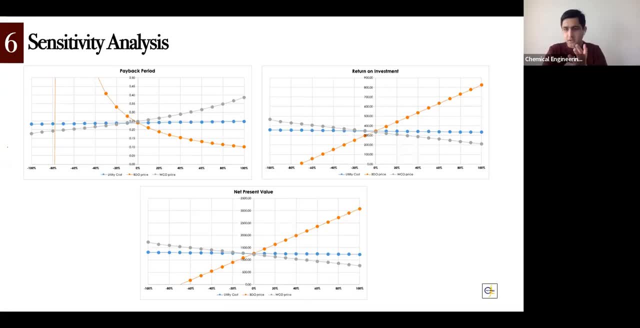 than it is to our other costs, like such as, you know, raw material cost or our product cost. 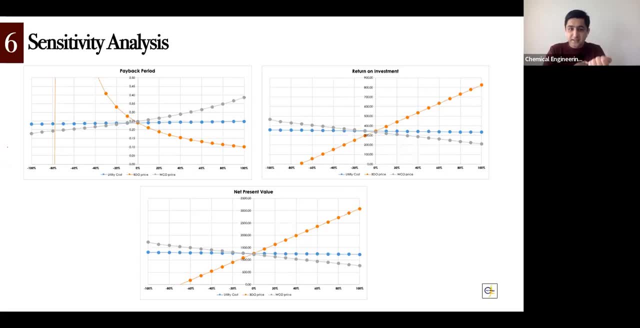 The product cost, if it changes, it affects the ability for us to pay back the loan, right? 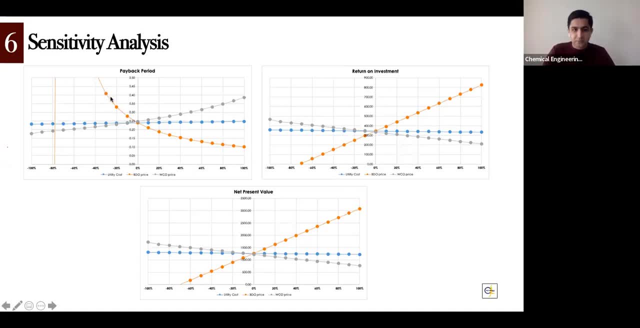 And you can see right here, if I change my biodiesel price, 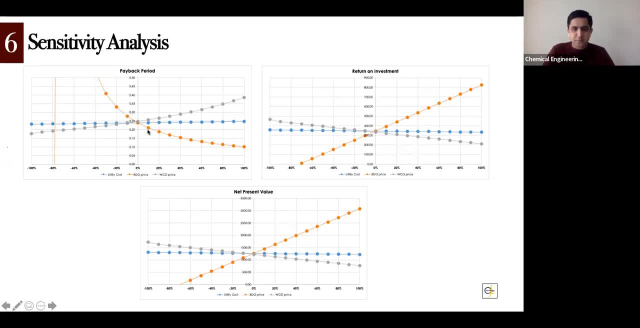 which is this orange line right here, if the biodiesel price increases, if it increased by 100%, 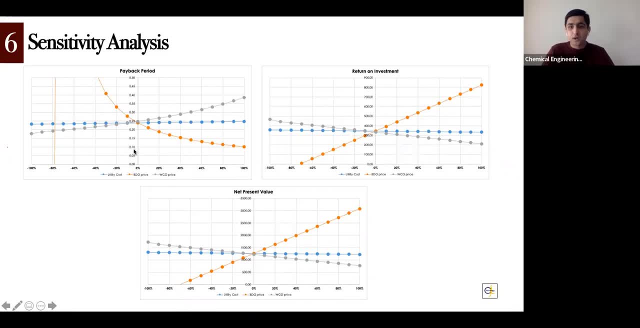 you can see I can pay back all of my loans within 0.1 years. 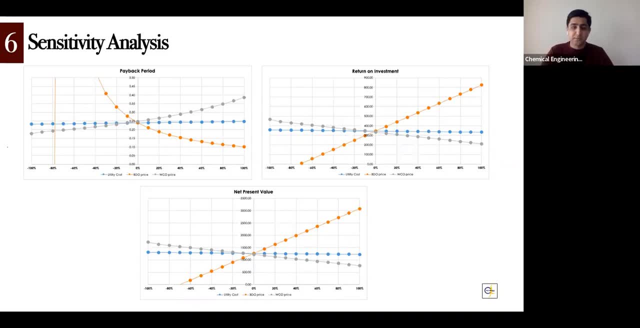 So it literally decreased by almost 30%. 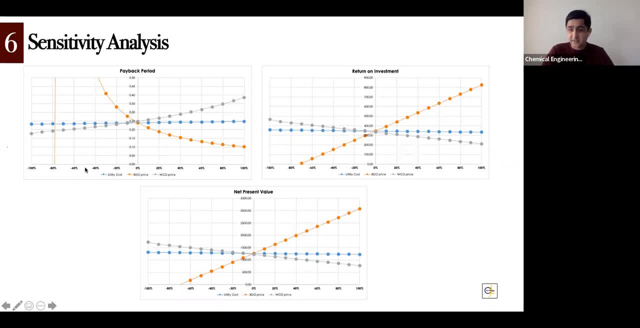 If my biodiesel price increased by 40%, and actually you can't see it in this graph, but if we went down to 60%, it would take us eight years to pay back the loan that we have taken, to cover the expense, the capital investment. So that means that our payback period is strongly dependent on our biodiesel price. If there is any change, if there's any decrease within the biodiesel price, that's going to affect our profitability negatively. 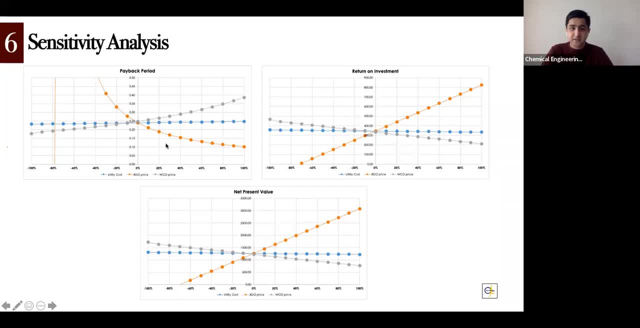 And that is very important. That is something that we have now understood in terms of the payback period. 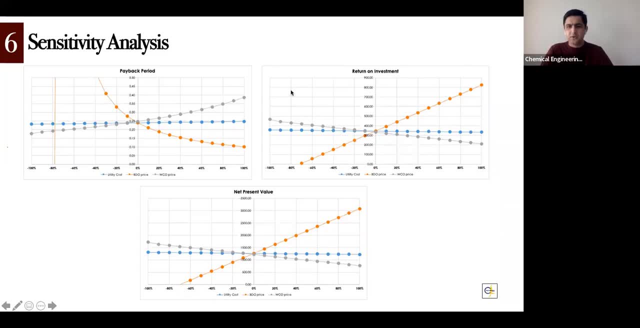 Then we come on to the return on investment. The return on investment, like I said earlier, it is the, it is the, the amount of profit, fraction of the profit, for the annual profit, divided by, divided by our initial investment. 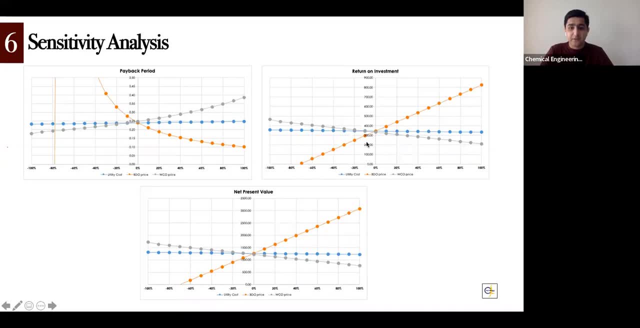 Now, likewise, our bio, if there is any change in our biodiesel price, it affects the ROI strongly. 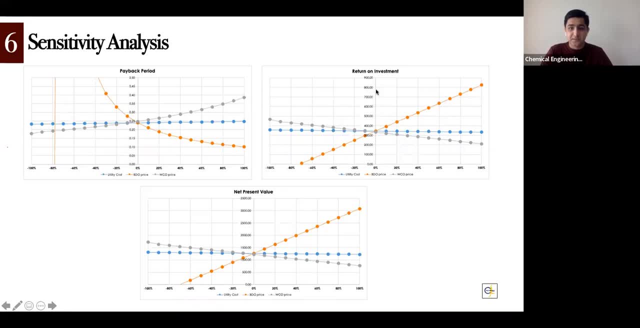 You can see there is a very strong change in our, in our value compared to our base cooking oil and our utilities. You can see the utilities, 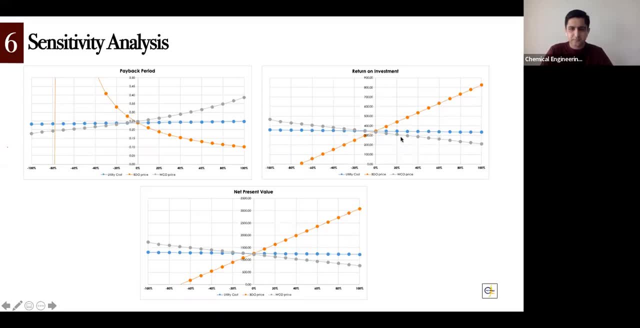 they have no influence on our ROI. 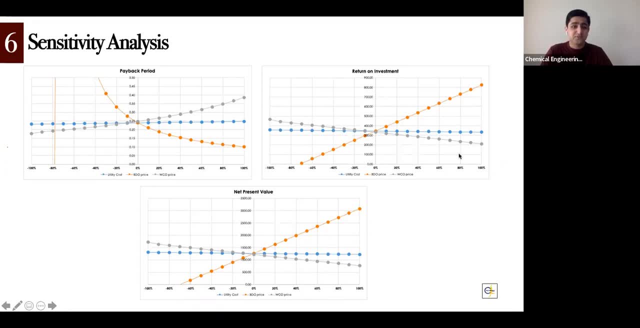 Likewise, the waste cooking oil has a strong, has a slightly medium influence. Why? Because if the waste cooking oil price goes up, that means that we need to pay, our profit is going down, right? 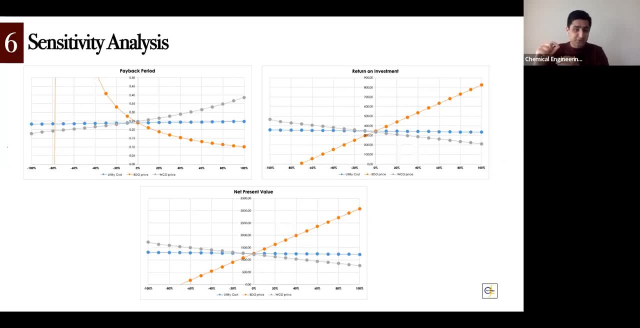 The less the profit, the lesser the fraction, and therefore the ROI is going to decrease. 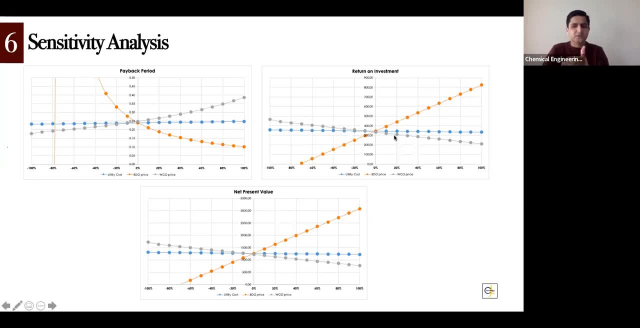 But since the waste cooking oil is not very expensive to begin with, therefore, even if we decrease, increase it by 100%, then it is not very much affected, and you're still very much in the profit zone, which you can see right here. Even if it is, if it increases by 100%, our ROI will still be 200%, which still, that means that we are still profitable. 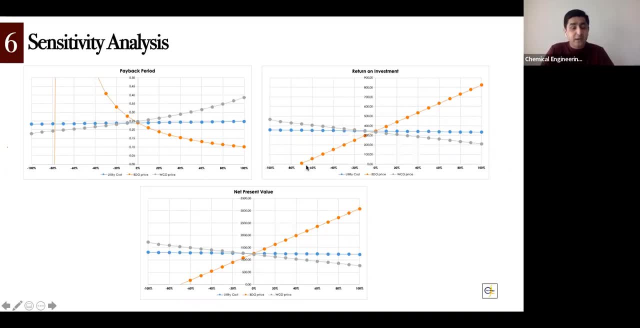 On the other hand, if our biodiesel price decreased by 70%, that means that we are no longer profitable. And I wouldn't even go up to the 70%. I would say if you're at around 60%, already there, we are hitting that around 50% mark. And already from that area, we can say that we will no longer be profitable. 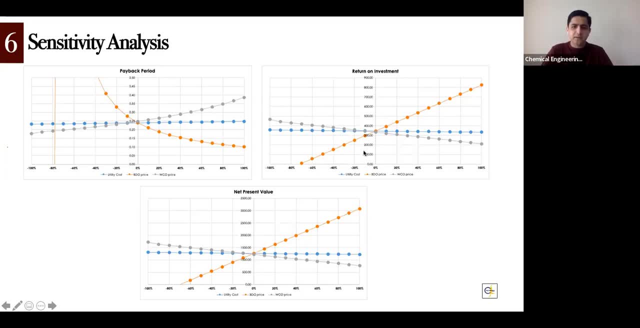 Likewise, and you have to remember that when we are looking at the curve of biodiesel, if you are at this stage right here, that means that you don't have that much place for other changes. So if you, if your ROI is only 50% to begin with, and if at that level, you have changes within base cooking oil or utility costs, then you would drop down to zero fairly, very, very, very quickly. 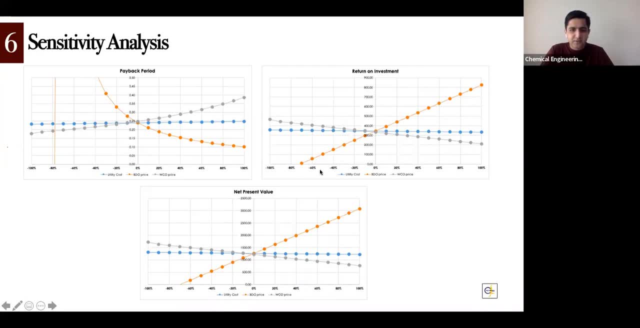 Therefore, you could always argue that around 50 to 60%, that is the limit that we can set. If the biodiesel price decreases by more than 50%, we are no longer profitable in terms of our return on investment, which you can see even now, return on investment and the payback period, there is a strong agreement between the two, right? 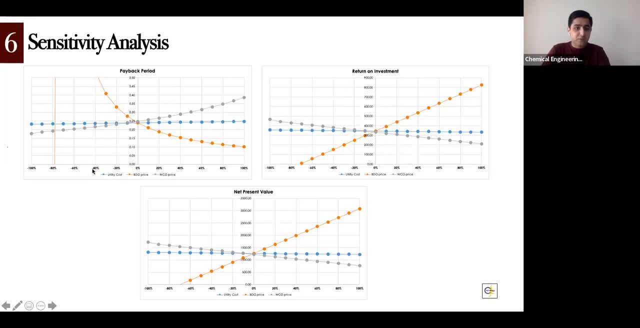 From this, we also found out that if we go below 50%, the payback period is more than eight years. 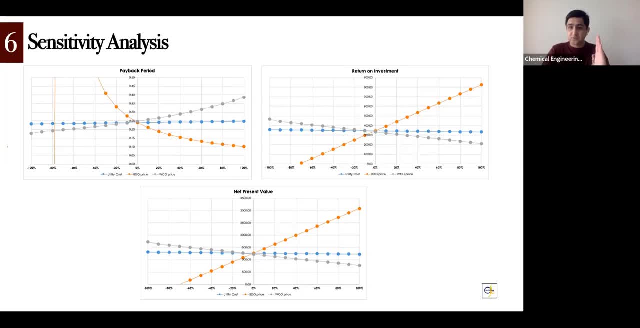 That means that 50% is the limit in terms of PP. Likewise, 50% is the limit in terms of ROI. 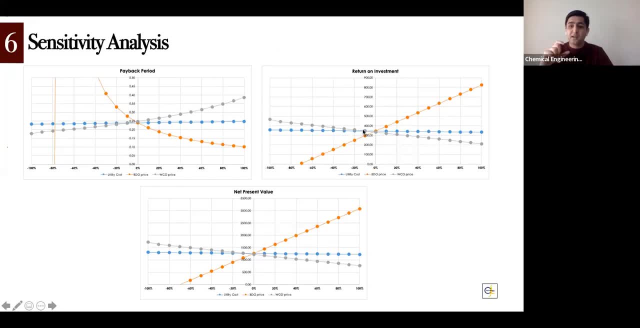 That means the main variable, that the pillar of our profitability is the biodiesel price. Likewise, 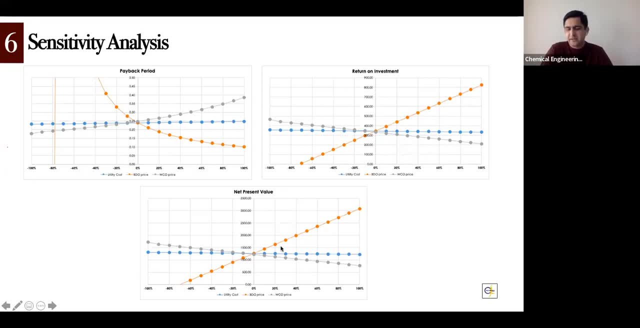 the net present value, this is the money, the time value, the more money you make, the more value you have. 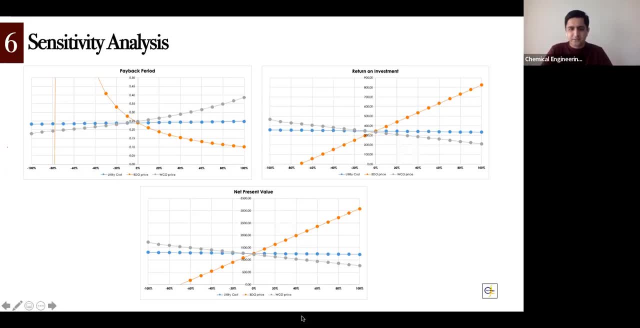 So in that way, you know, in that, in that regard, it is, it is of course common sense that the more expensive biodiesel is, the more money we make, the less expensive it is, the less money we make. 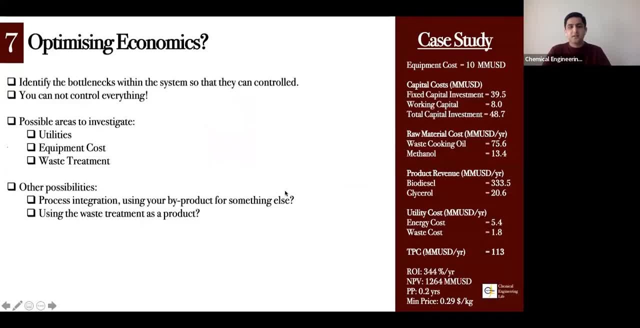 So now, finally, so once you do all the analysis, luckily in this case, it was profitable. We made a great deal of money, which was amazing. Many times you don't make that much money. 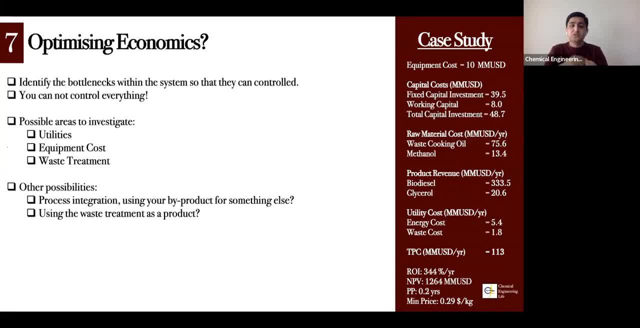 Instead of waste cooking oil, let's say if I had used soybean oil, soybean oil has a very strong market. 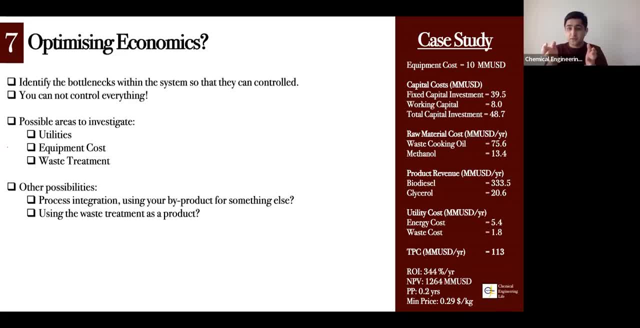 It's a very strong demand, and it is a very scarce material as well. Therefore, it actually costs around, I believe it costs around $0.8 a pound. 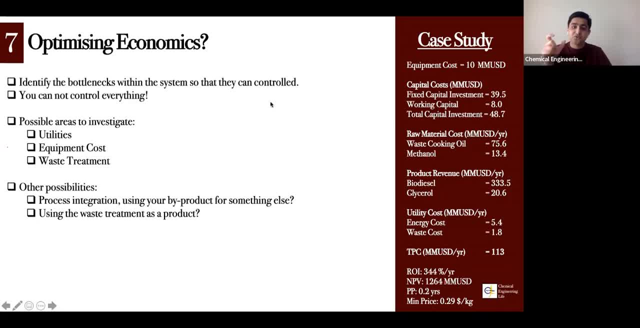 $0.8 per kilo. If I had used $0.8 per kilo as a price, we wouldn't be profitable at all. 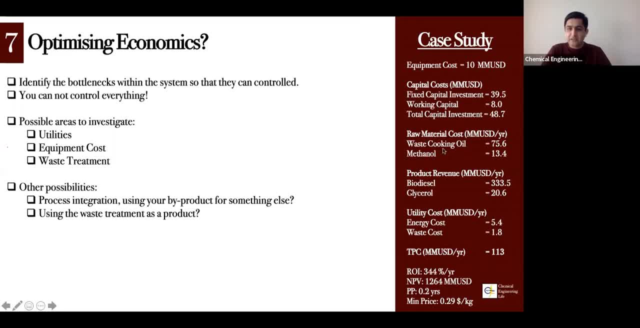 Because if you look right here, right now, waste cooking oil costs only $75 million, and it only costs $0.2 per kilo. 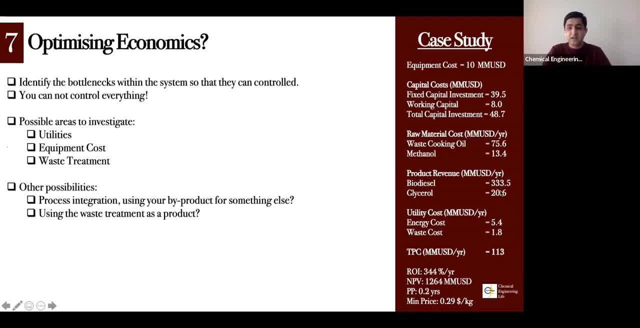 If you had used a more expensive oil, it would have been at the same level as biodiesel. 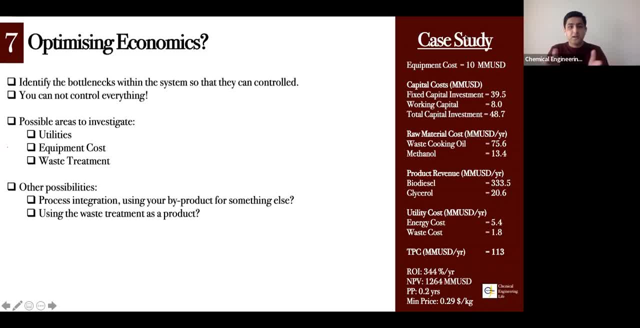 And that means our profits would not be very high. Therefore, 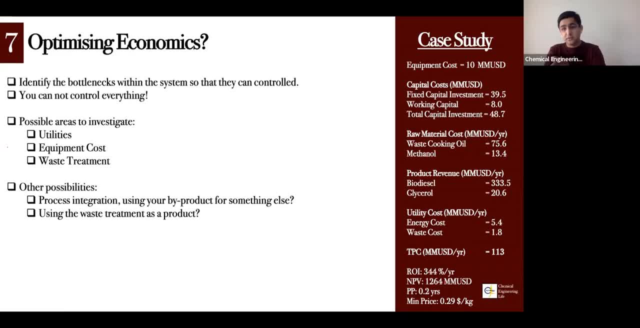 the first step is to understand if you can use a cheaper material to start with, or if you can, you should do it. Many times it's not that simple. 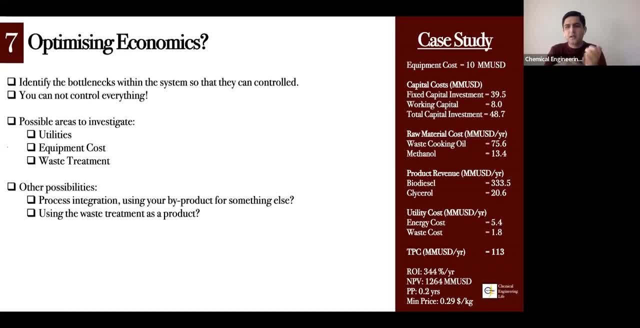 You can't just take a random raw material. Of course, it has to fit with your overall process, 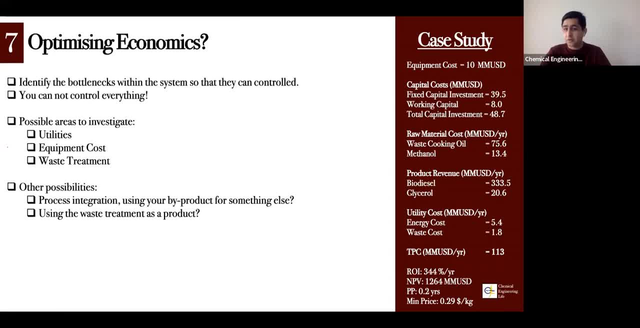 Finally, the utilities, they tend to be a bottleneck. 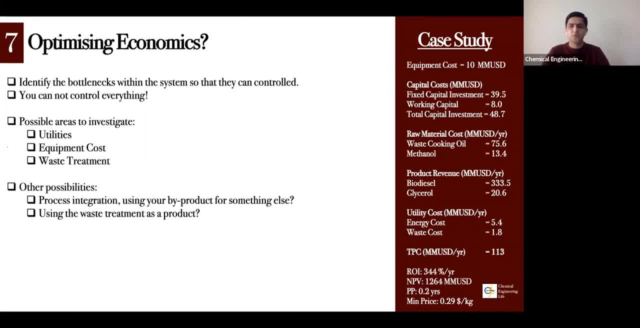 You could do heat integration instead of using so many heat exchangers. 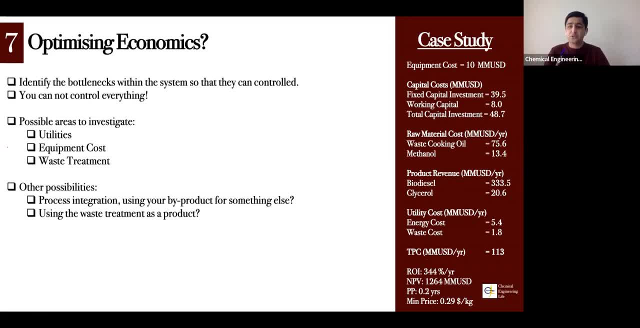 And to use steam and cooling water, you can do heat integration too. If you have a stream, process stream that is very hot and a process stream that is very cold, you can connect them if possible, and you can do the heat exchange there. 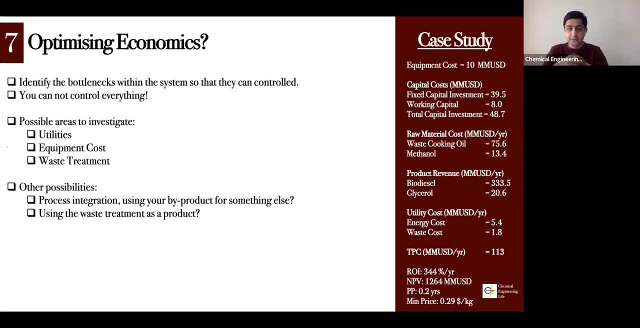 You could save a fortune on utility costs. Finally, you have waste treatment. 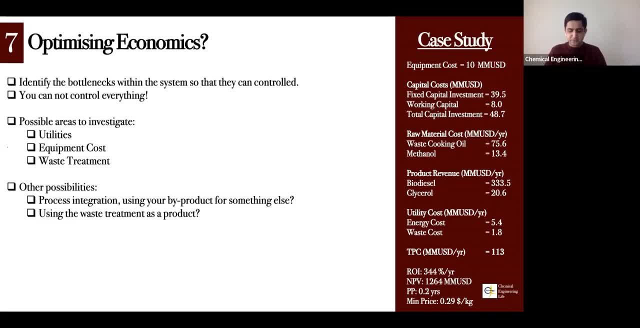 If you have a waste stream that you feel that you can purify and then sell it off, as an actual product, you should do that because instead of having to pay 2 million, you might end up earning 2 million. 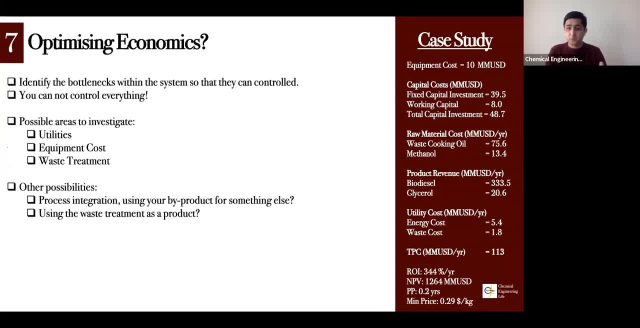 And every single penny matters when you're doing this technical analysis. 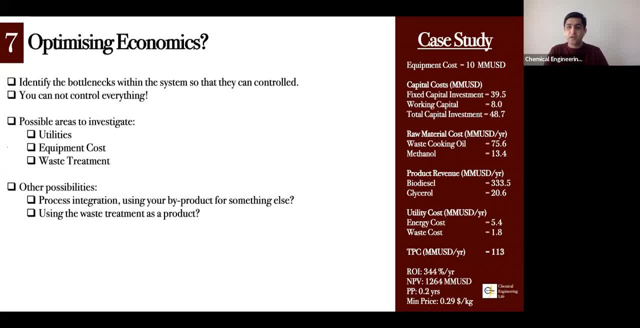 The biggest example is water disposal. If you have water, like for example, I designed a process once where I had a fermentation reactor and we were using water to dilute the process. After that, the same water then goes out. It was not being used anywhere. 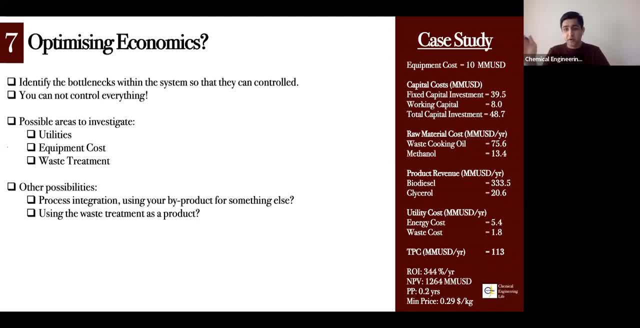 Instead, all that water then had to be removed from the process. 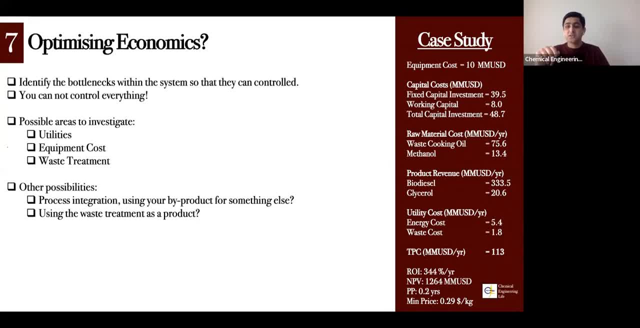 90% of the waste treatment cost was in the water disposal cost. 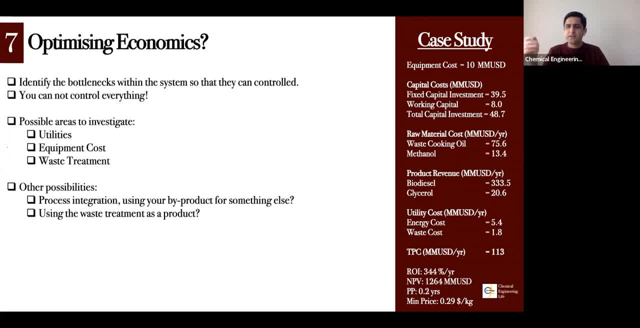 I mean, there's no point of literally giving away all that water. 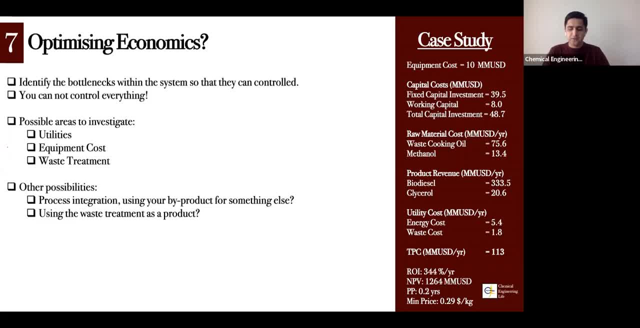 Instead, what you can do is you can either create a water treatment, 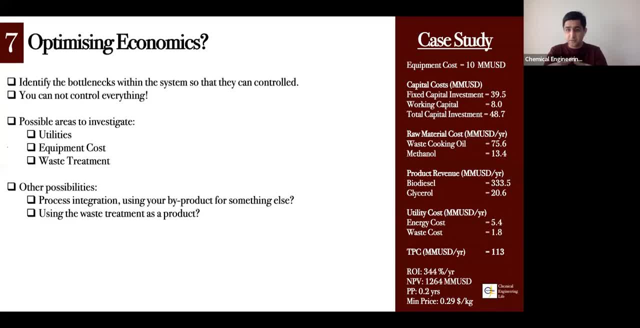 you can design a water treatment plant right beside your process and clean the water, and then reuse it back into the process. 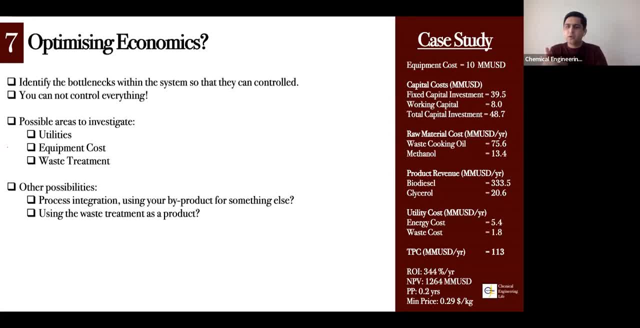 It may seem that it's going to cost you a lot more, and it will, in terms of your equipment cost, in terms of the utility cost. 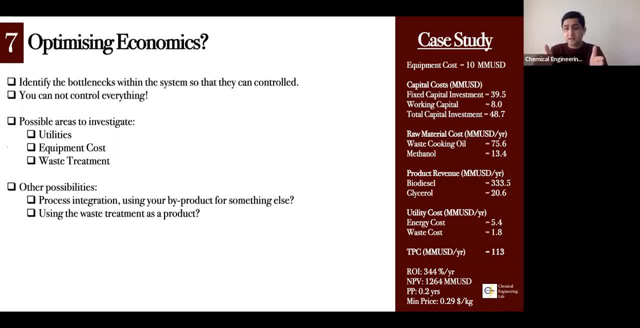 But in the long run, what you're doing is you're saving a lot of money. 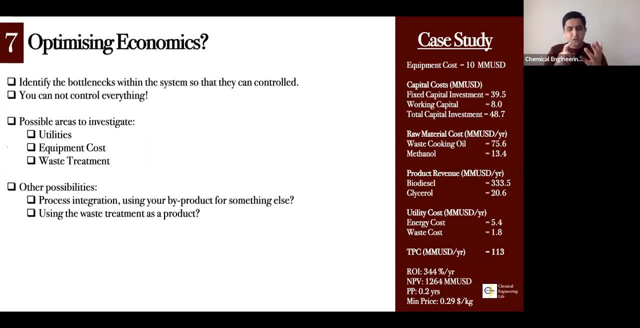 Because if you have to buy water every time, then you're no longer dependent on the market. Market deviation, the sensitivity is okay. 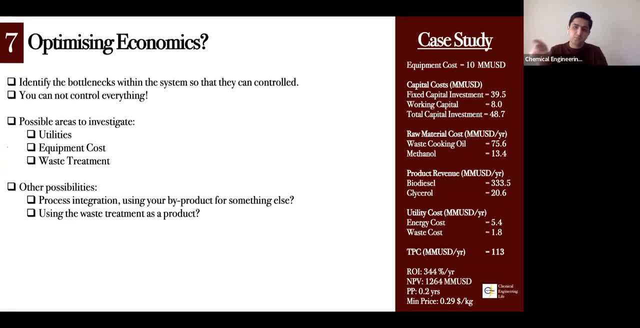 It doesn't matter because you only have to buy the water once. Then you can recycle the water, and it helps in the sustainability area. 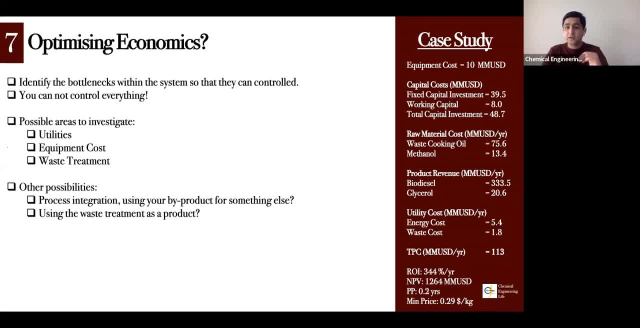 But these optimization techniques only work if you have money in hand. 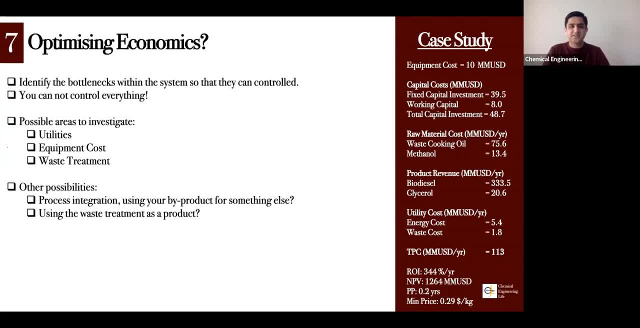 Like for example, I said the water treatment, let's say it ends up costing you 5 million extra, but you only have 2 million in pocket to pay for it. 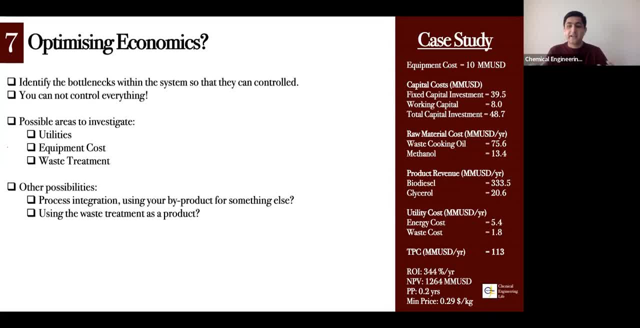 Therefore, you always have to keep in mind that these things are interrelated. 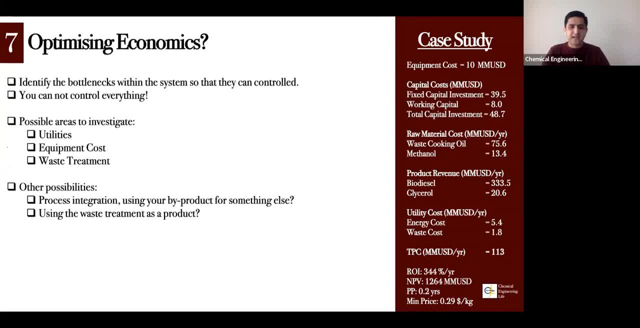 And something that I was told when I was doing it, that half of the things are common sense. As an engineer, you need to use your common sense and to make sure if these things work or they don't work. 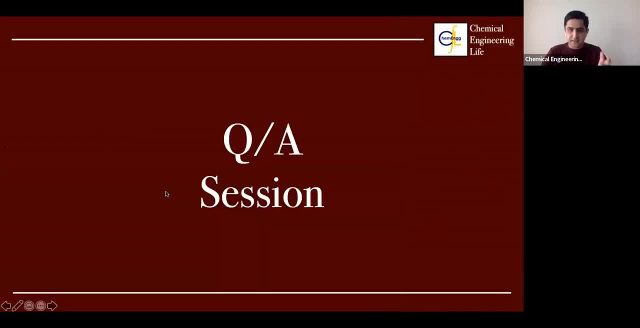 And I believe that is all I had to say about technical economic analysis and the values of production. So if you guys have any questions, you can feel free to raise them in the chat or you can unmute yourself and ask. 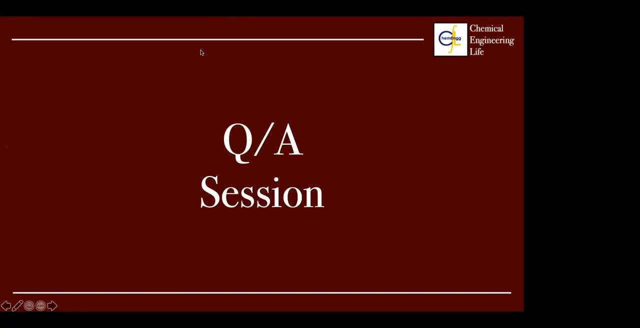 Hi there. Hello. Thanks. Yes. Hi. My name is Akhil. I'm calling from, I'm dialing in from Cape Town in South Africa. I'm a master's student at the moment in chemical engineering at the University of Cape Town. Thank you very much for the presentation, chemical engineering life. 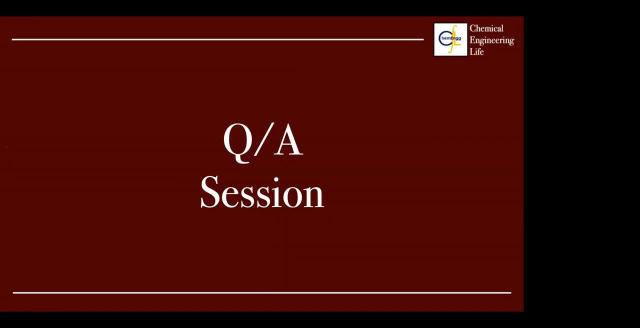 And thank you very much, Hamza, for the interesting presentation. 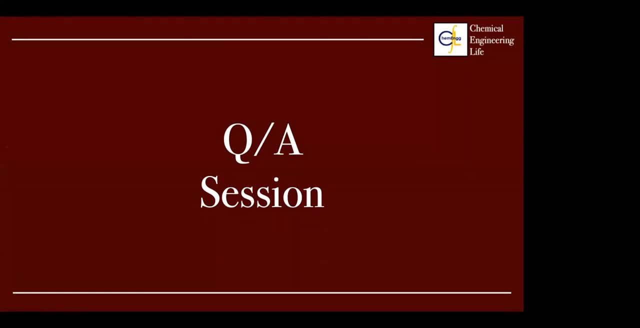 My research project is actually on a new process developed by University of Cape Town, where I'm conducting technical economic analysis on this new process 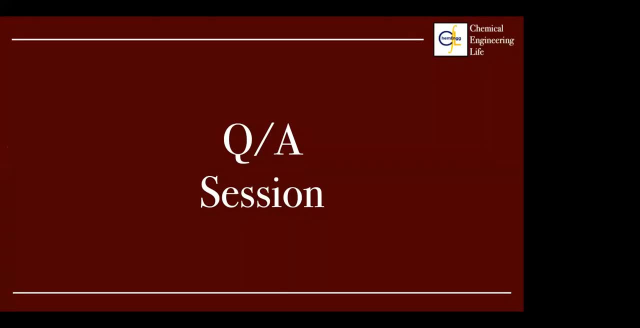 in collaboration with a commercial partner, with a cosmetics raw material producer. 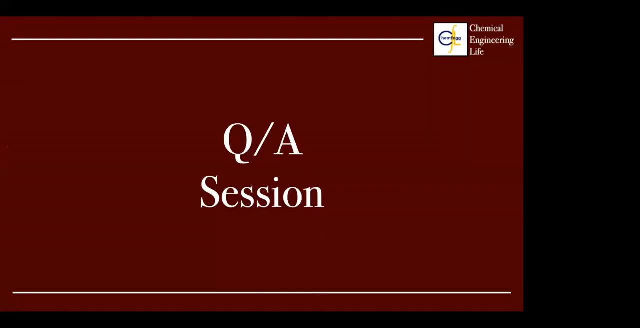 And therefore, you know, going further than just kind of 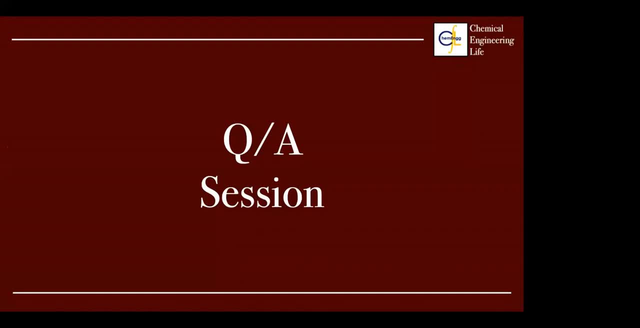 the theoretical technical economic analysis, a lot of my work or a lot of the focus of my study is in fact to get actual equipment costs 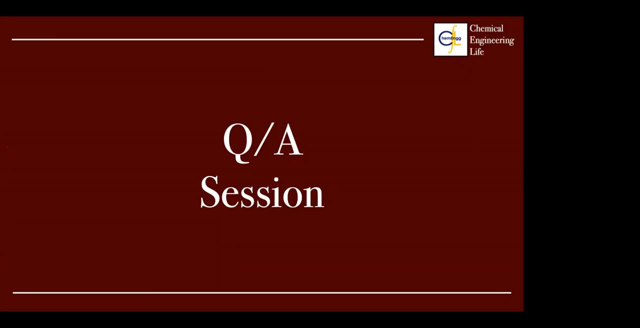 and actual cost estimations for me of the inputs to a model like this. 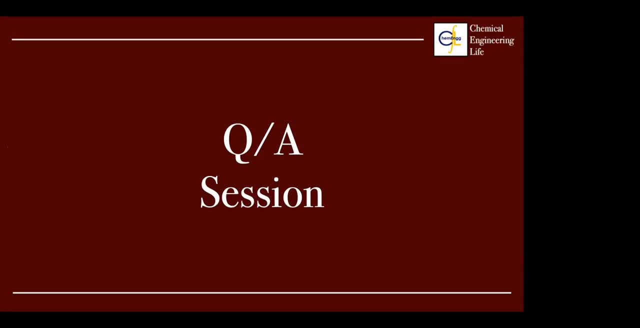 And I'm glad that you also mentioned, you know, under the uncertainty analysis, I'm doing a Monte Carlo simulation because a big part of my project is in fact conducting a Monte Carlo simulation. 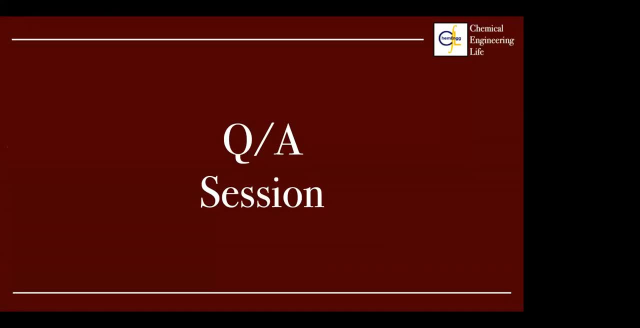 And I'm doing it in Python, just because of the programming abilities of Python. 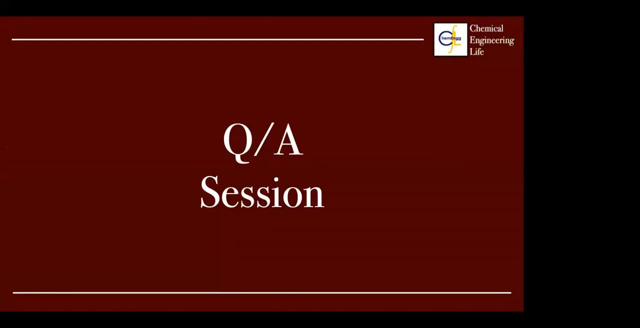 But I mean, a lot of my difficulty is just finding relevant factors, 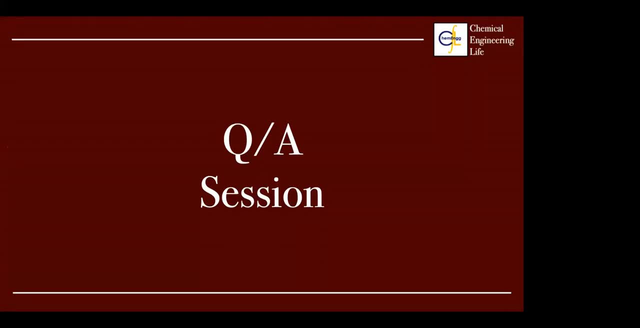 both from literature and from suppliers and commercial partners as reliable inputs into my process. 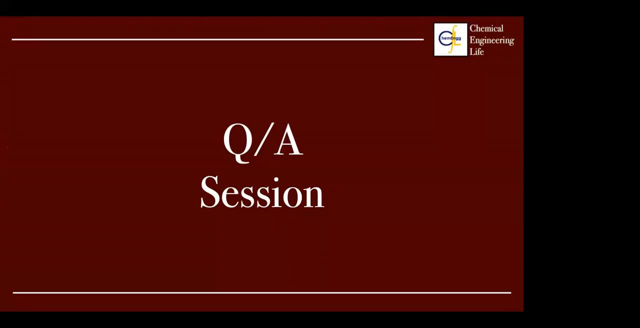 Maybe my question then just to the broader audience is, you know, are there very reliable and well-established and well-understood resources, handbooks for not only for literature, 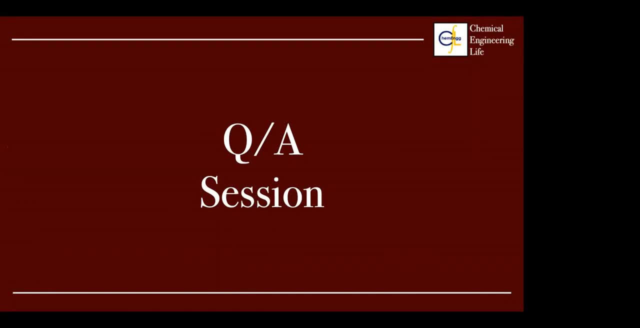 because a lot of the literature I've gone through is laboratory-based studies, you know, 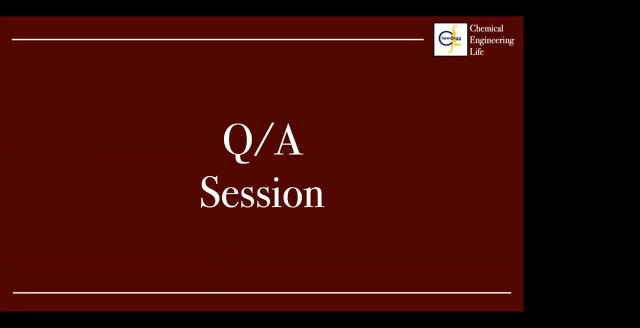 utilizing the performance of laboratory equipment, such as centrifuges, et cetera. 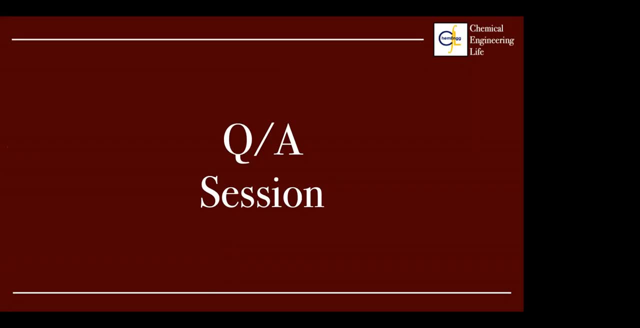 What is out there in terms of the more industrial or information on industrial equipment performance? 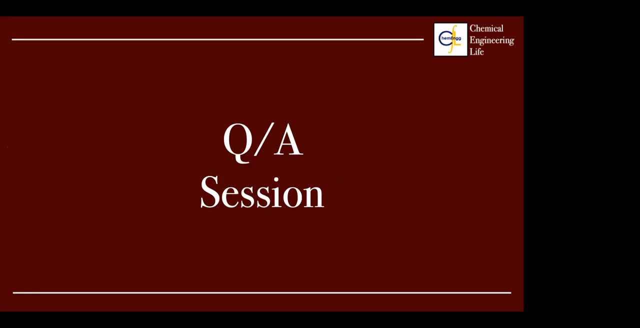 So for centrifuges, for aqueous two-phase, a big part of my project 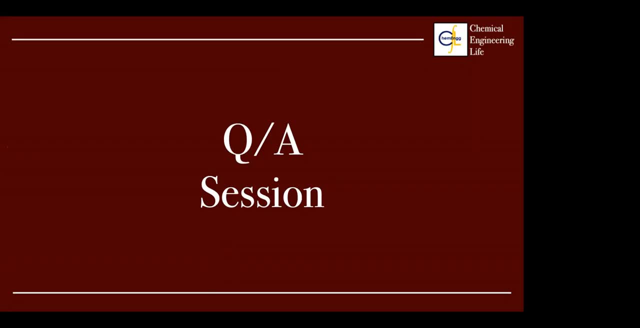 is understanding the aqueous two-phase system, which good layers. 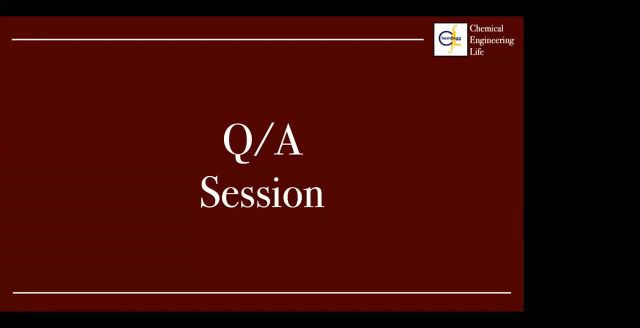 So yeah, if anyone or yourself and anyone has come across such resources, where could they be found? I mean, that is a very good question. 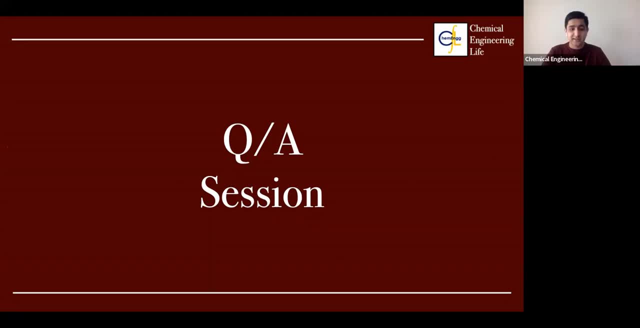 And let me begin by saying it's not easy. It's very difficult to find these forces and these factors, especially for equipment that you mentioned. 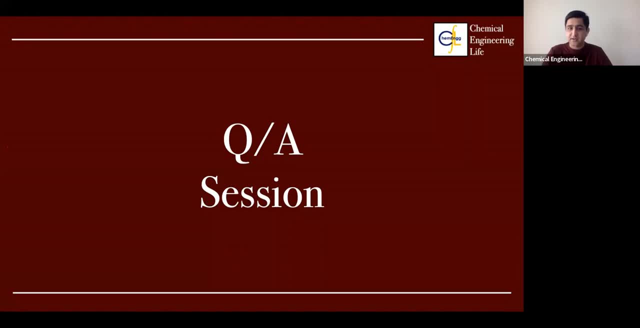 Like it's very, it might be very easy to find it for flash tanks, but when it comes to some less used equipment, it tends to get very difficult. 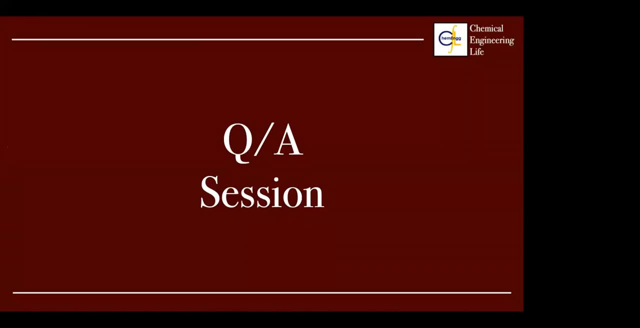 And the way to do it is that, like what I did was 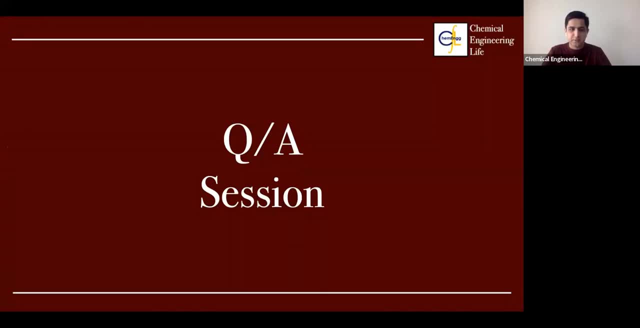 when I was doing my thesis back in day and doing my technical analysis, I used this, 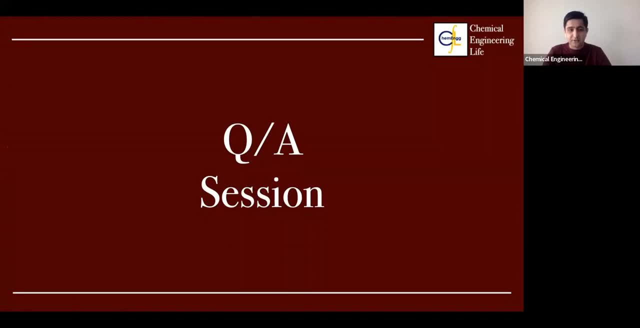 I have forgotten the name of the organization that have done the paper, but I can share that with you later on, on email, because they have validated 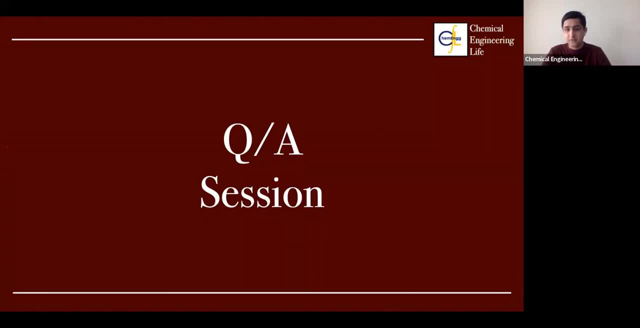 and verified an industrial example and all the factors that they have used. 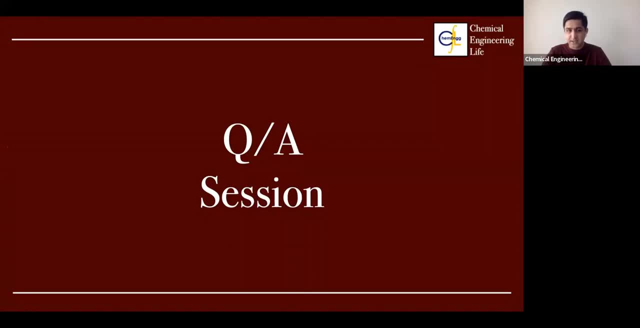 So I would suggest that you can use that. And I believe they have given examples of centrifugers, flash tanks, and all of it. And I believe that they, 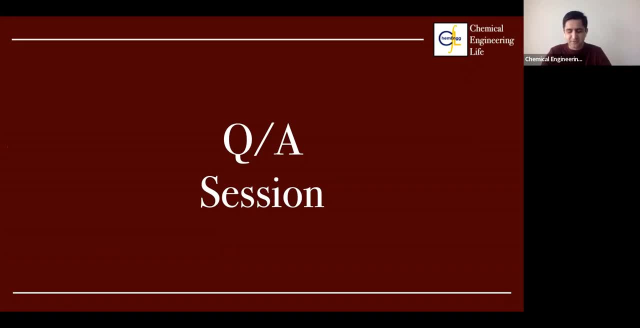 I'll find it and I can share with you right now because the name of them is not coming in my head right now, but typically I use those. 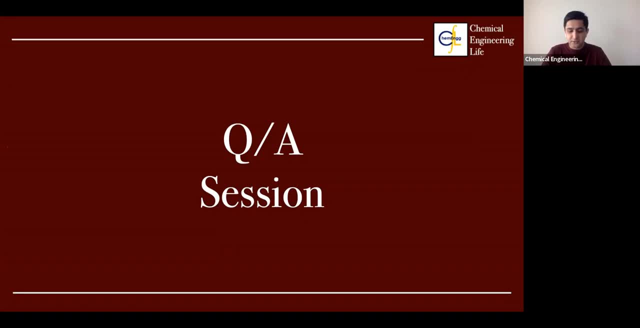 And like I also said earlier, that it's always a good idea to use validated papers. And verified organizations to take these values from, because there are multiple research papers that you can use, but many of them are theoretical. And there are a few papers out there that are based on industrial example. 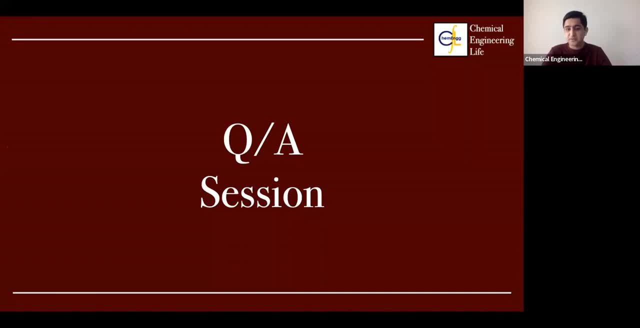 And the one that I'm referring to right now is actually based on an industrial example that has been implemented. And from that, they found the values. 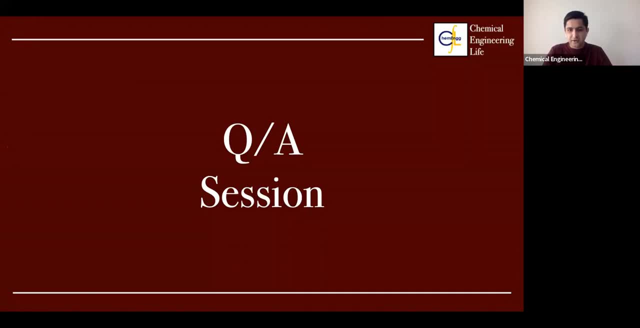 You could also, so that's regarding the equipment cost and the factors. Secondly, 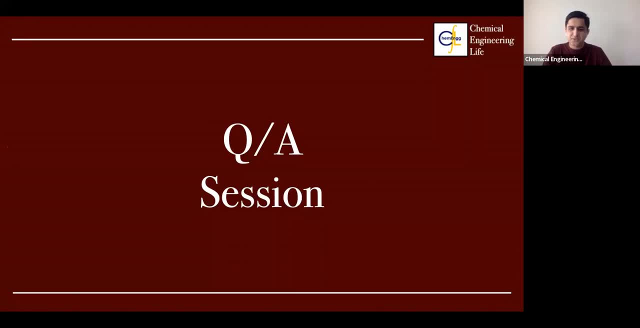 you could also, what you could do is, like I said, so there's this book, 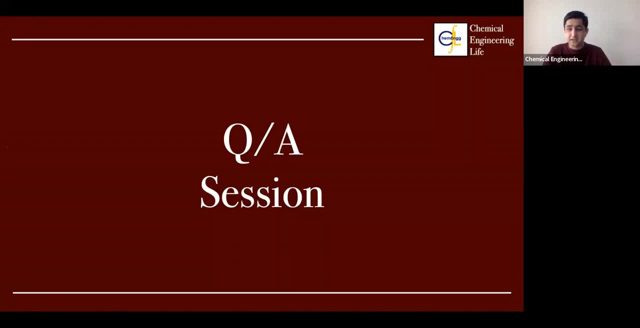 this Plant Economics and Design for Chemical Engineers. It is a very good book. 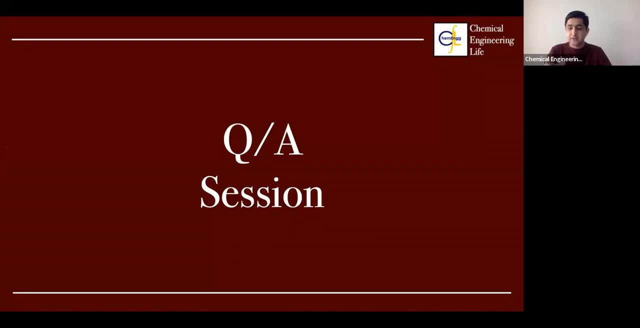 They have defined the methodology and they have defined the constraints, the brackets for different factors, especially when it comes down to, like for example, how to calculate the capital investment, how to calculate the TPC. But I would strongly suggest you use that as well. But- Is that by any chance a textbook? is that by any chance the textbook by Turton? It is by Peter and Timmerhaus, I think. Peter and Timmerhaus. Okay, I'll take a look at that. 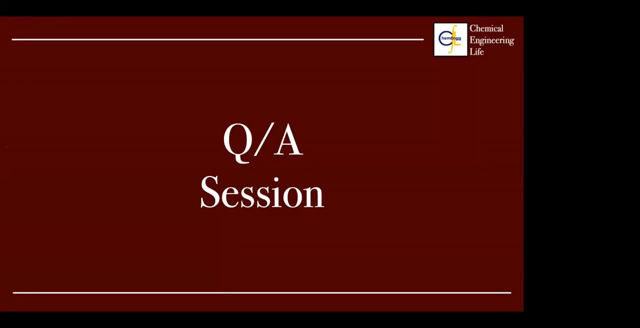 If it is, I'll share the information of all the papers and video right after the webinar. And actually with everyone that is in attendance. So you all can have a look at that on the material. 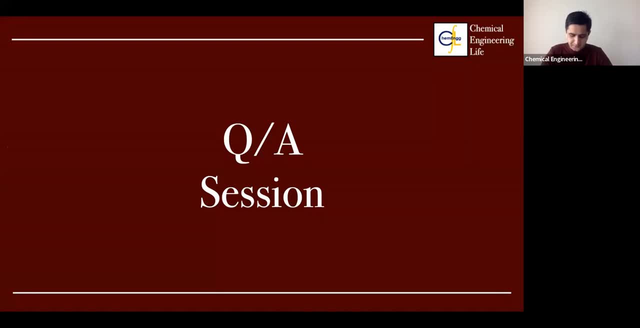 But yeah, but you just have to, you know, look out for all these equipment. 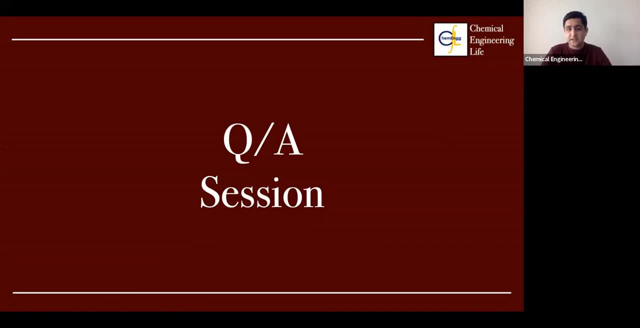 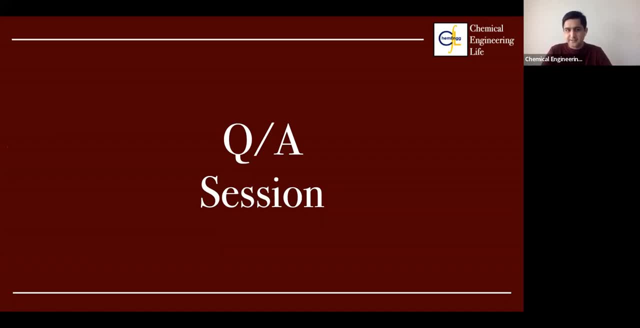 when you use working with utility costs, for example, I, like, like when I'm, like, I designed this plant in the US. 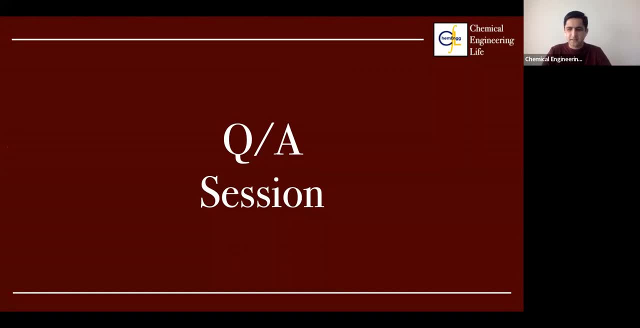 So then I used their, what do they call it, the EPA, I think, not EPA, like their National Electricity Organization. I don't know what the name is, but I went to their website and I used theirs. 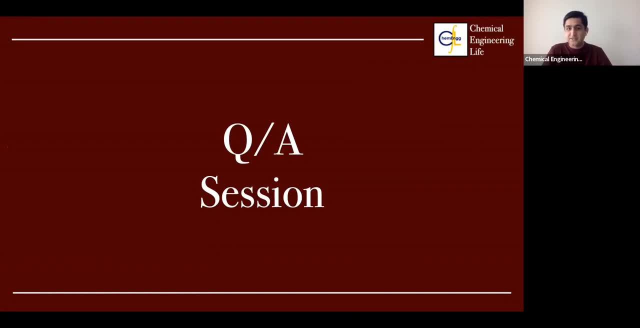 So if you're doing it in Cape Town, for example, then instead of using literature, to actually the values, it's always a good idea to just take directly values from the actual 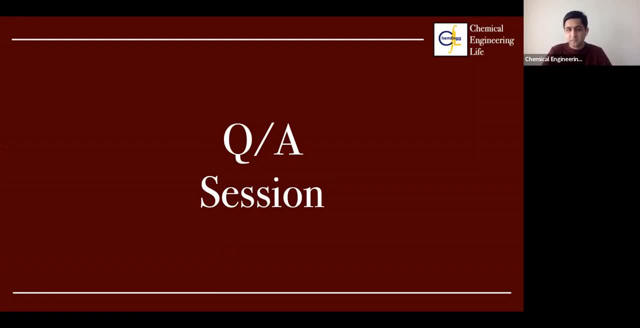 company, countries, you know, your, like, what do you call it, the people that are providing electricity and so on. So that's one way to go. I'm just sorry, just thanks, thanks for that answer. And it would be great to receive those resources. Coincidentally, I'm, I'm also busy with a 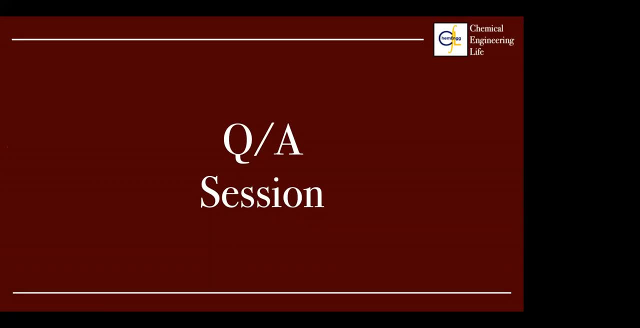 chemical engineering consulting project for a company in Kenya. 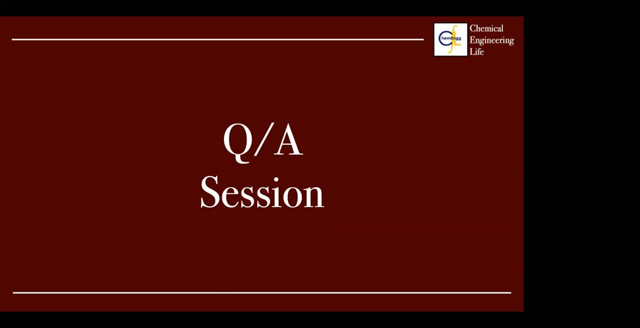 So I'm going to be working with a company that wants to turn an alternative oil source into biodiesel. 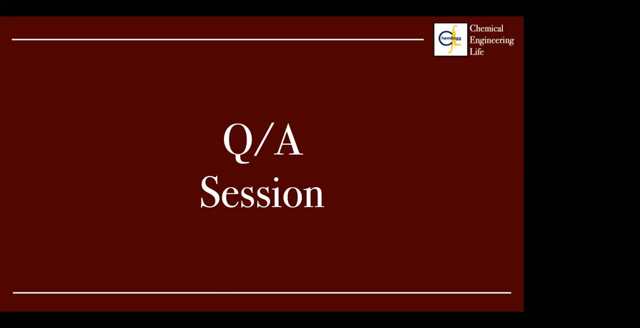 So it's quite interesting seeing the, I know of a few other companies that use waste cooking oil. 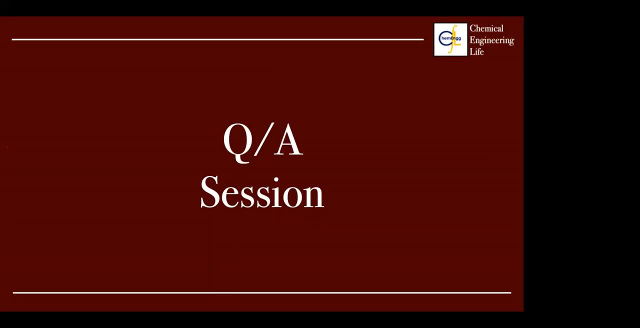 And I, as, as you presented the conclusion, I guess, based on engineering judgment and common sense is that using waste cooking oil will be very profitable because you're paying very little for your, for your raw material 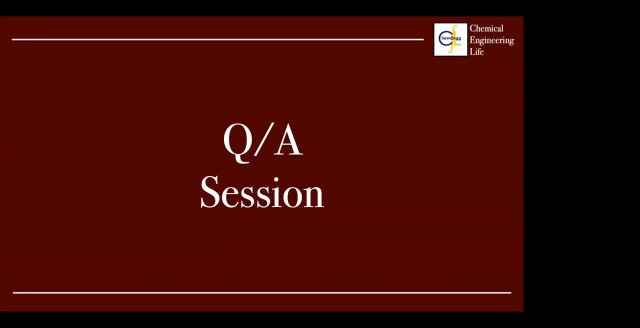 and methanol isn't, you know, you're not going to be able to do anything with it. 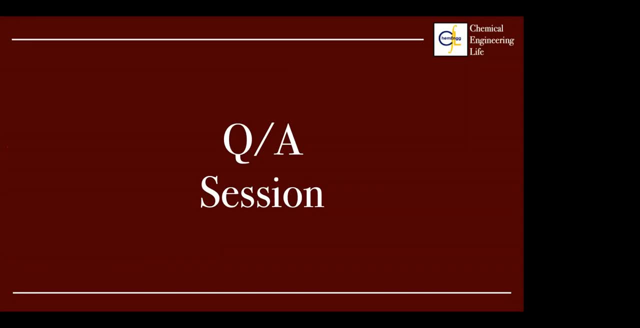 So I'm just interested in seeing how that plays into your, your, your, your, 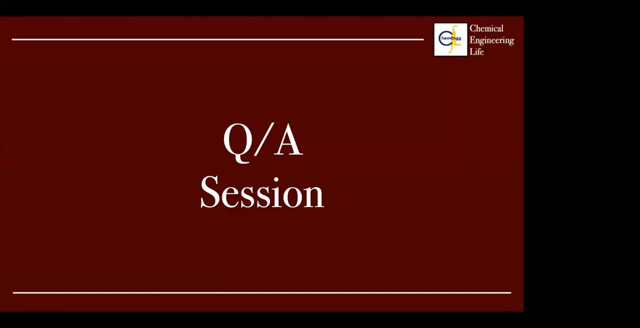 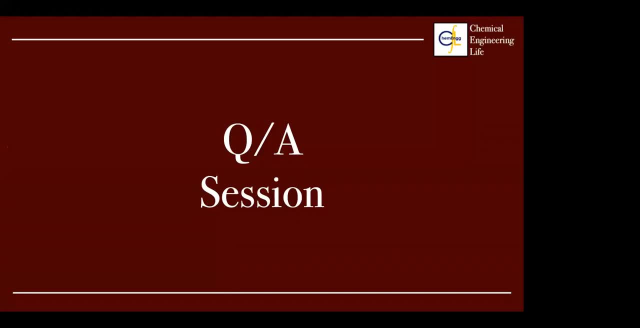 your, the early 2000s where everyone wanted to kind of produce biodiesel but the economics were just too 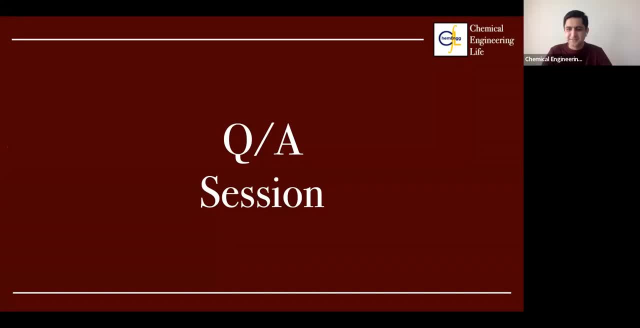 sensitive for any investor to really buy in long term exactly um but yeah these alternative waste uh all these alternative oil feedstock streams are becoming very popular just because of that economics because of the difference between the biodiesel cost and that raw material cost which 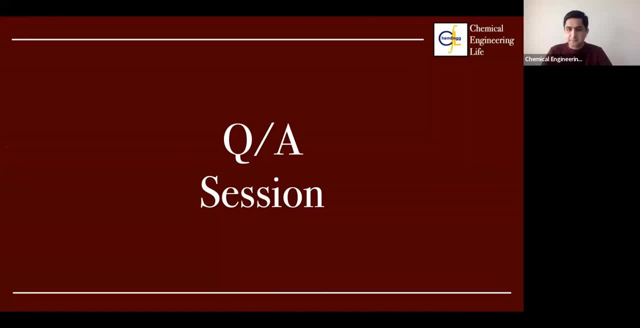 is which i found was quite important exactly yeah thank you for the very interesting presentation 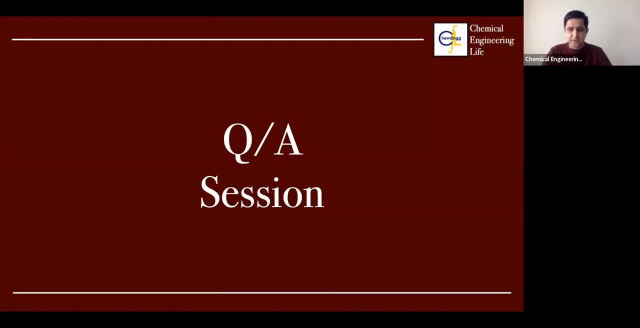 yeah well thank you i fully agree because the thing with soybean oil is that the soybean oil itself is a very high demand as a raw material so you can use soybean to produce so many other 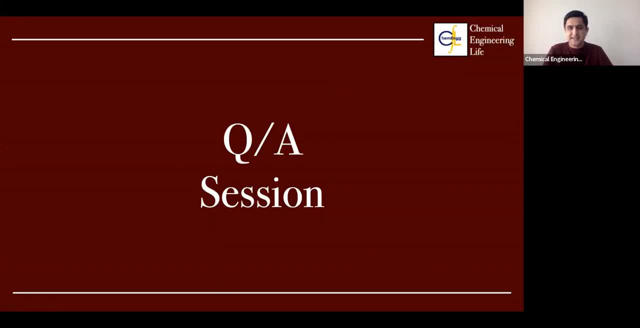 products and uh like i said for like already at this stage you can you can look at it you can say that biodiesel it sells at a price of 0.9 dollars per kilo soybean itself costs around 0.8 dollars per kilo so the only profit you're going to be making is 0.1 and that is that is a limitation when you use these uh these oils and but luckily the waste cooking oil and i and i personally believe that that is a very great way of producing biodiesel because i mean it's a waste stream you know you're not really using it for anything else you don't have any uh other 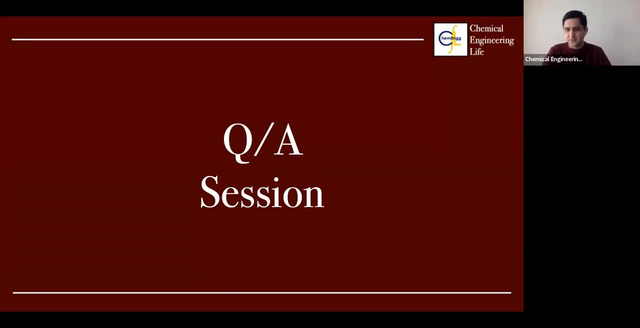 competitors for waste cooking oil and that is of course the main reason why it's so cheap 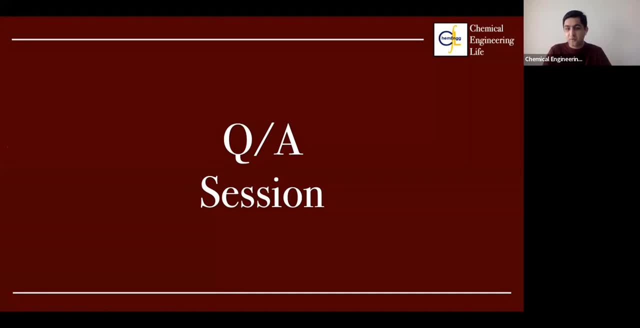 but in reality but in maybe in coming years it will also become more and more expensive as we get but hopefully so will biodiesel as the demand goes up you're very right 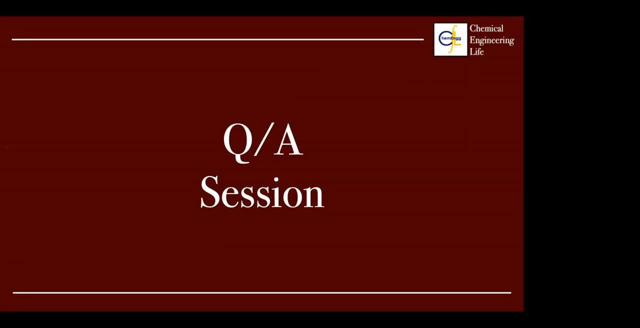 yeah just i i actually know of one company that i was once in discussions with um it's a company called neutral fuels based in dubai in fact and they their whole business model is based on using waste cooking oil to convert to biodiesel and then selling back that biodiesel to the commercial partners that they get the waste cooking oil from so they're very targeted in terms of their marketing and their and their commercial relationships with um a lot of major restaurant chains um and some i think logistics you know companies which are obviously very interested in being able to reduce their carbon footprint while while achieving some cost benefit from using an alternatively produced fuel exactly so that would be quite interesting to to look out for yourself as well um if if you exactly yep thank you thank you for yeah thank you for that interesting that that's quite interesting and like you know like you said yourself a lot it is quite profitable a lot more and more people are going towards it 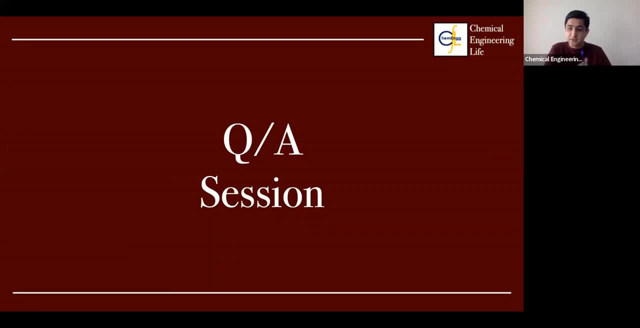 it's a good thing yeah i think it's a good thing that you're moving away from petroleum towards 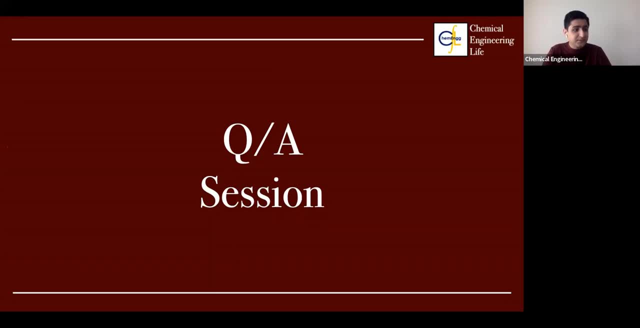 like for example waste cooking oil i believe only in the u.s they they produce like uh i don't like millions of barrels of which cooking oil and it is a waste product that you're not getting that we cannot get rid of so if companies like that are investing in reusing that then it's great 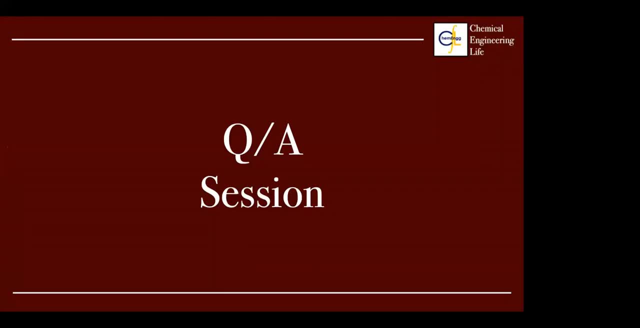 for the environment itself so yes it's great that it can work out for everyone yeah and what would the name of the company that you mentioned sorry neutral neutral fuels neutral fuels okay great 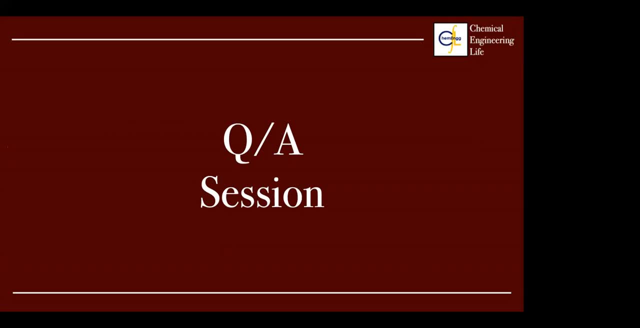 i'll i'll remember to check them out so thank you does anyone else have any questions okay okay okay hi 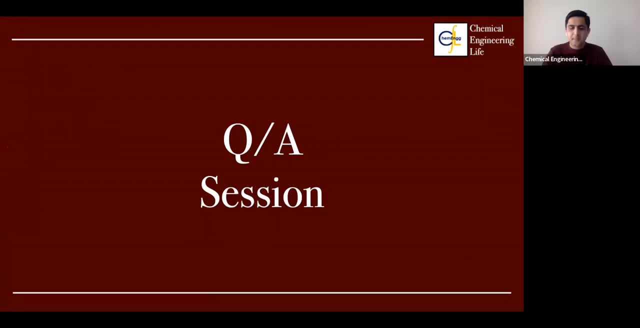 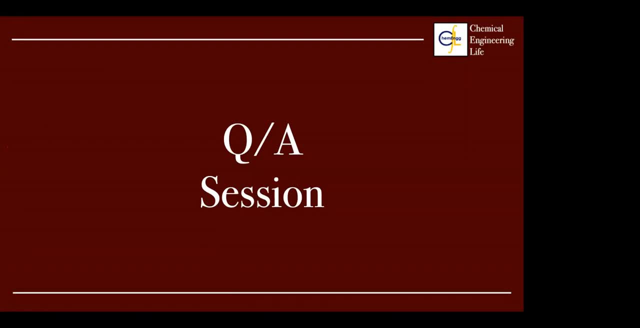 there's a huge amount of biodiesel produced worldwide i mean waste cooking oil produced worldwide yes it's a good option for biodiesel production but the supply logistics is not the supply chain it's not really um effective it's not we don't have existing supply chains and 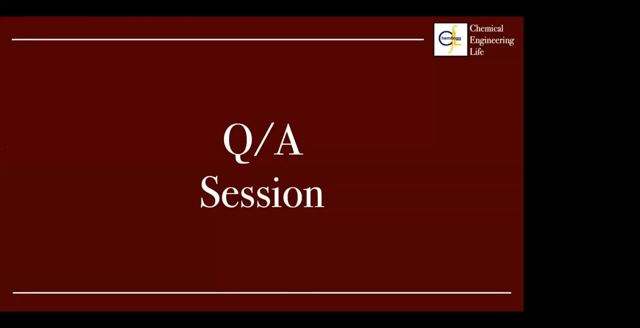 how does um this inability this variability in supply exactly how do you, how do you understand badly affect this economic analysis? 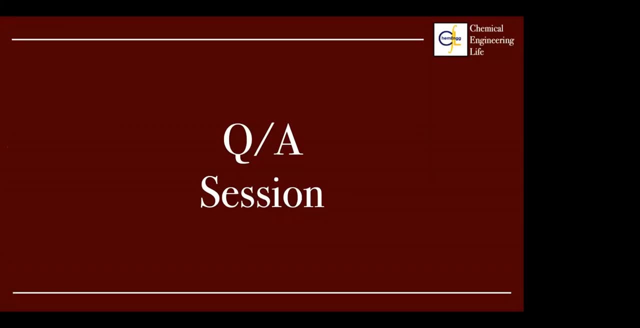 I don't know if there's a huge impact of this non-established supply chain in the economic viability of a project. Yep, that is actually a very good question. 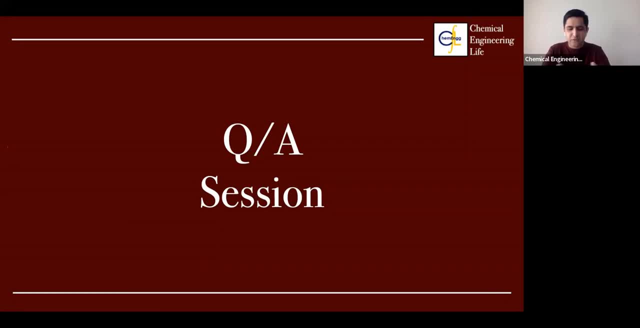 That is an excellent question. And the problem with waste cooking oil is that it is not a commercial product, right? So we don't have companies that are like gathering waste cooking oil in tanks, and then you can just give them a call and have them brought that to us, right? If you read the research paper that I wrote, the price is $0.2 per kilo. That is actually the price that was calculated based on the transportation cost. 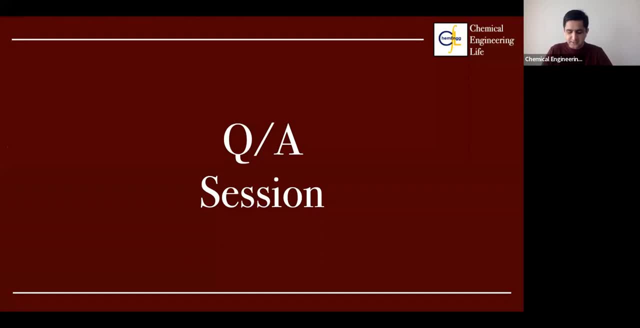 So what I did was that when I was doing the calculations, is that I recalculated that on typically how much does it cost to transport this oil from one place to another. And then I believe it takes a reasonable transportation, what do you call it, the distance. And then based on that, then we calculated the waste cooking oil price 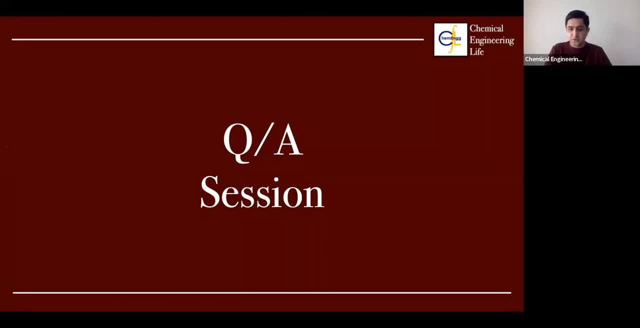 that we would be paying for it to be brought to us in terms of supply chain and from the supplier. 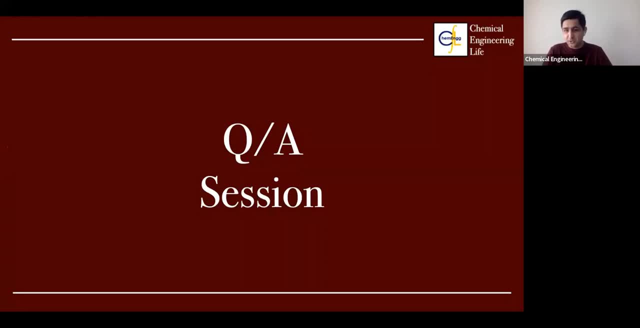 And that is actually one of the reasons why it was so cheap to use it using a source that I picked. 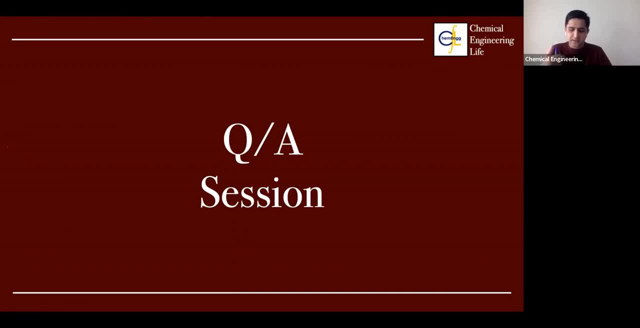 If you dig deeper into the supply chain, and if you have, and if you have people that are gathering waste cooking oil in one place, they have these, let's say, huge tanks, 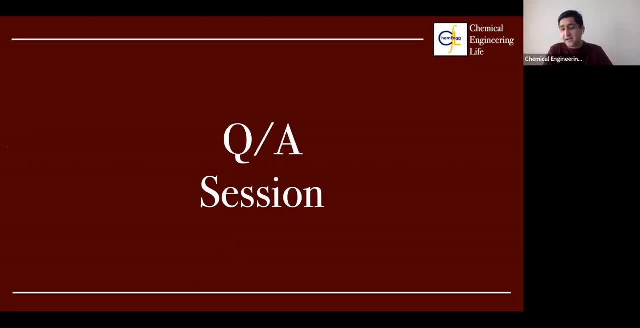 and then they give you the waste cooking oil, automatically it's gonna be more expensive. 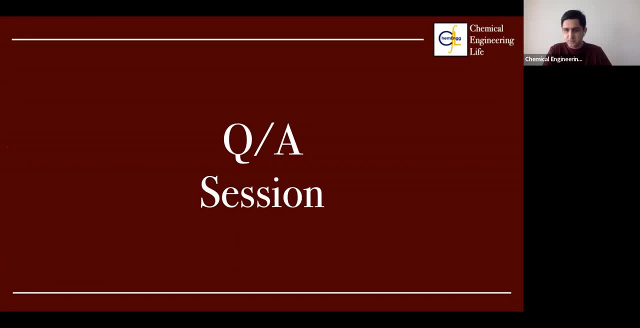 That is the limitation with it. And then you said it very correctly that the supply chain of waste cooking oil is difficult because it's not very easy to assemble. 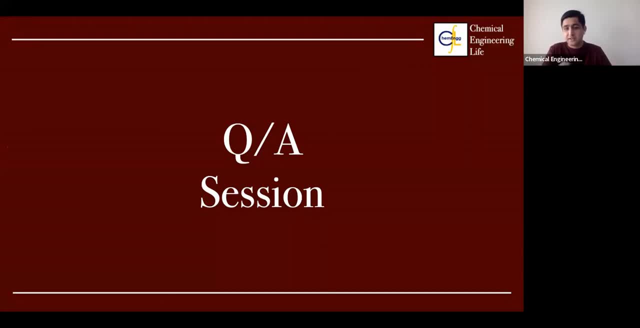 You could go to different restaurants and you can ask them to give them to you, 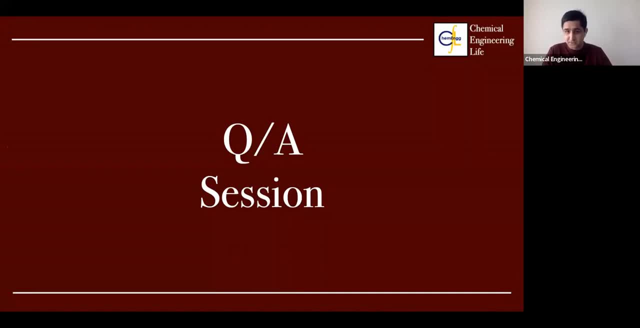 but it is very difficult. And that is a huge limitation in the biodiesel production, because it's one thing saying that you can use biodiesel and you can have it transported to you to produce biodiesel, but having to gather that amount of waste cooking oil is a challenge in itself. 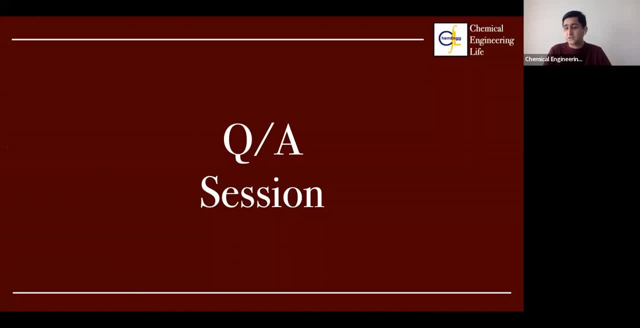 And I believe that is one of the main reasons why waste cooking oil has not really been used yet commercially to produce biodiesel. 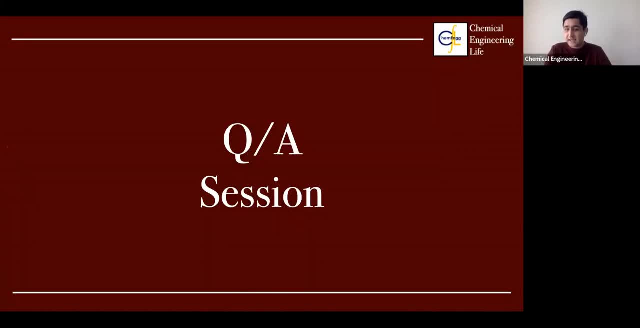 And just like you mentioned earlier that there are different companies now that are moving towards it, but in reality, in a general scale of things, the reason waste cooking oil has not really been commercialized or not used, 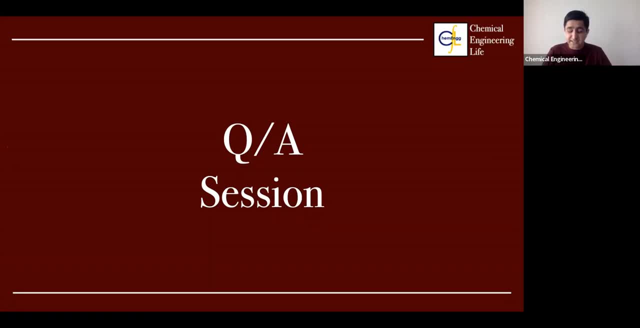 I believe in 2019, around the globe, only 17% of the global production of biodiesel is by waste cooking oil. Even less than that, that 17% was still an exaggeration. And the main limitation of using biodiesel is that it's not a commercial product. 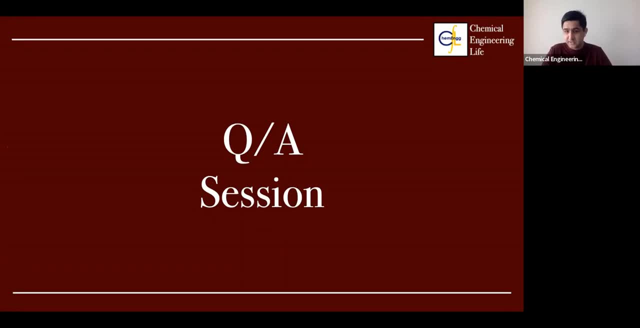 Using waste cooking oil is actually the supply chain. And that strongly affects the economic analysis, because if you say that you want to produce biodiesel 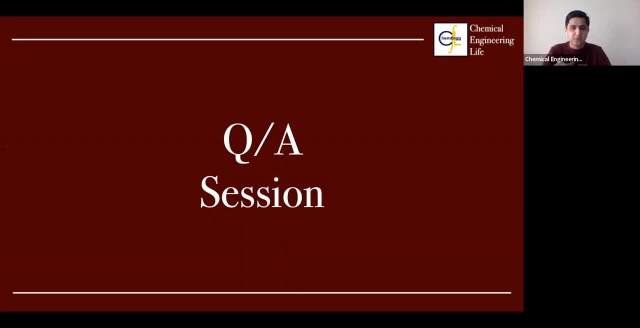 and you are going to go out there and gather waste cooking oil from all these restaurants that are in your area, that is one thing. But let's say you're living in, I don't know, in New York, and you want waste cooking oil brought to you from Texas, then you need to take into account that the transportation cost and all that stuff, that's going to increase the price of waste cooking oil. 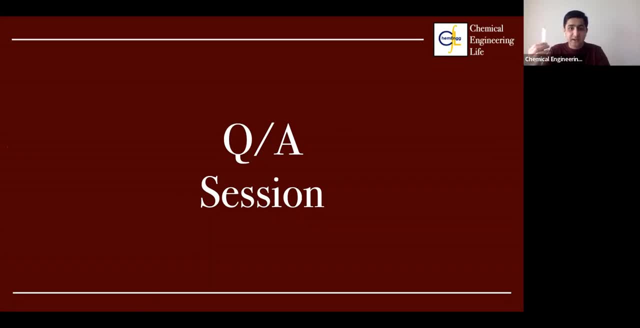 Likewise, if you reach out to a company that are gathering waste cooking oil and they are selling that to you, then it's even going to be more expensive. 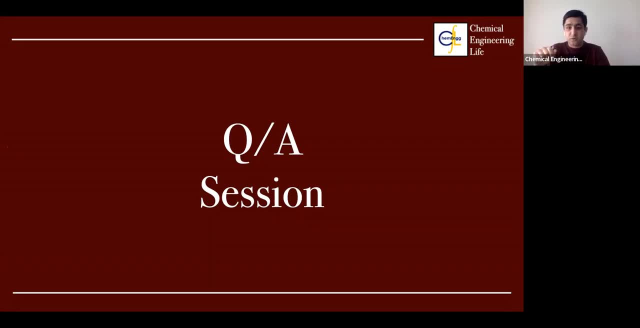 And so you're very right. So therefore, that is a strong question mark on the technical economic analysis 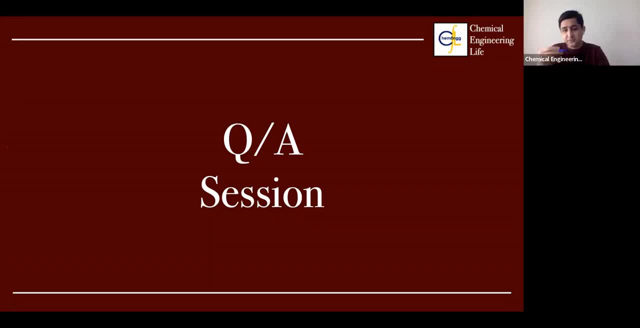 about how you're going to gather waste cooking oil. And if you do it through how you do it with the other ways, then it's going to be more expensive. If you do it yourself in terms of transport, transporting it or gathering it from different areas, then it's still going to remain slightly cheaper than if you were buying it from a middle person. 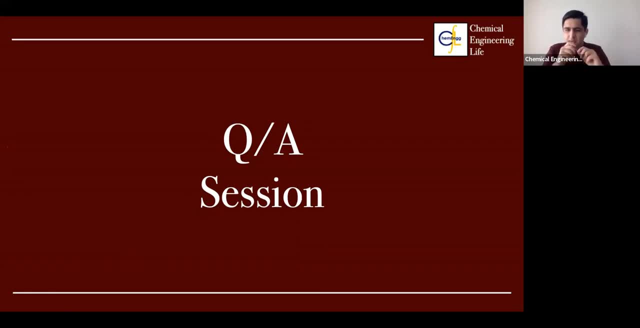 I hope that answers your question, if I didn't go away from what you asked. 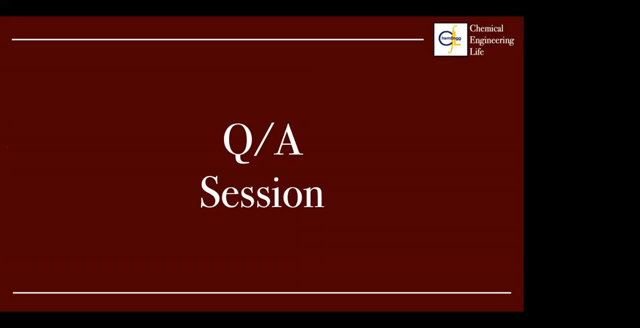 You did answer it quite well. But then I was probably thinking in my head, 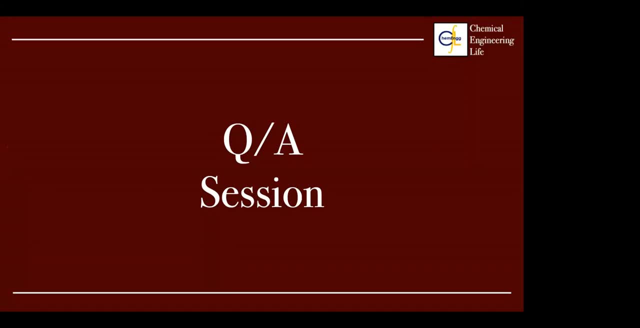 because I'm quite too devoted to sustainability. 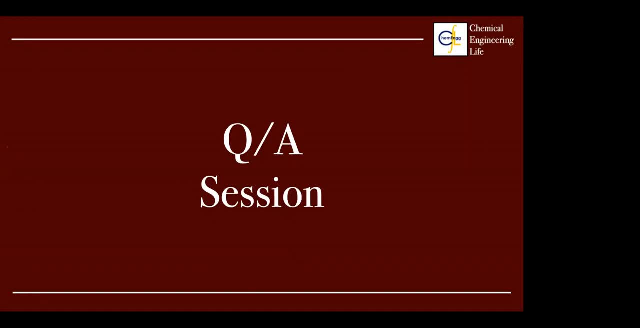 If we kind of approach it from the triple bottom line of sustainability, talking about before we look at the economic aspect. 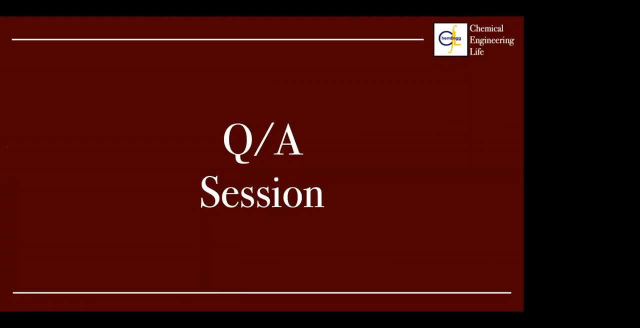 Maybe we could focus on the social aspect. Because when Andrew spoke the last time, he said there were some companies who had this social relationship with restaurants and sources where they get this stuff. It could really help a lot in gathering this raw material. Because for now, it's looking like a waste. But when it becomes a big deal, everybody will begin to hoard it. And the price increases. And when the price increases, it affects the overall sustainability of our project. Right. 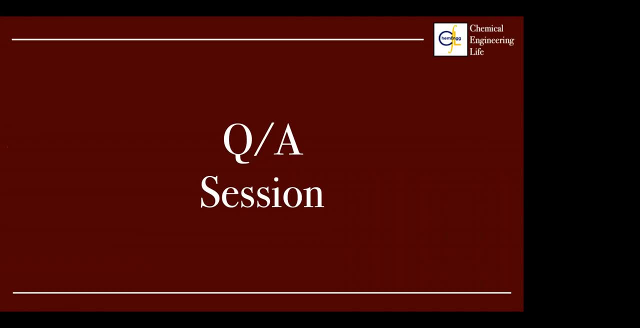 So I think the major aspect to look at is the social aspect. Because a larger quantity of this oil comes from restaurants and homes. 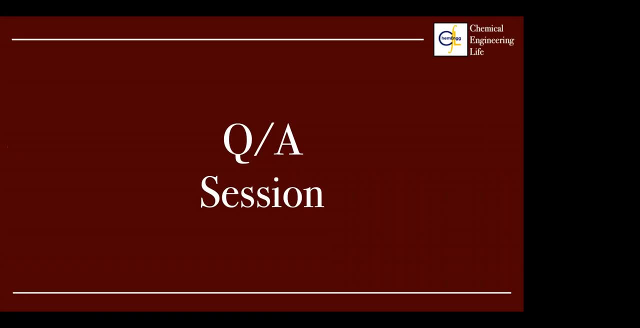 And if there's no established relationship between the suppliers and we or the builders of a biorefinery who needs this waste cooking oil, I'm not sure there will be this constant supply. 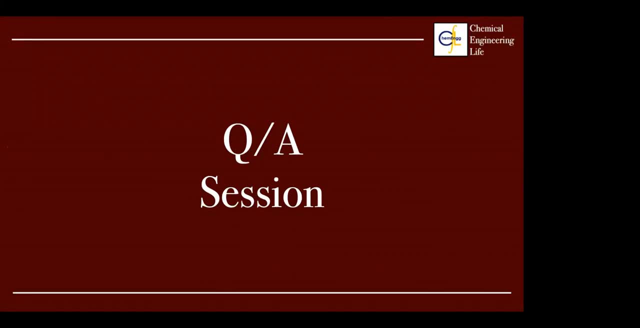 And that way, our analysis will always be false. Exactly. And that is very true. 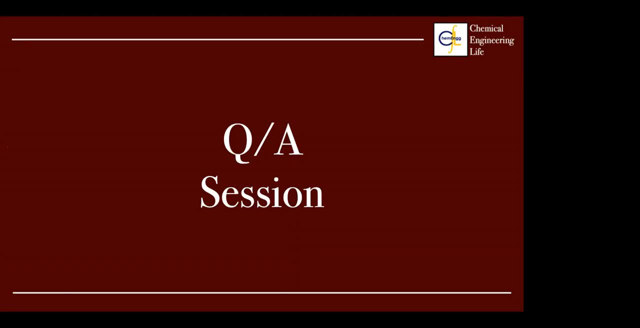 Because just like how earlier it was mentioned, back in the old days, when soybean oil became the talk of town, it actually used to be very cheap as well. But then once people started to realize that it can be used for so many things, the price simply skyrocketed. 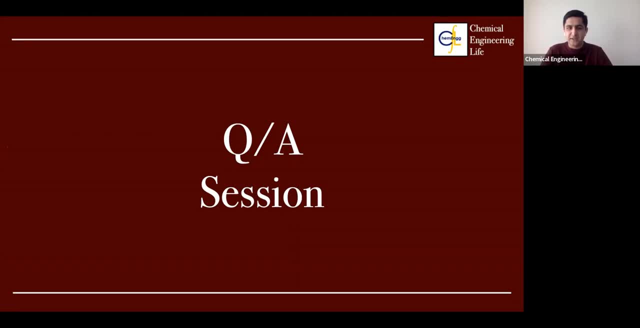 And that is one of the reasons why we do this sensitivity analysis. And like I showed you earlier, in this case, we only vent up until 100%. 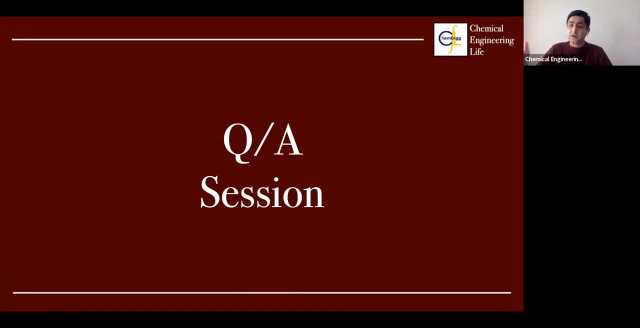 But in reality, it could go a lot, a lot higher than that. Because just like you correctly mentioned, yourself, once people start to realize that the waste cooking oil can be used to produce biodiesel, which itself is a very expensive product, and you can create an ROI of 300% per year, people are automatically start going to hoarding it. 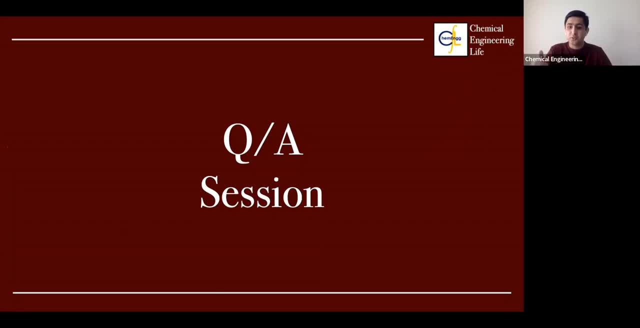 And restaurants and houses, they are going to start selling it to us at an additional price, 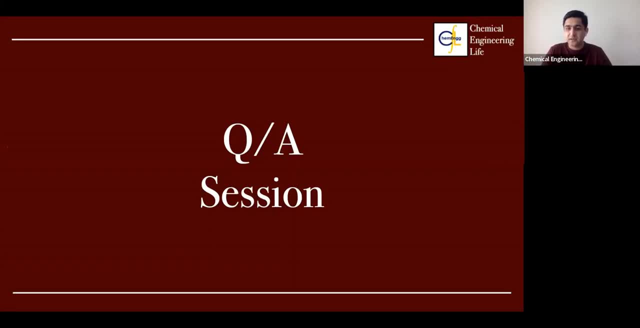 even though nowadays people are simply just throwing it out. But in the coming time, they will start hoarding it and start selling it at a much higher price, which will limit the profitability of biodiesel production. 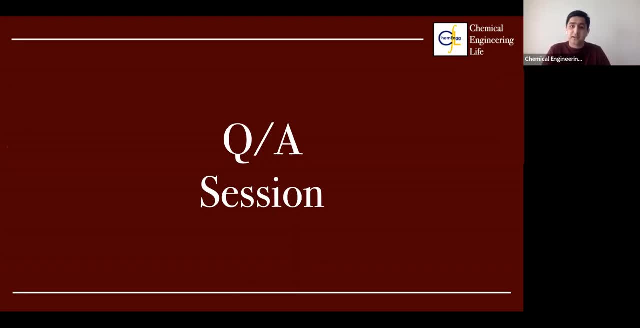 And that essentially is the bottleneck right now when it comes to bioprocesses compared to petroleum fuels. Because the reason petroleum fuel is so lucrative, so expensive, much more, one could say, profitable, is because they don't have these loopholes that biodiesel, currently, have, especially when you're using oils. 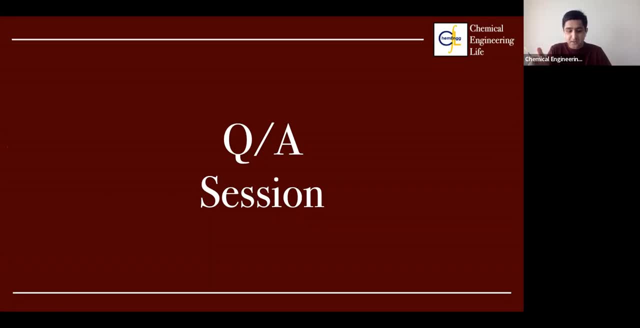 Because right now, to be honest, when you think of soybean oil itself, it's not that much of an economical problem, but it also tends to be an ethical problem. Like, does it make sense that we start using soybean oil instead of for feeding different people, we start using it for biodiesel? That's also a question mark. That's also a problem why you can't use it for production. 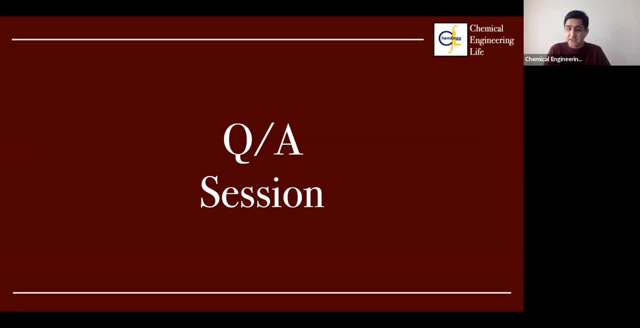 And although it's expensive, the waste cooking oil, even though it's a waste, it will get more expensive. I have found sources where some companies in England, I believe, even in the US right now, they are selling waste cooking oil at prices as high as $0.6 per kilo. So it is slowly being commercialized. And the higher the price it goes, the less the profit profitable the biodiesel production will be. 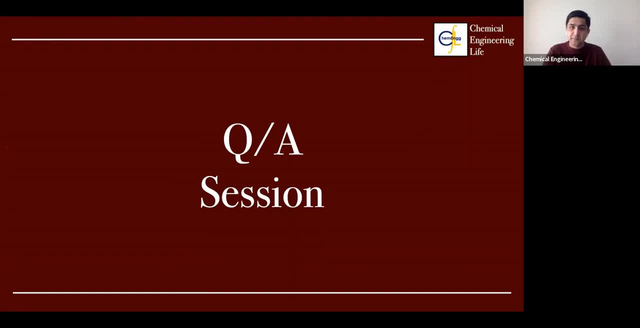 And it is, sadly, a limitation. But then, as an engineer, then your job is indeed to find ways that you can optimize the economics of the process. Because if the raw materials are going up, then you have to find different ways in which you will have to increase your profits from your production. And that is something that you have to look into something we call a process integration or something you can go down and you can, for example, right now, the research paper that I shared with you before, glycerol is a very low end product, for example. You can use glycerol to produce succinic acid. Glycerol, it sells at around $0.8 per kilo. And that $0.8 is actually very high because the market of glycerol has plummeted. So it even sells as low as $0.3 per kilo. 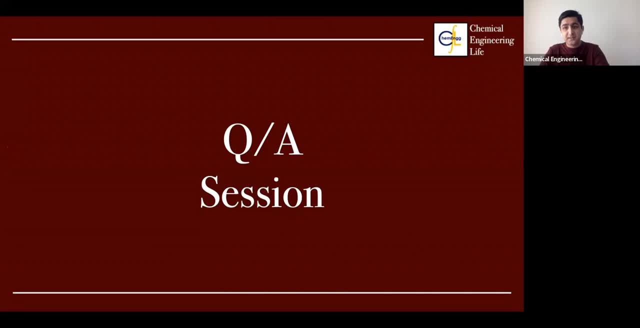 But if you use glycerol to produce succinic acid, then you have two processes. Then you're selling biodiesel and you're selling succinic acid. And succinic acid sells at around $1.2 per kilo. 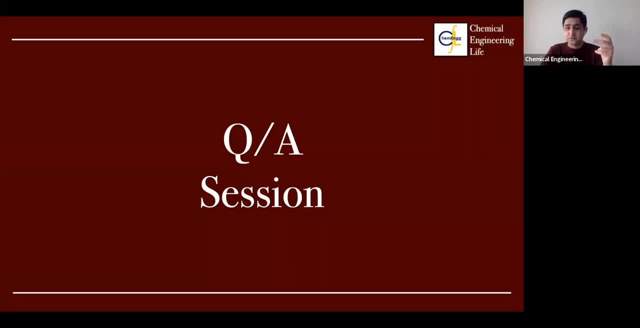 So in that way, you can increase the profitability of your process to make it more competitive to petroleum fuel. I hope that answered your question as well. Yeah, very well. Thank you very much. Thank you. 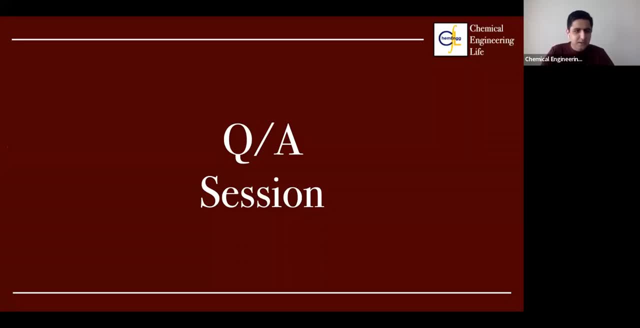 Then I can see someone asked a question, Mansab. It is because in the paper that I shared, the paper, it is an example of process integration. 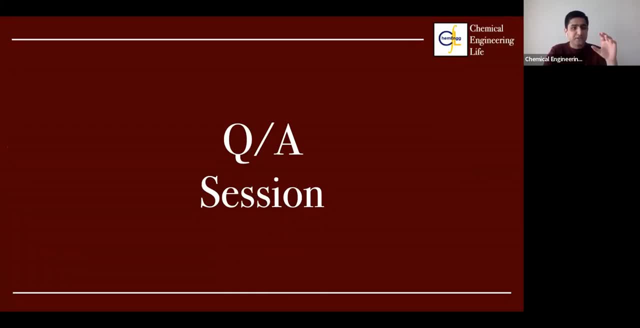 So there are three different processes within that paper. So you actually have the thing that I just mentioned right now. 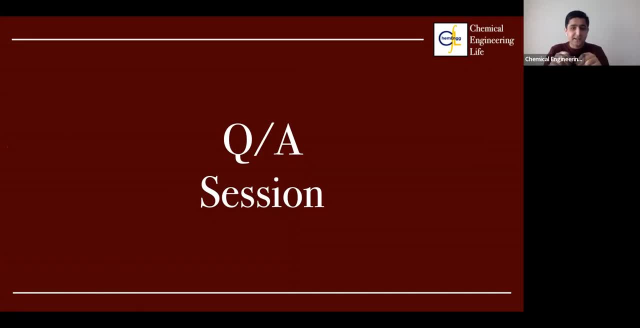 So we have biodiesel. But because biodiesel cannot be as profitable compared to petroleum fuel, just like we talked about that wage cooking oil will go up in the coming days. So therefore, the approach that we took 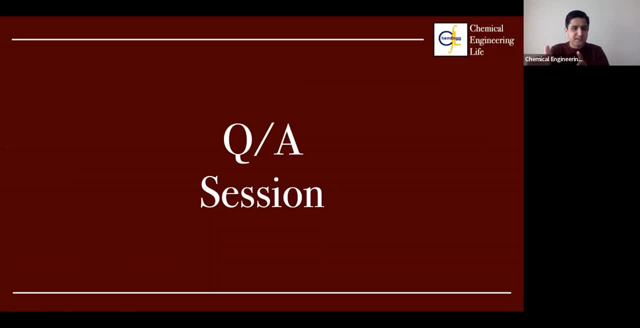 was that we integrated biodiesel with succinic acid, what do you call it, succinic acid production. 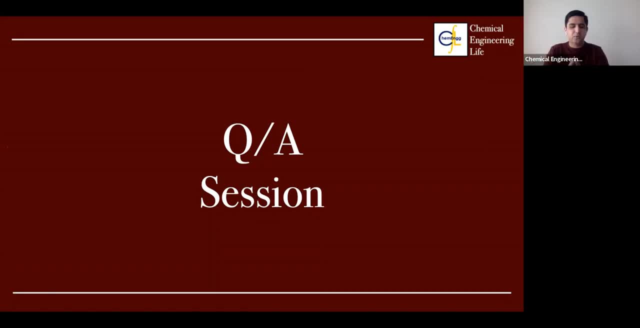 By doing so, we increased the portfolio in a way. In the same time, the methanol that we 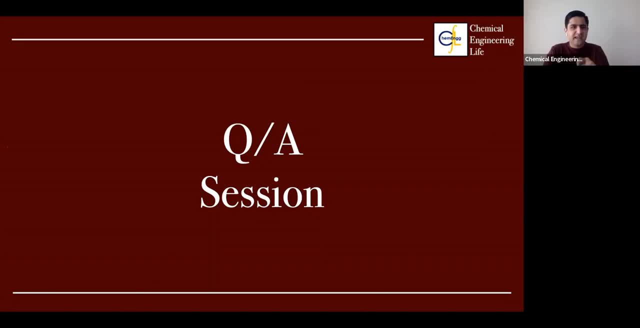 are using is the raw material. Instead of buying methanol, we actually produced, methanol in-house using methane, CO2, and water. And that's what you're looking at as the raw material. 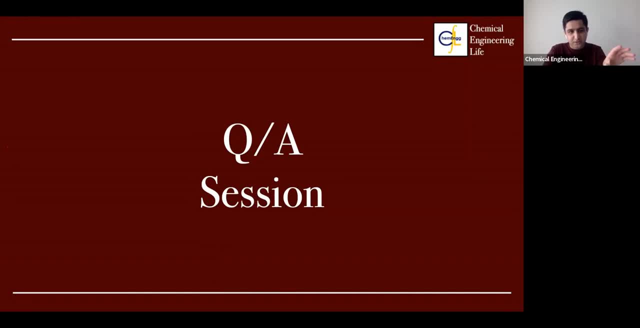 So in the paper, there are three different processes. The first process, that is the methanol production. The methanol from the first process was then used to produce biodiesel. 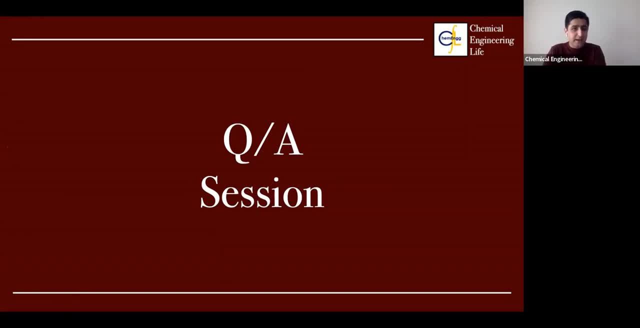 And then biodiesel, then we got biodiesel. And for biodiesel, you're only using wage cooking oil and methanol. 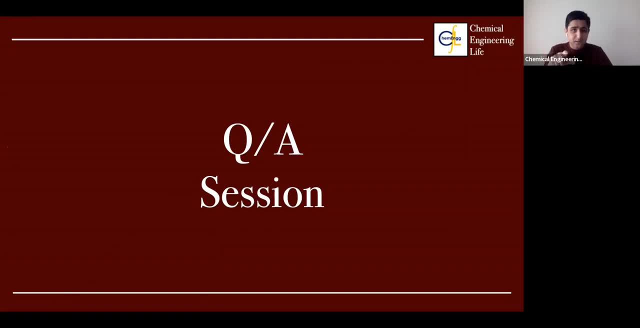 And then the byproduct stream from biodiesel was then used to produce. Succinic acid. I hope that answered your question. 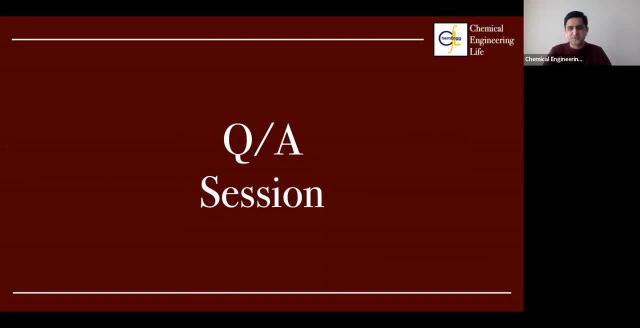 And I'm sorry, I didn't make it clear in the information that was sent out. 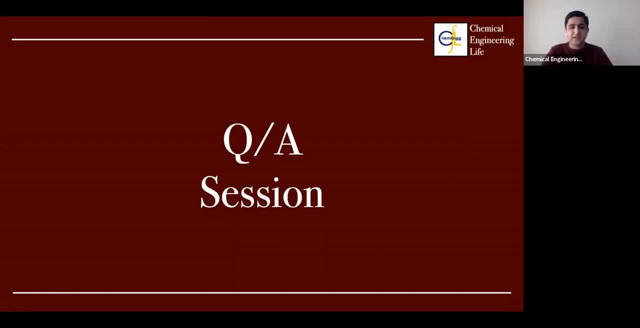 But for this webinar, we decided only to look at the biodiesel production and not the other two processes that were discussed in the paper that was shared with you all. 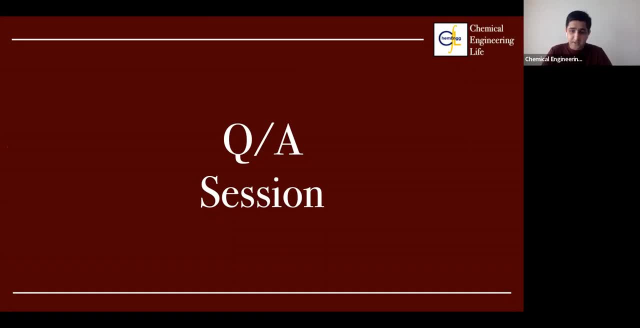 And yes, of course, I'll share my email with you. So if you guys have any questions, you all can feel free to reach out any time to ask about the techno-economic analysis. 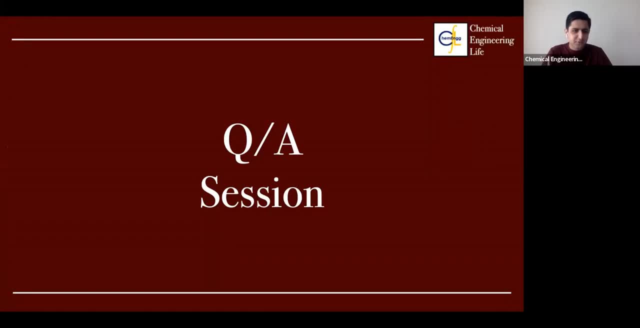 And regarding the simulation, I'm afraid I cannot share the simulation with anyone because they are protected by some confidentiality agreement. 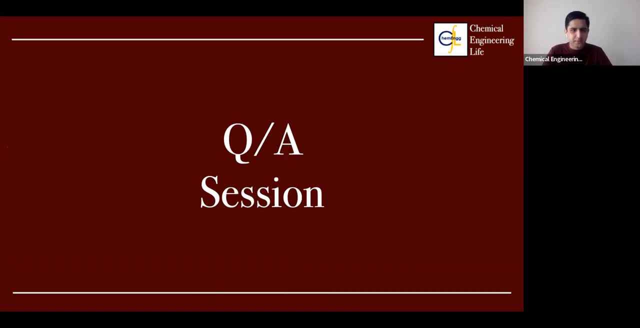 So I'm afraid I cannot share the process simulation file. But if you have any question, I'll be more than happy to help you and answer any question that you guys may have in terms of the simulation. Does anyone else have any other questions? 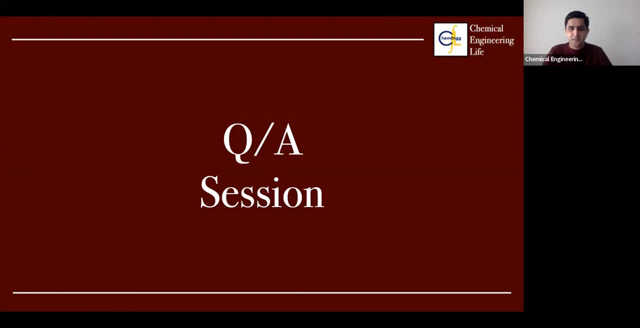 Great. Then I think we are also a bit over time now. So thank you to everyone that joined in today. And thank you for listening to me speak. 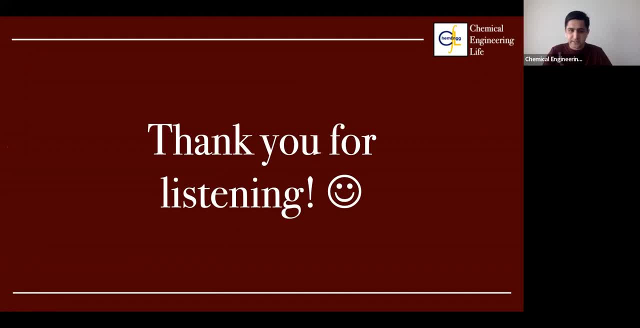 And like I said, I will share the literature that I have and also the different other textbooks that I have been using for techno-economic with you all. So you all can get a chance to also use them in your future projects, if you wish. And if you guys have any questions or about any of it, feel free to simply share my email with all of you. And you all can simply reach out any time you like. And I was told. 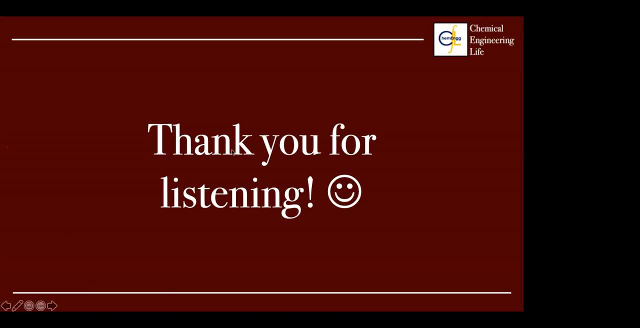 Thank you so much, Hamza. Thank you. Thank you. Thank you, everybody, for joining us today. 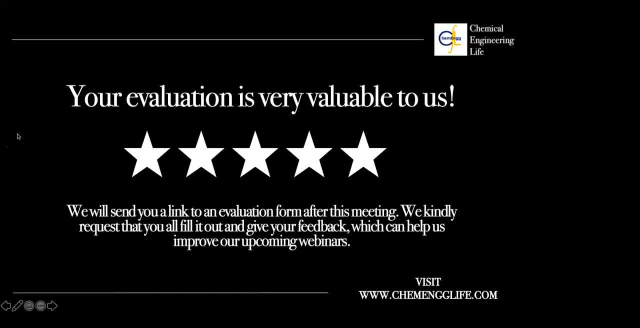 And thank you, Hamza, for making us smarter on the techno-economic topic. 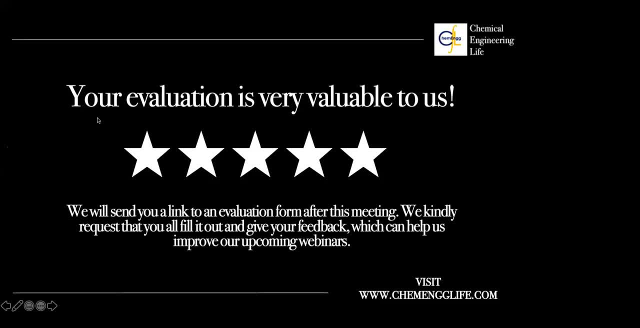 I definitely feel like I have a bit more knowledge here now. OK. And thank you, everyone, for being such a great audience. 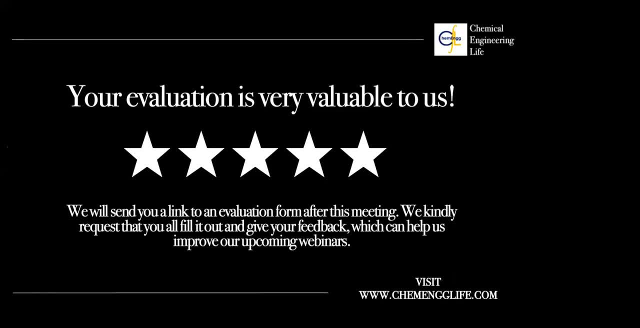 To be a part of such webinars in the future, make sure to become a member on our website. 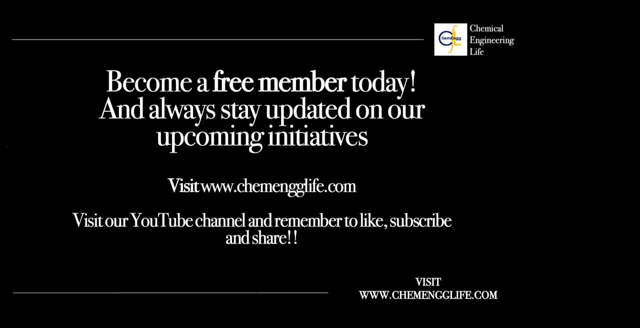 And this webinar will be uploaded on YouTube. So you can rewatch it any time if you feel the need to revisit the topic.